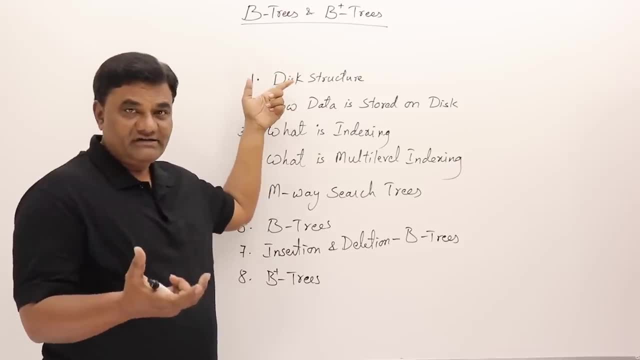 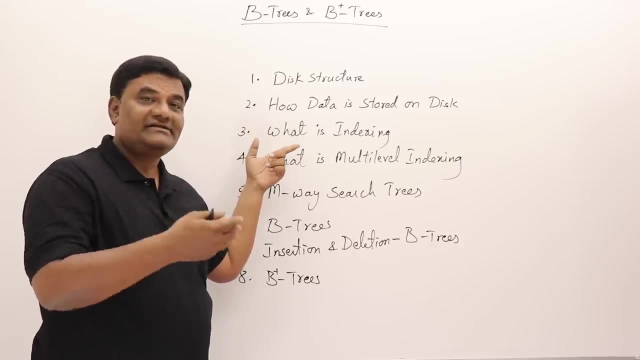 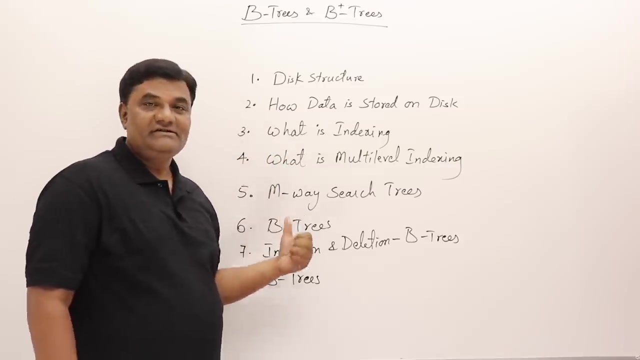 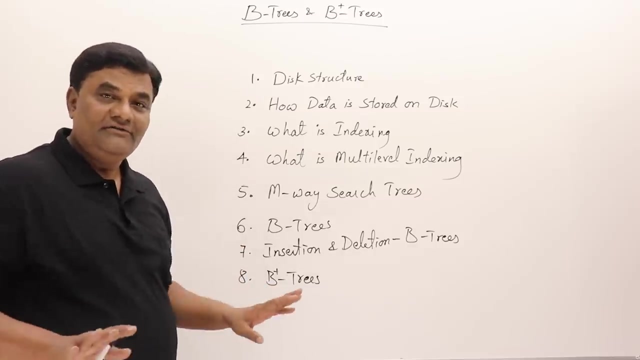 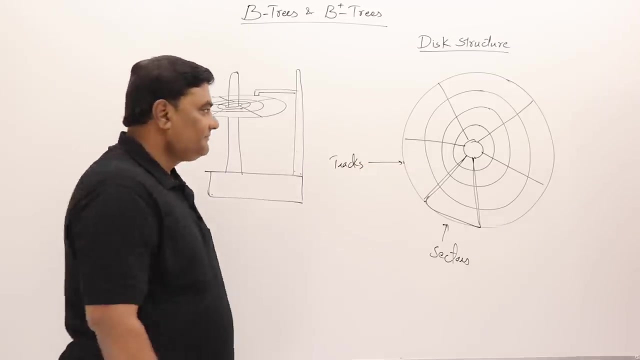 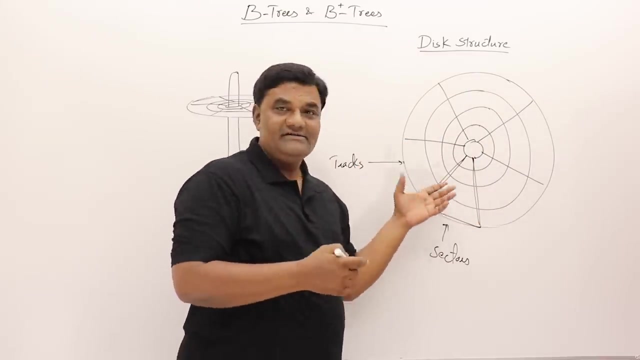 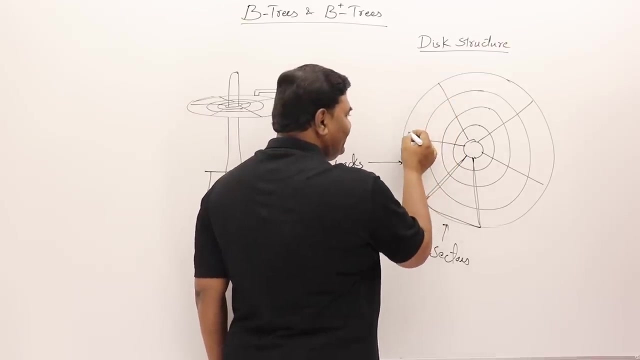 Let me read out the topics. If you know all these topics, then you can understand perfectly what B and B-plus trees and B-plus trees are. If you know all these topics, then you can understand perfectly what B and B-plus trees and B-plus trees are. 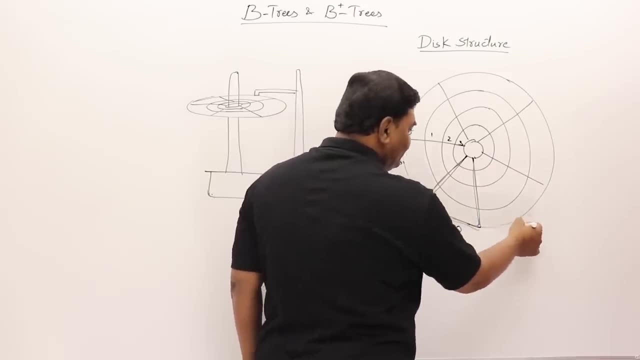 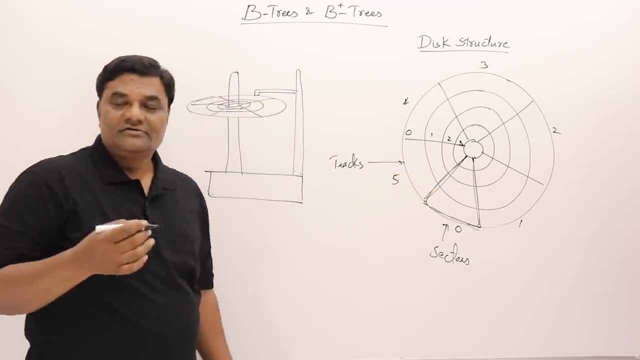 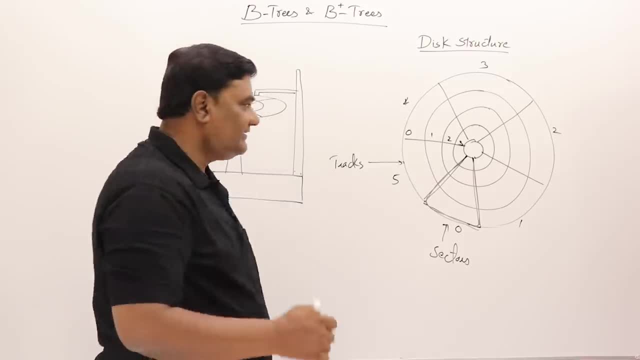 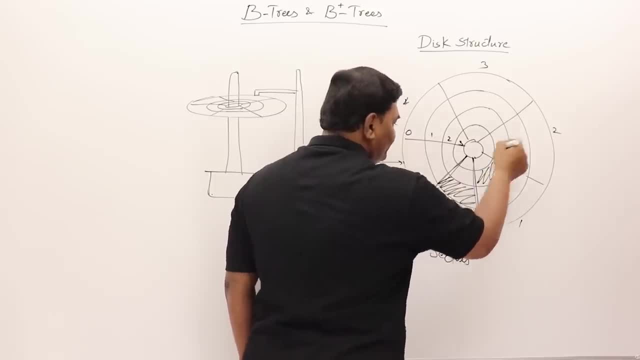 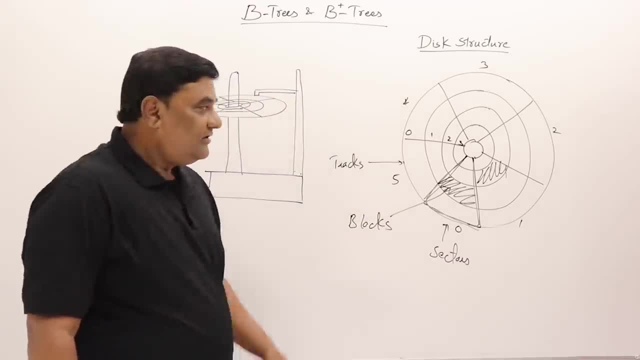 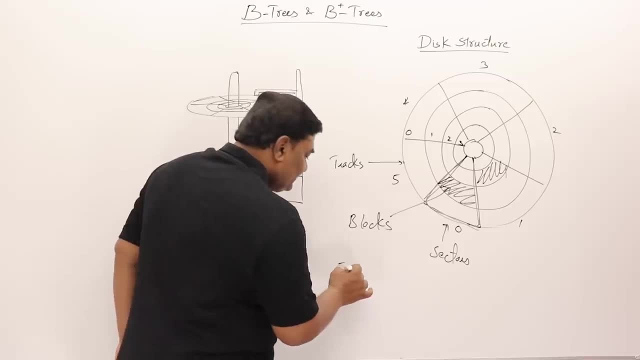 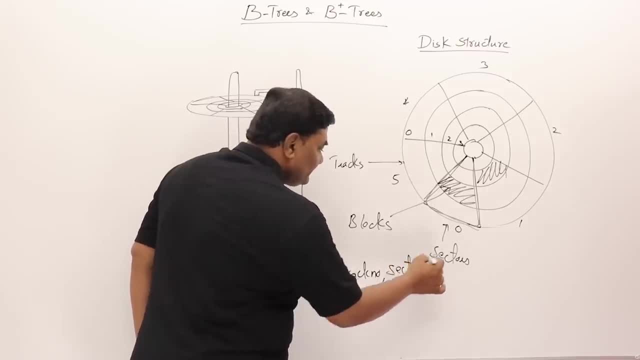 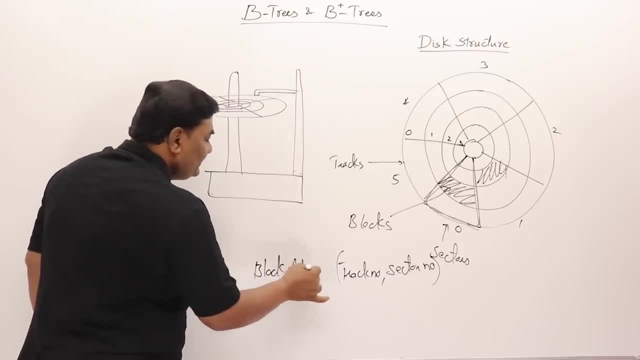 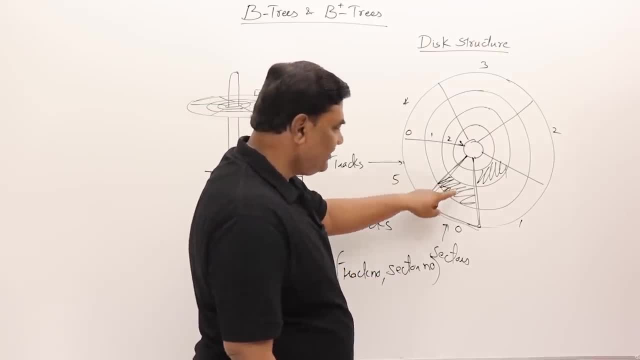 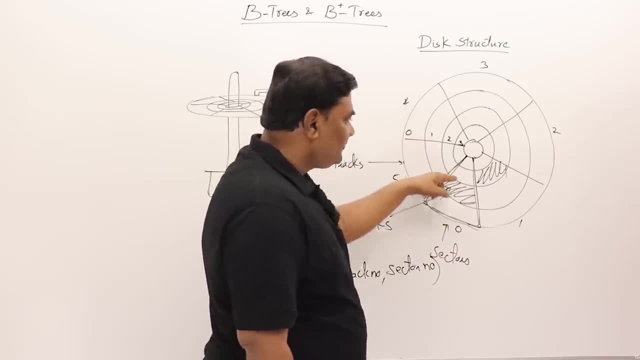 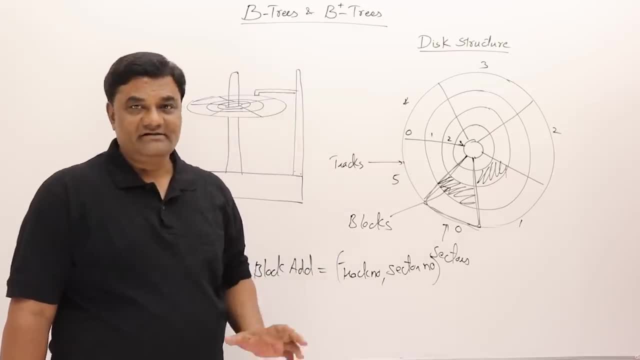 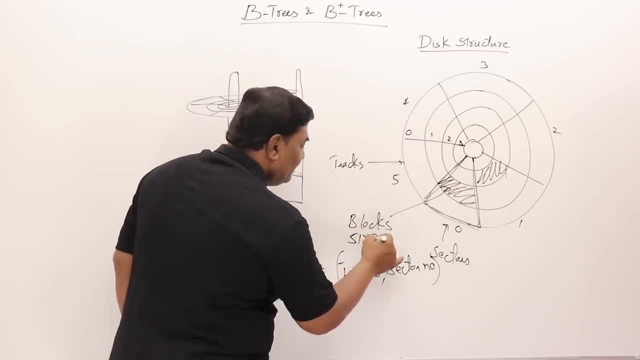 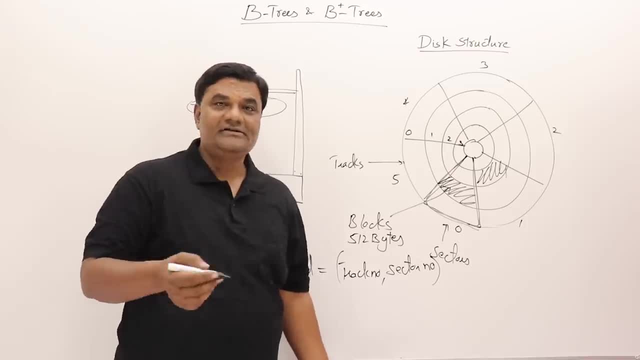 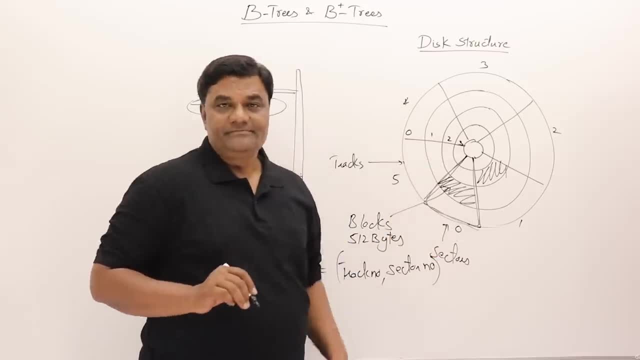 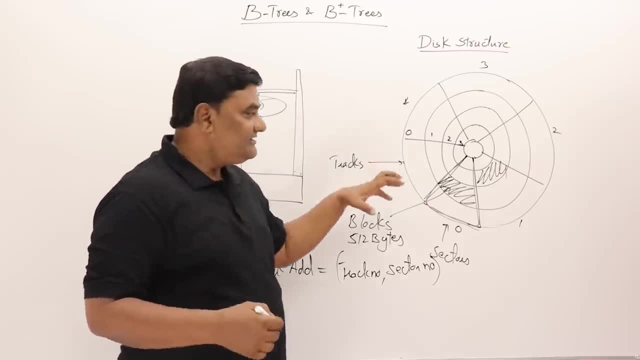 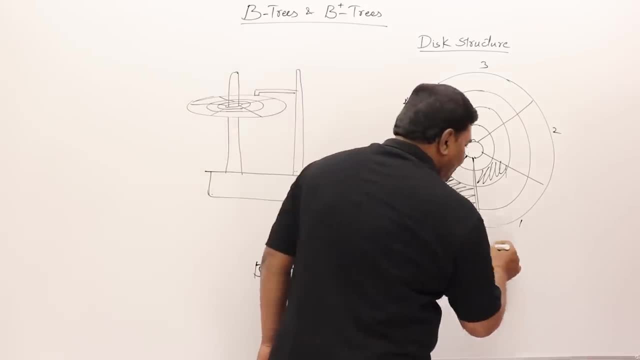 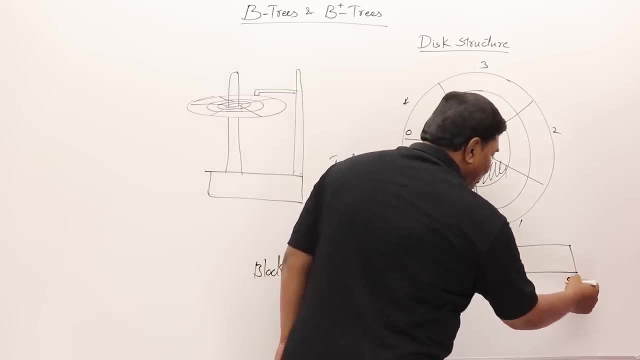 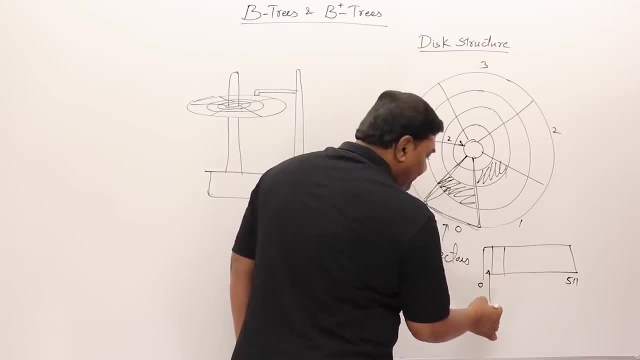 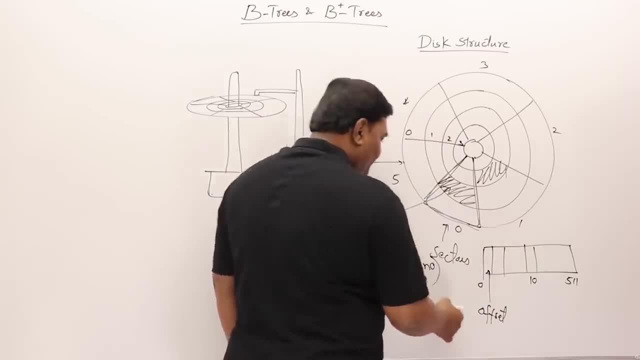 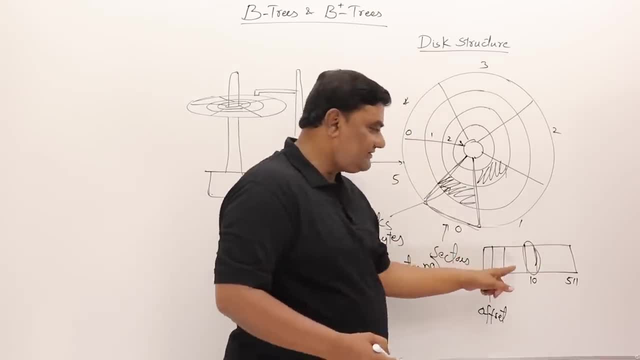 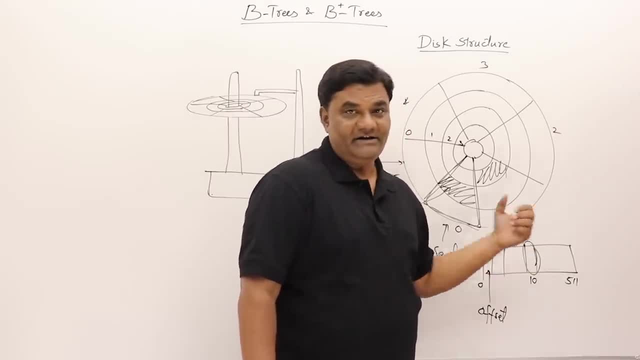 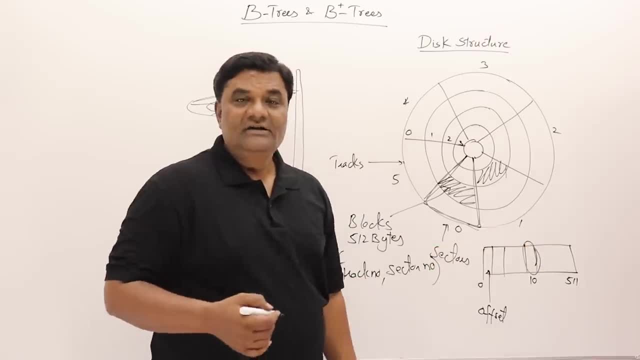 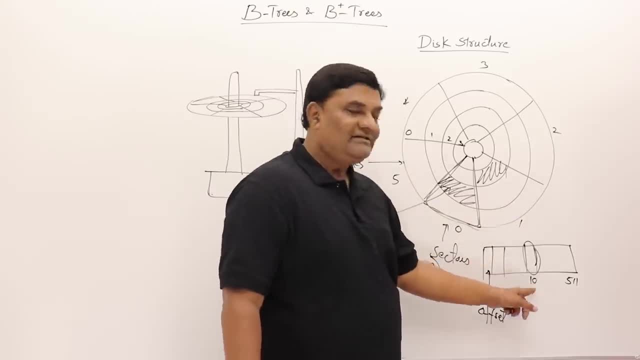 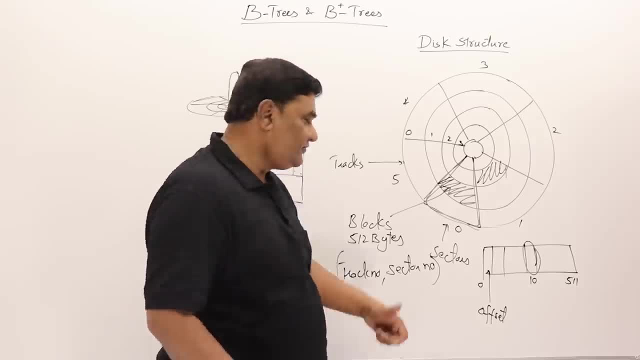 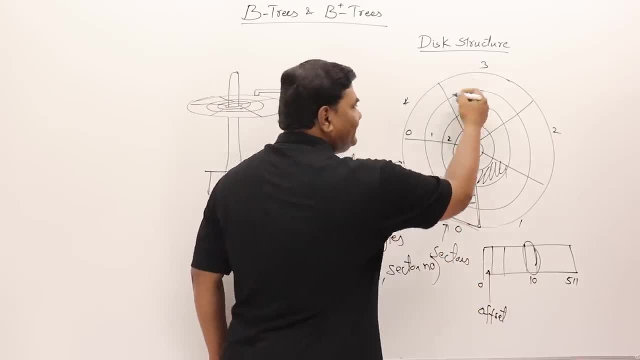 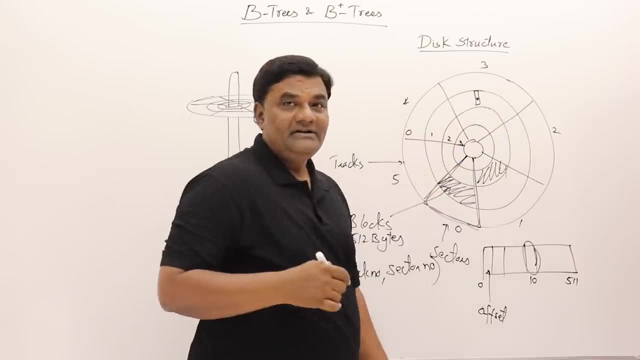 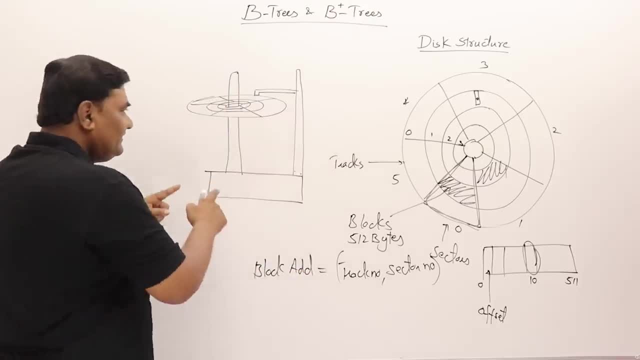 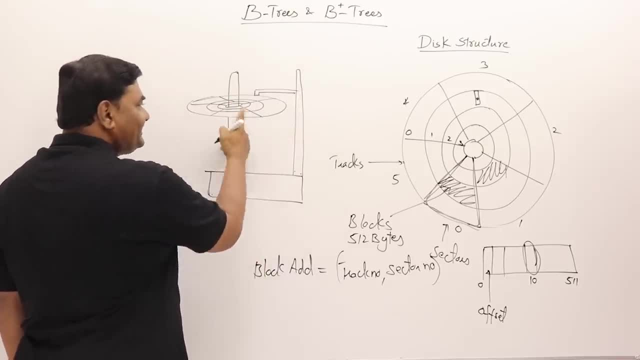 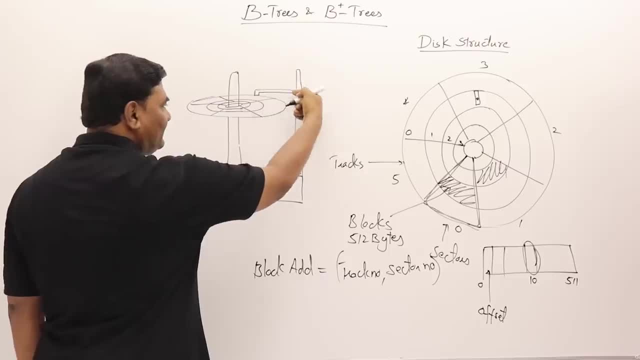 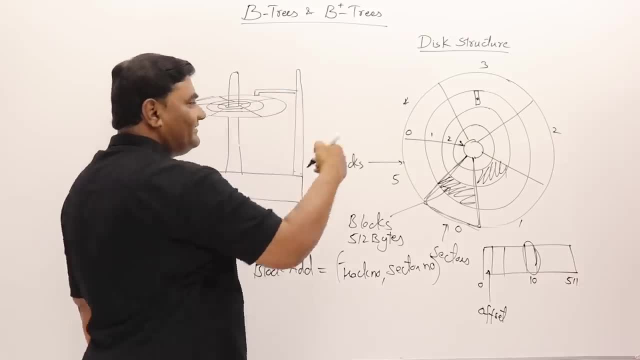 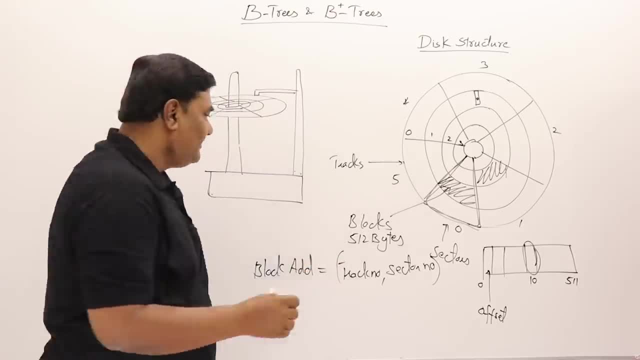 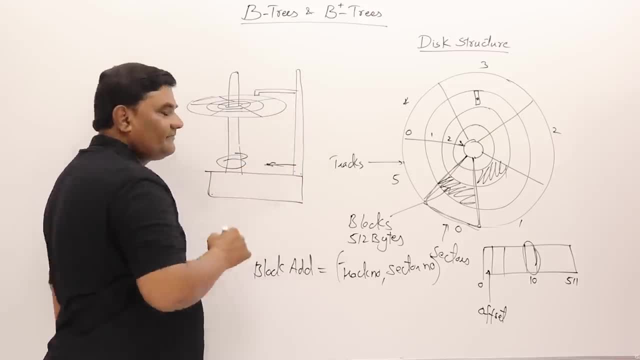 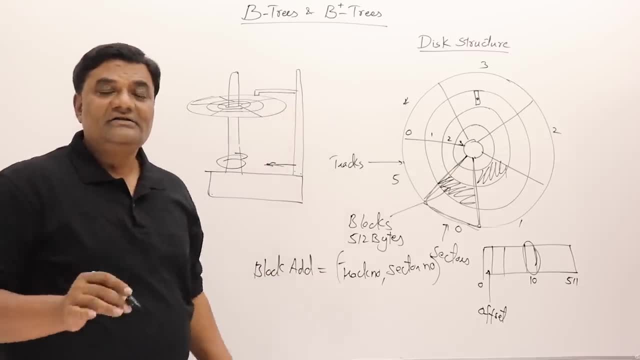 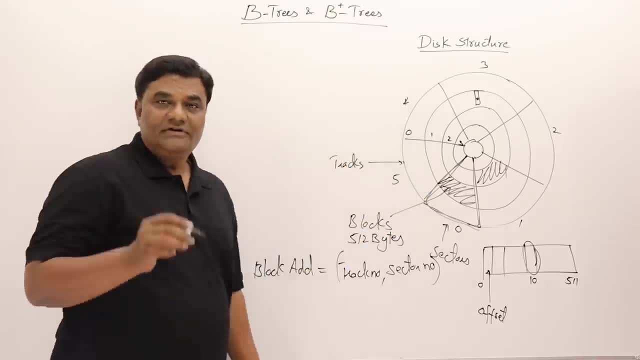 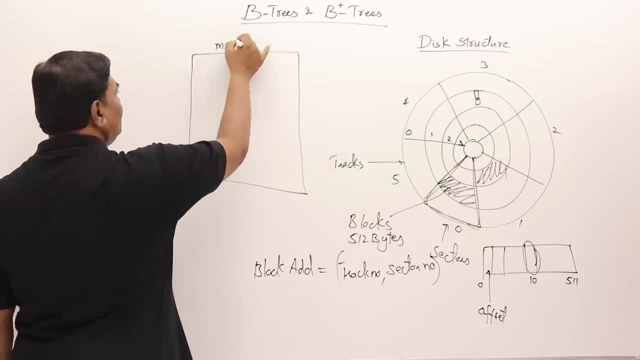 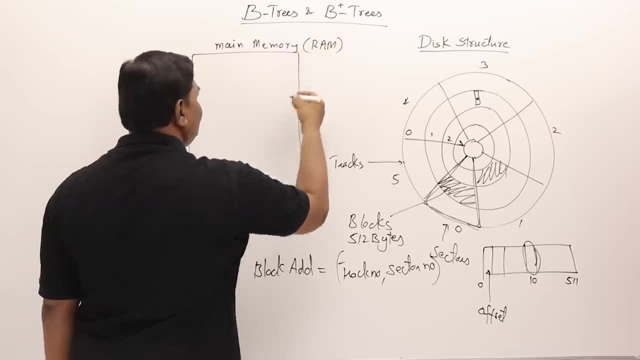 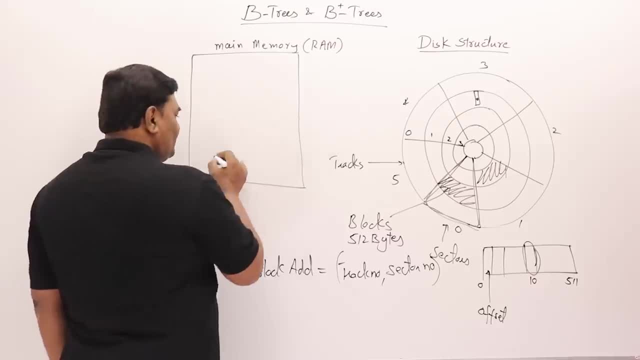 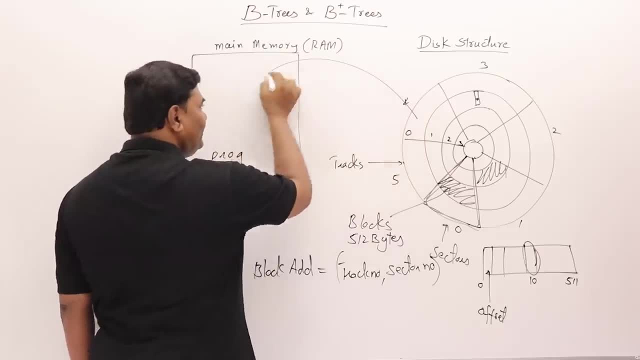 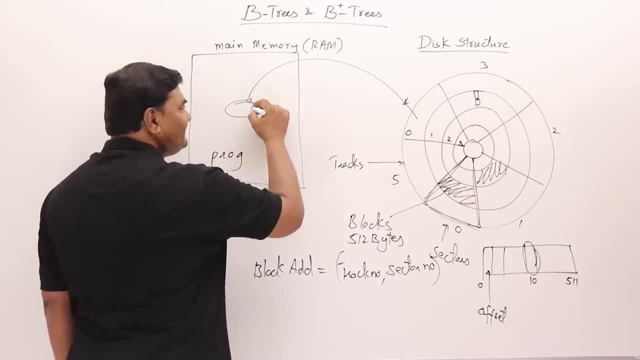 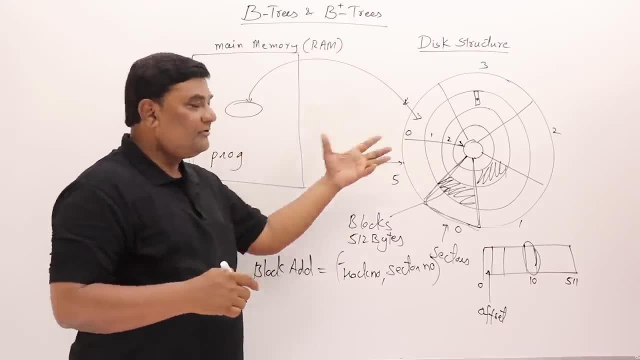 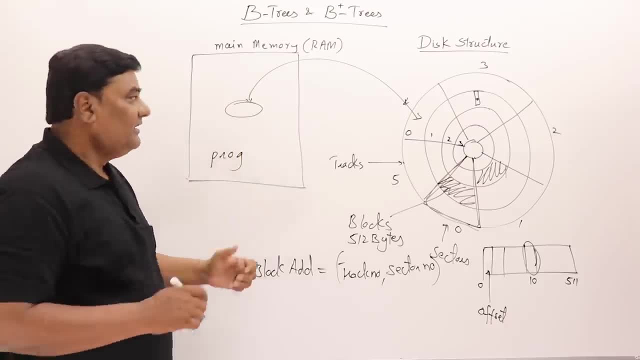 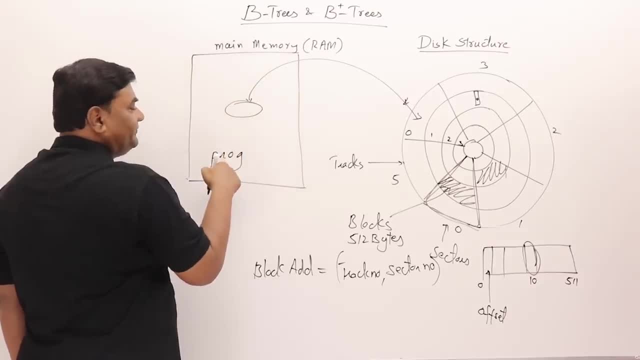 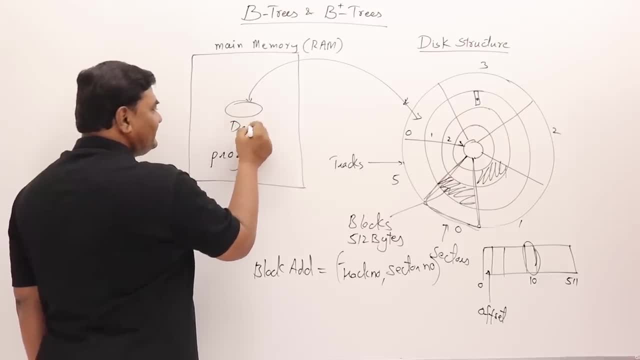 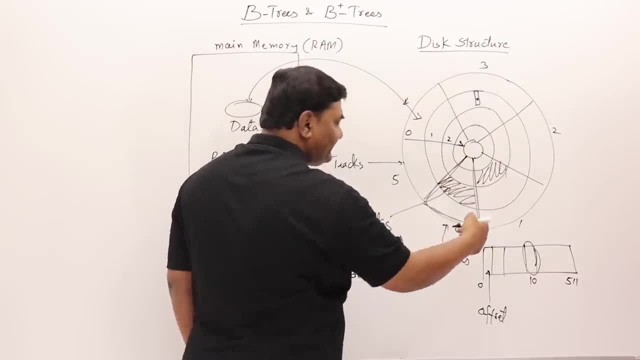 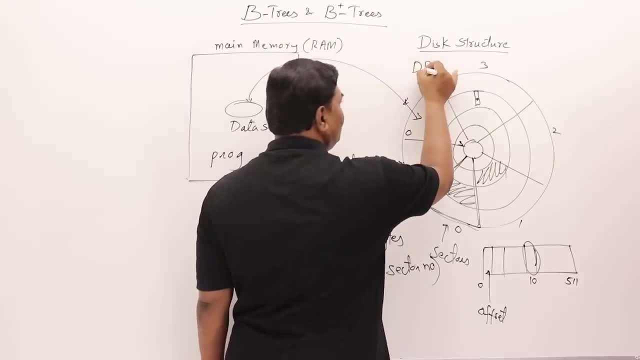 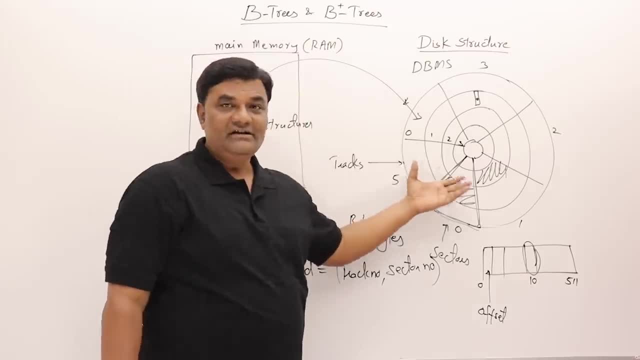 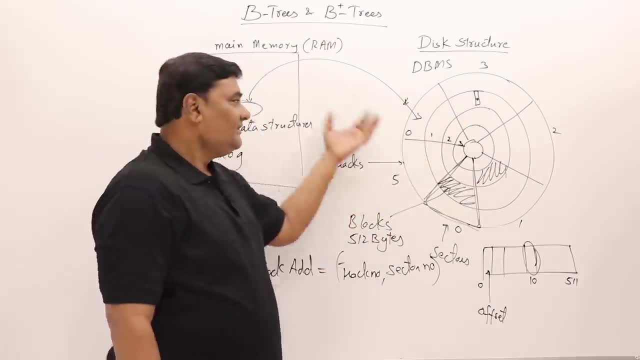 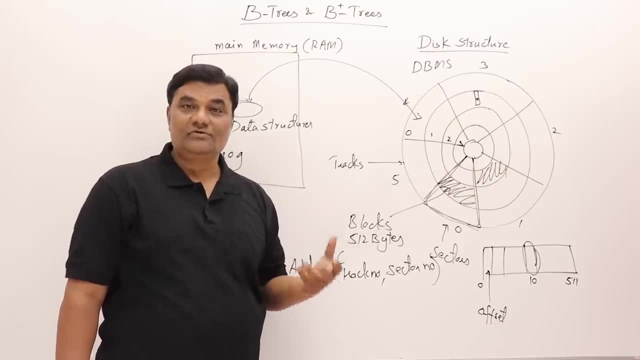 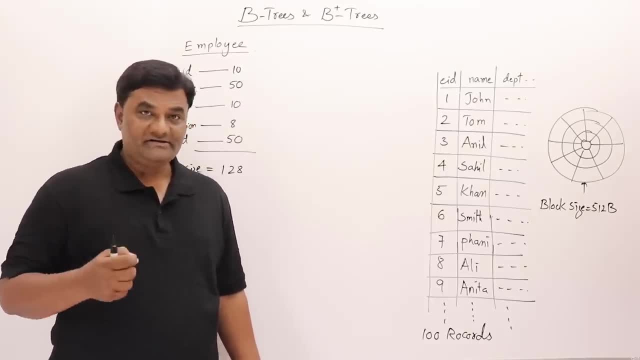 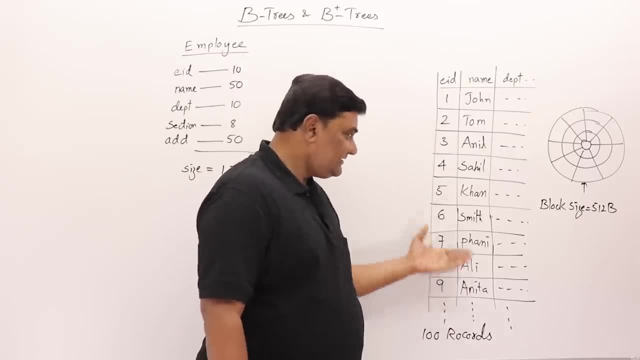 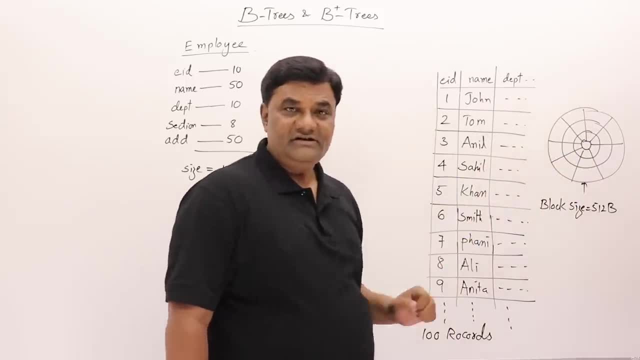 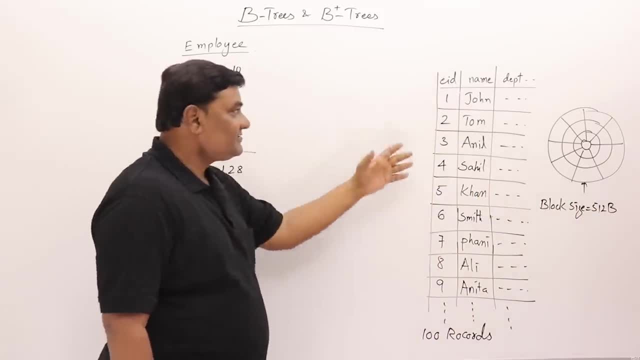 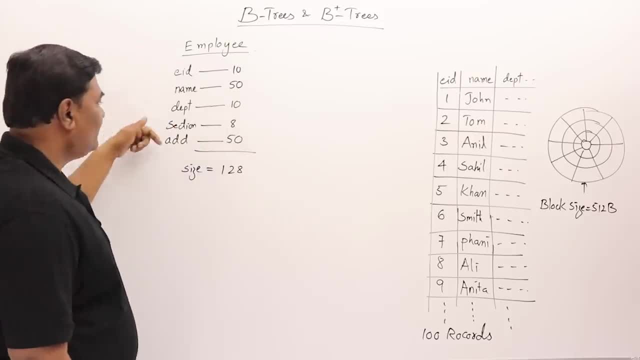 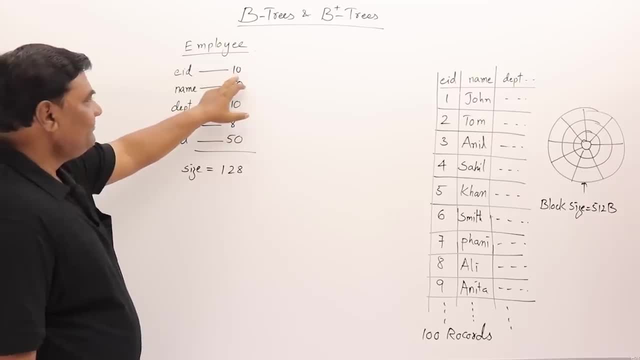 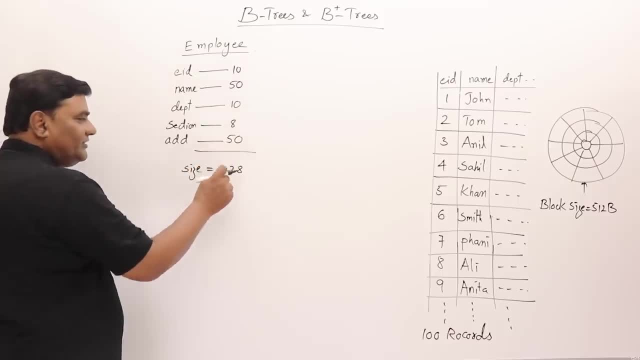 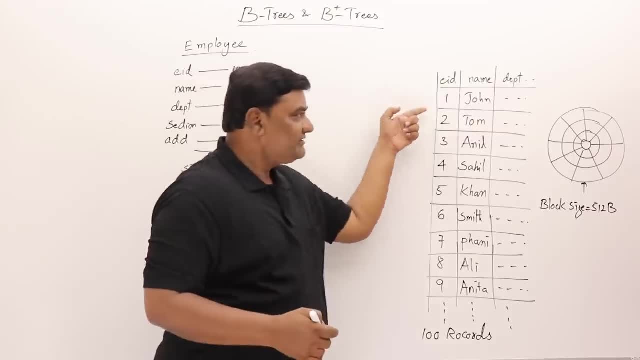 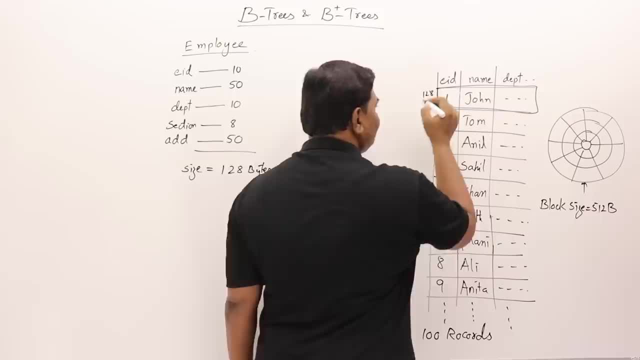 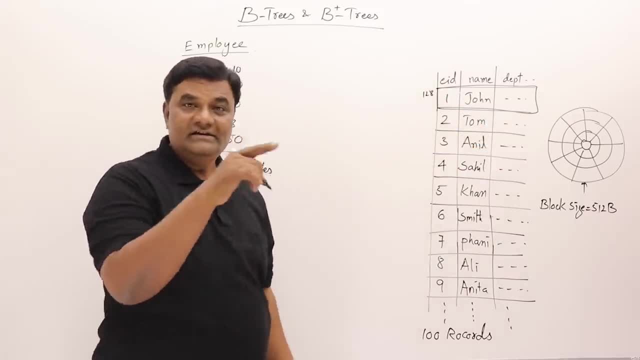 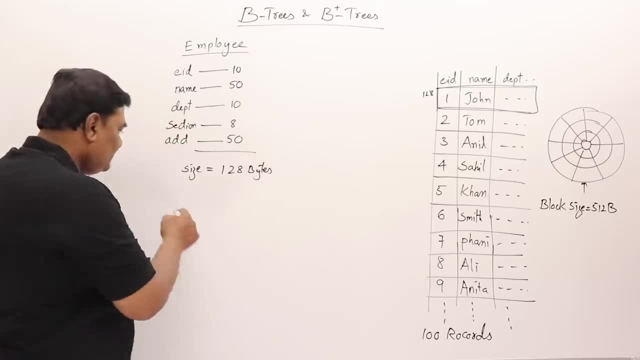 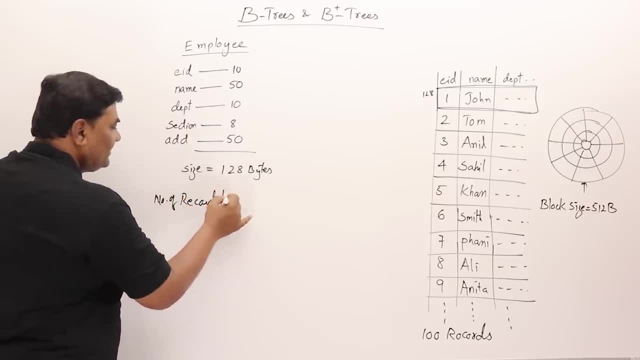 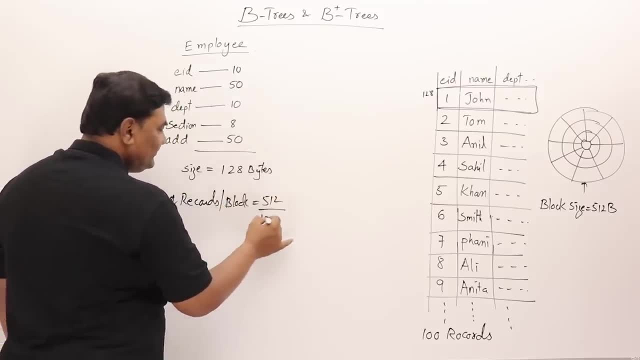 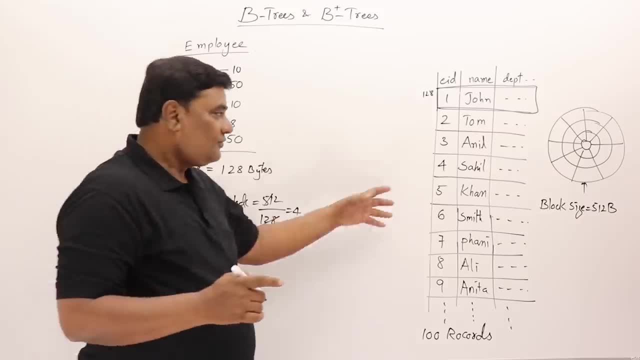 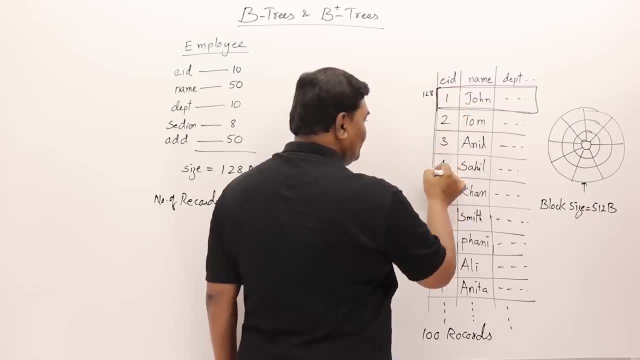 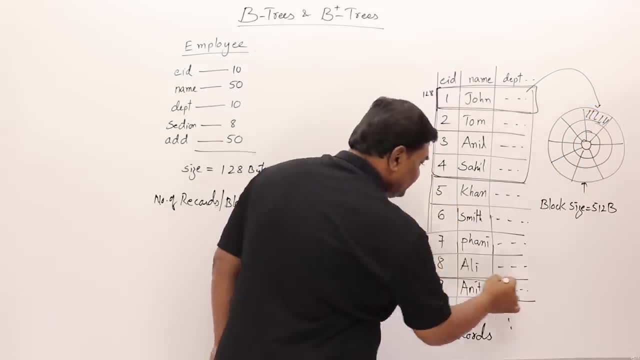 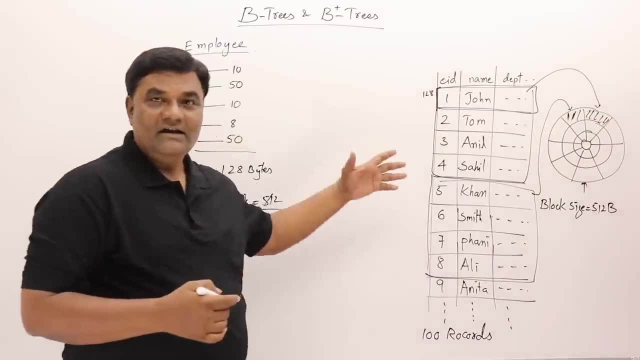 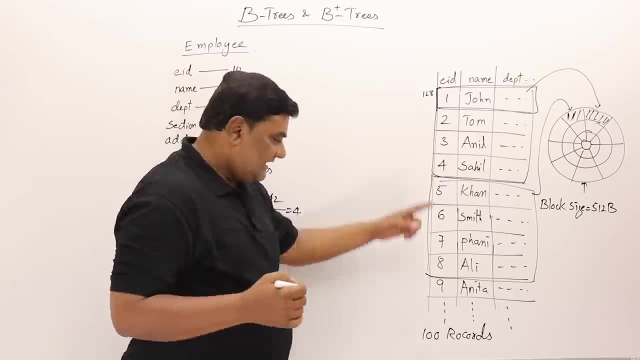 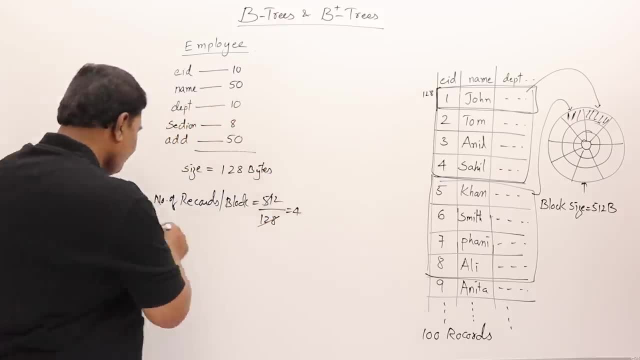 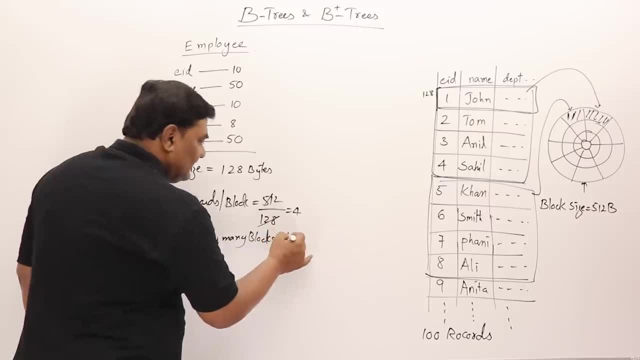 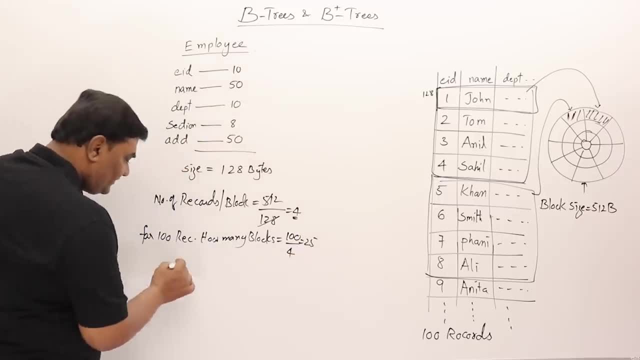 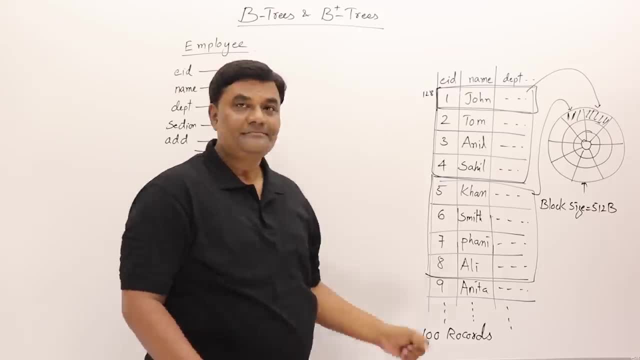 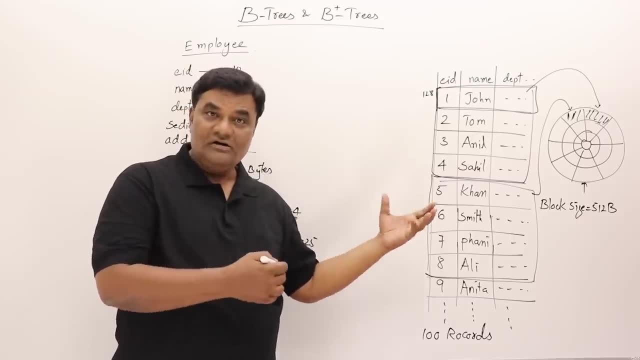 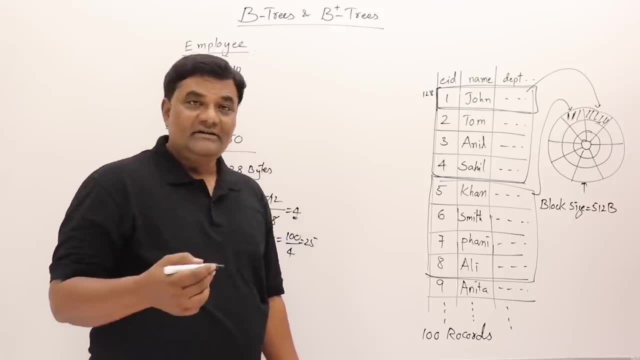 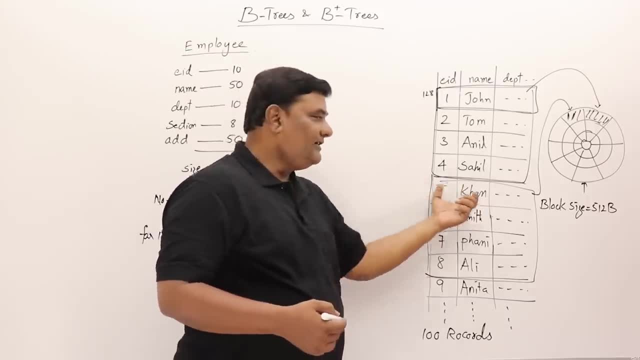 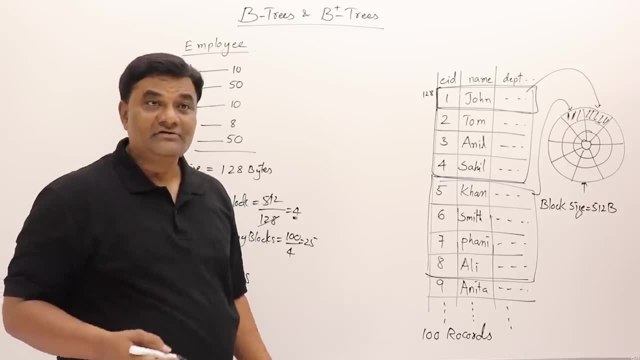 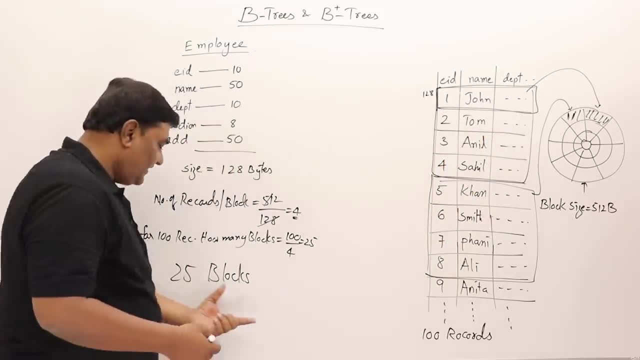 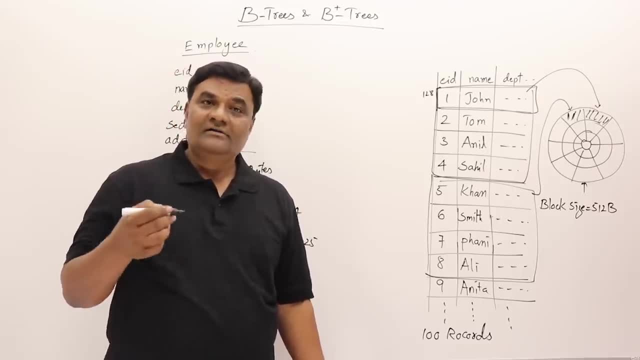 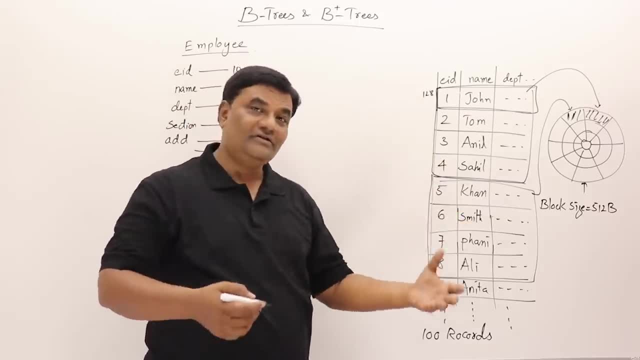 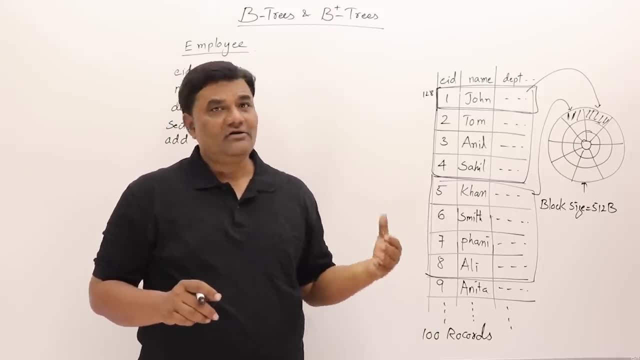 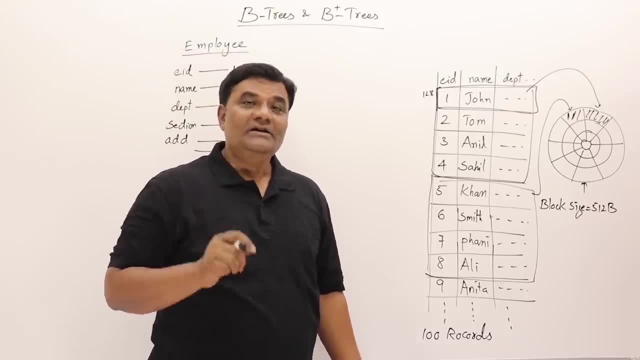 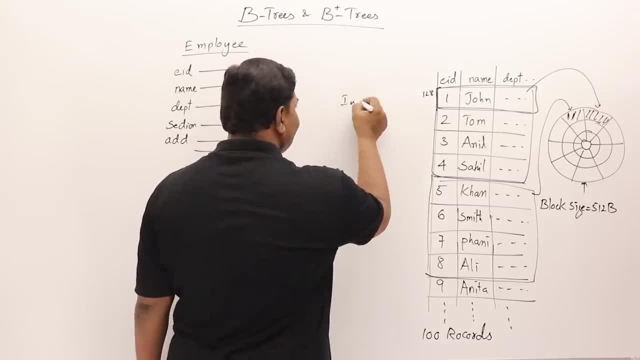 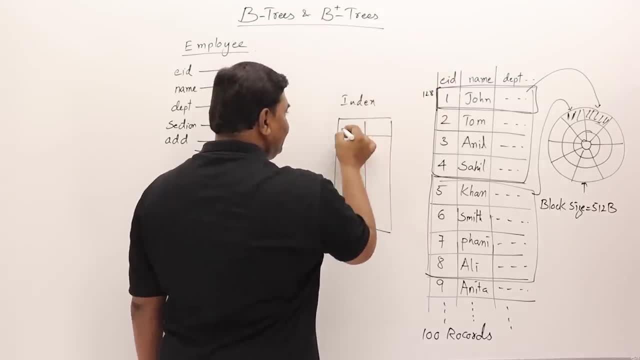 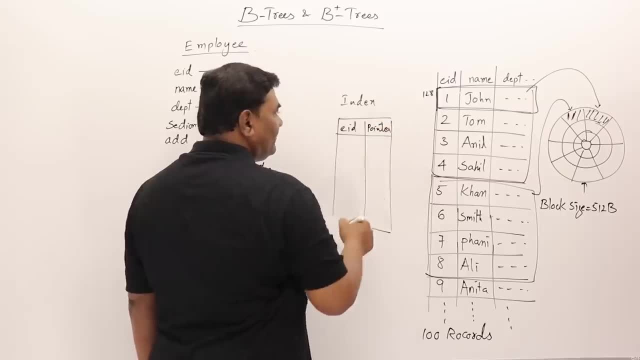 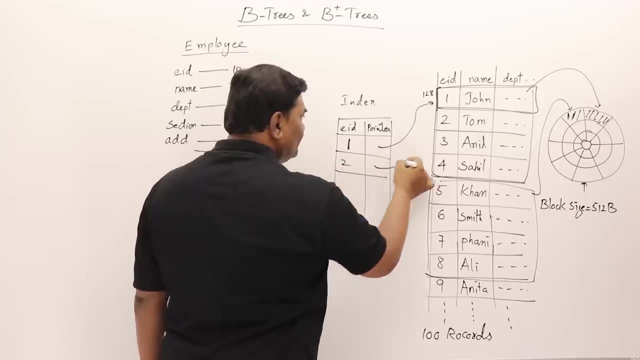 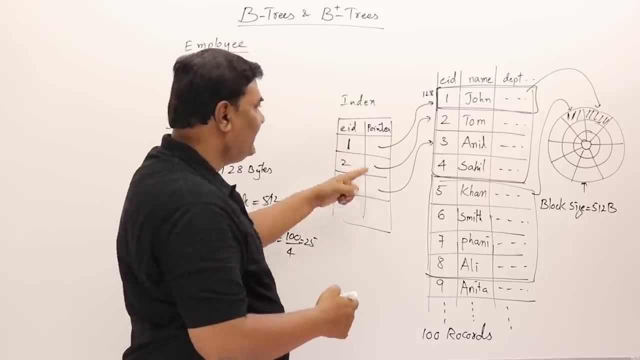 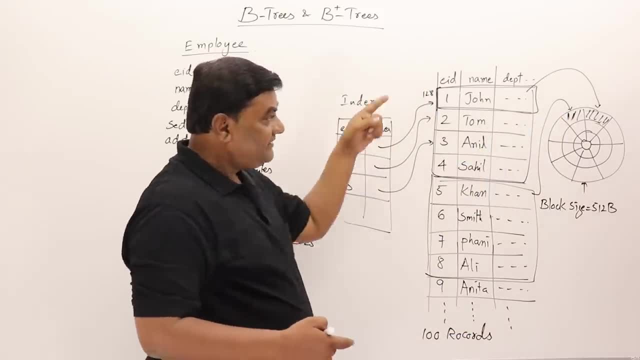 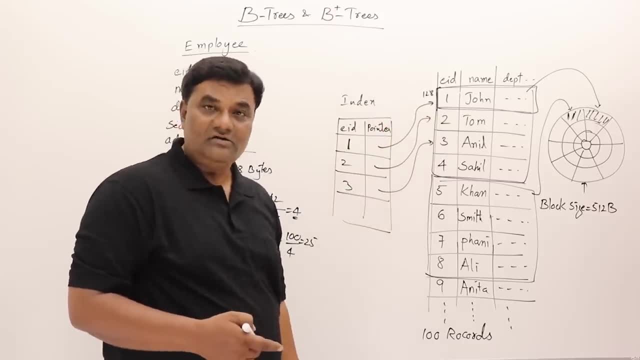 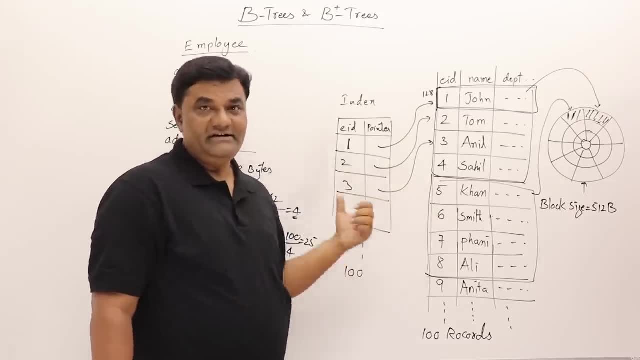 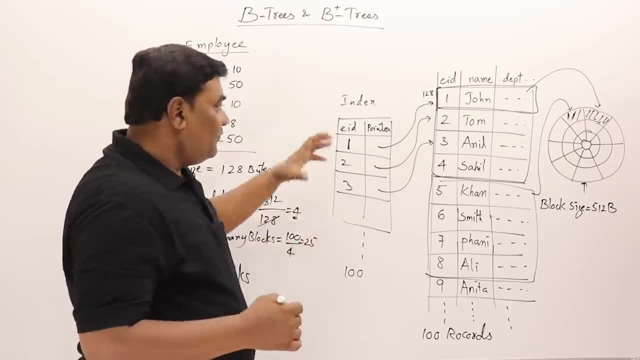 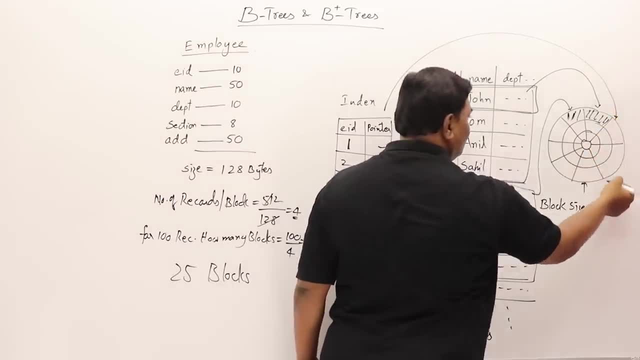 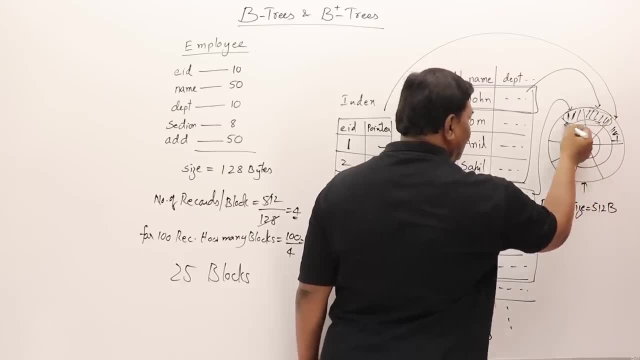 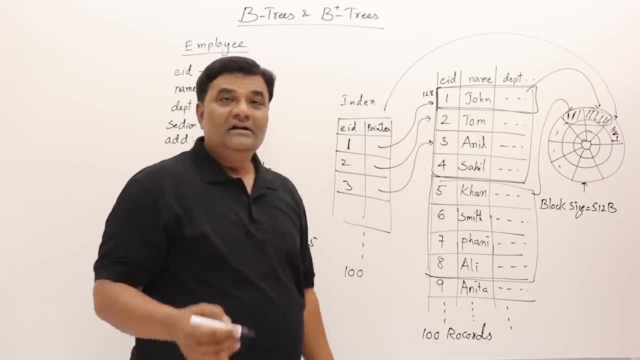 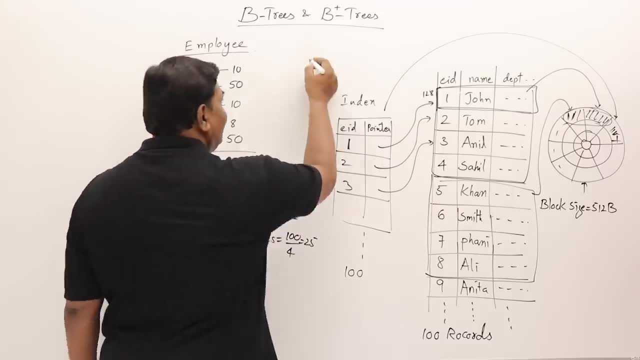 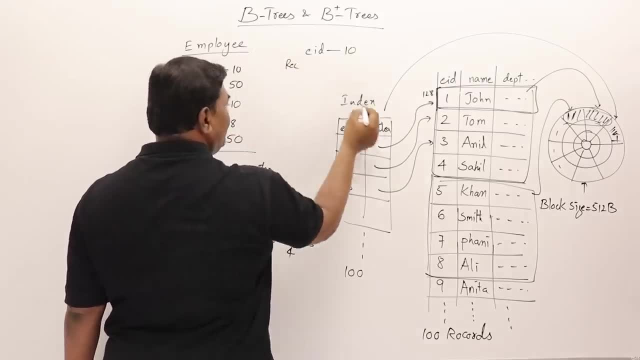 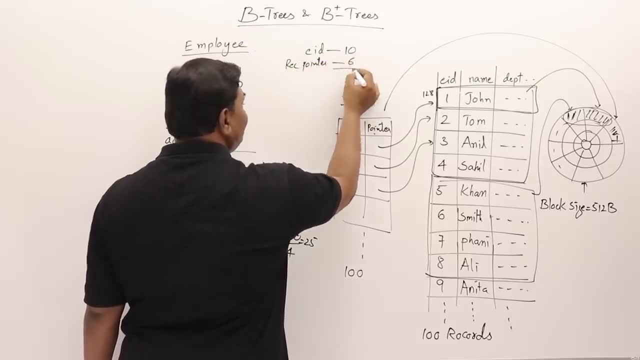 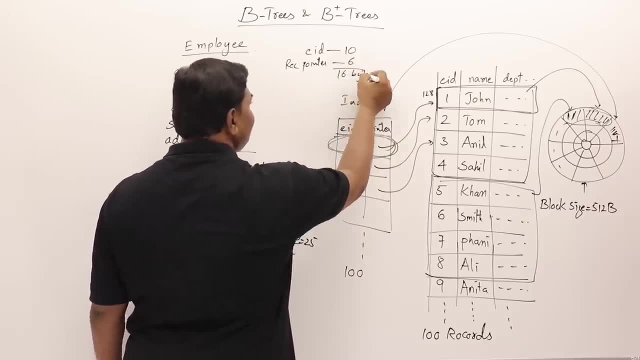 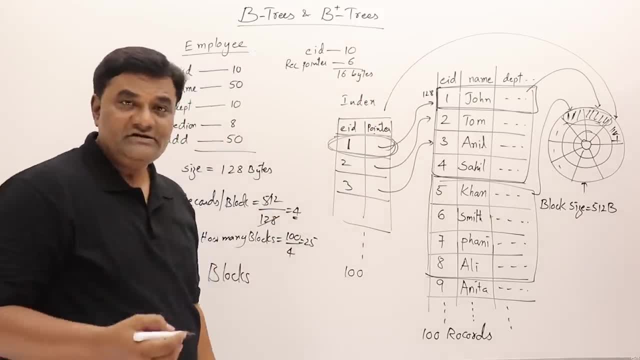 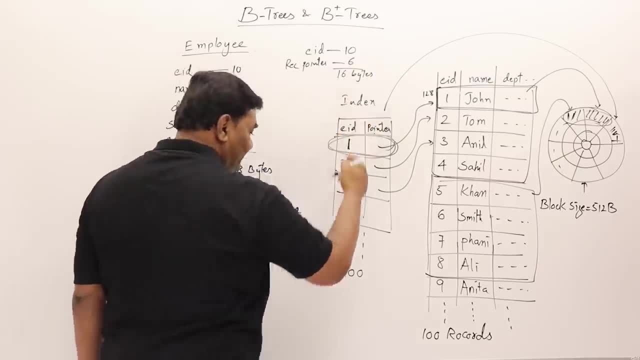 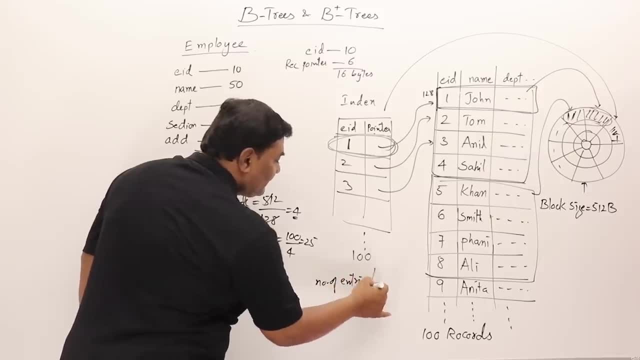 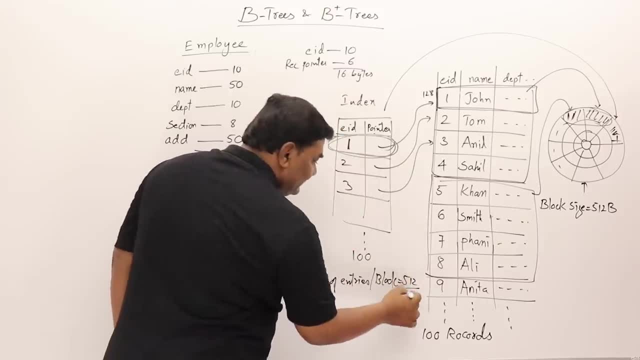 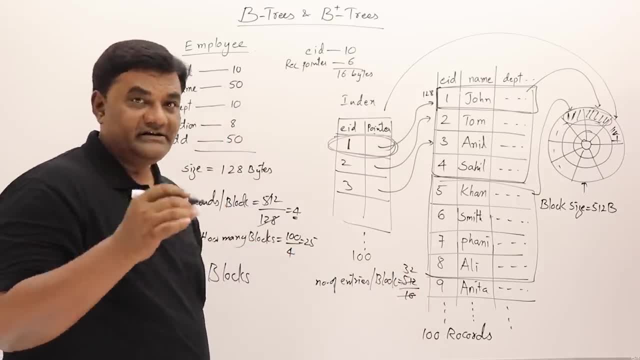 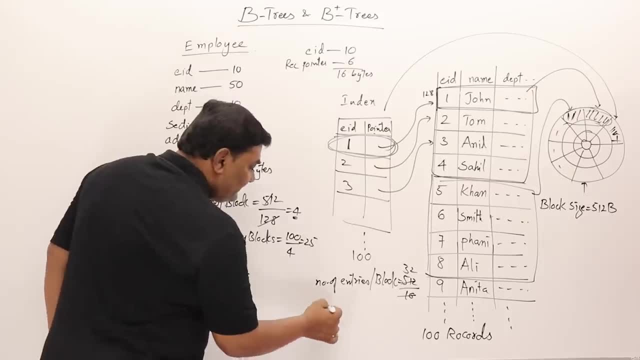 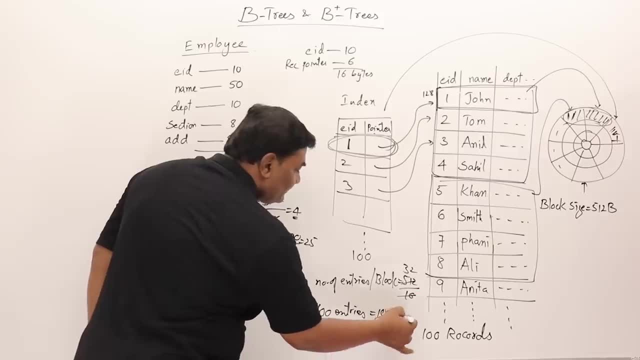 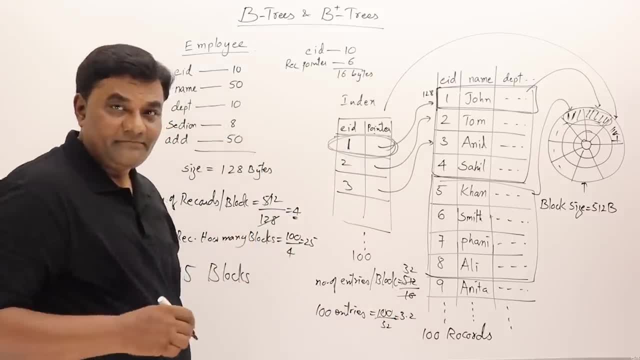 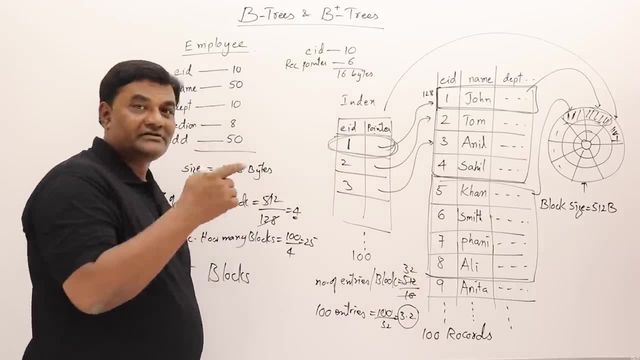 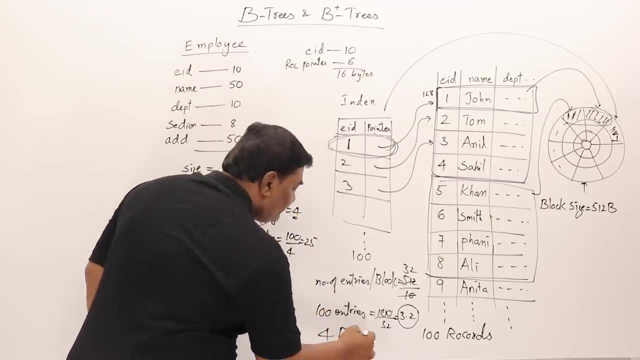 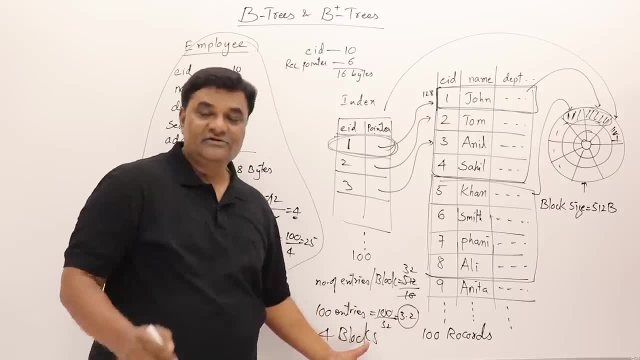 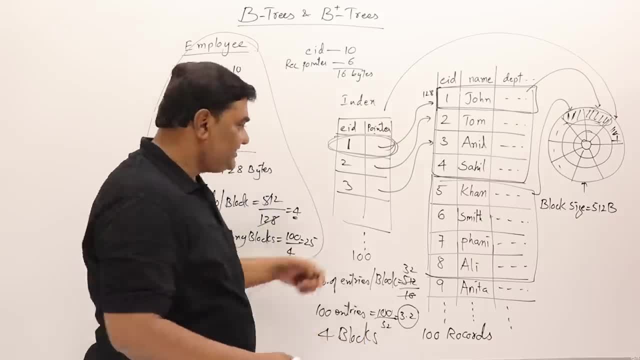 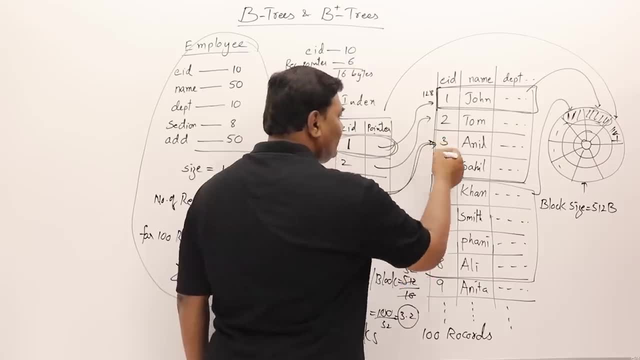 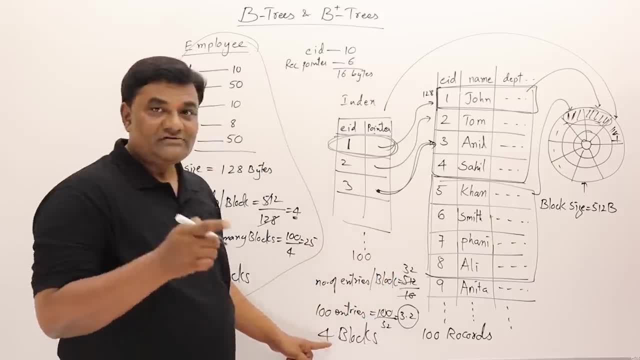 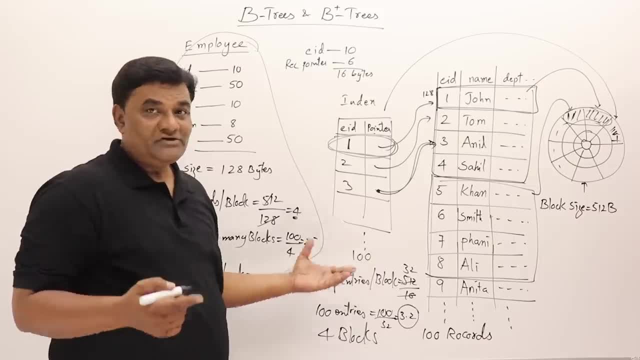 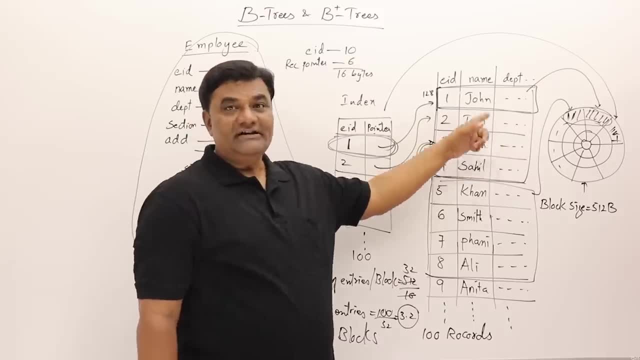 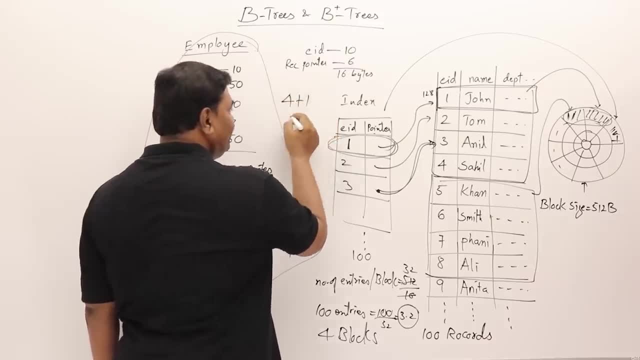 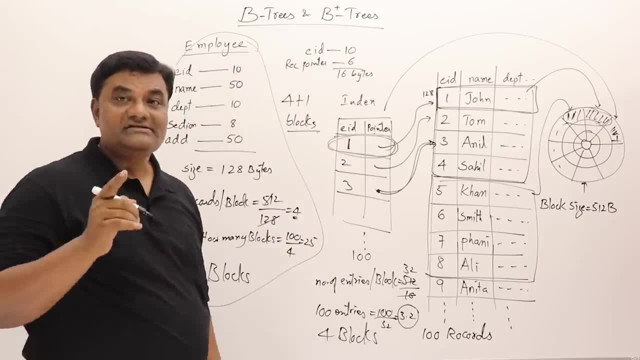 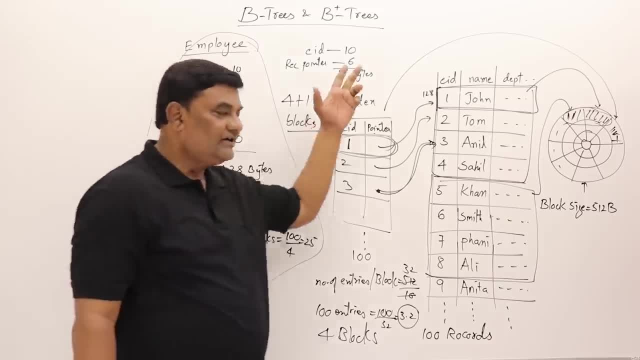 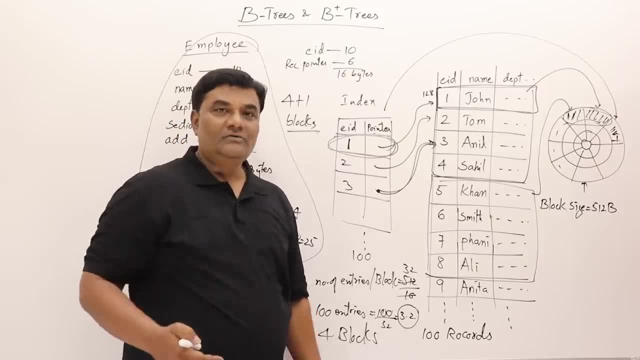 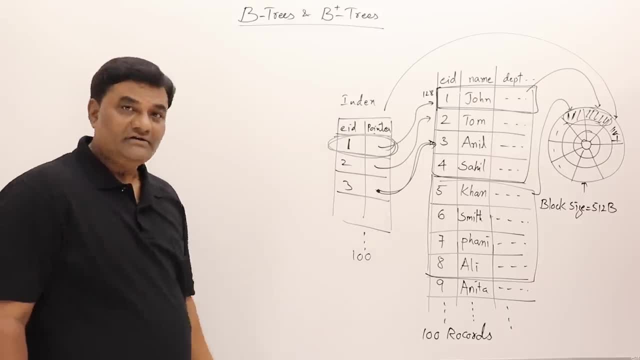 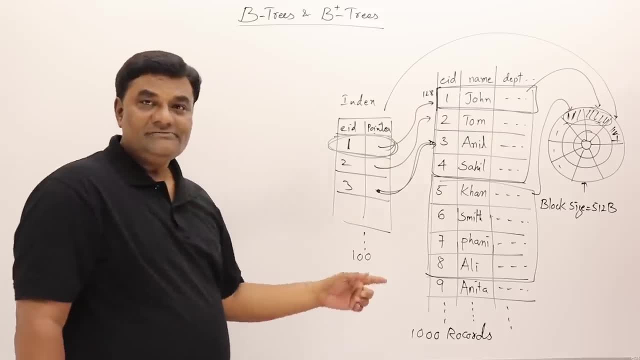 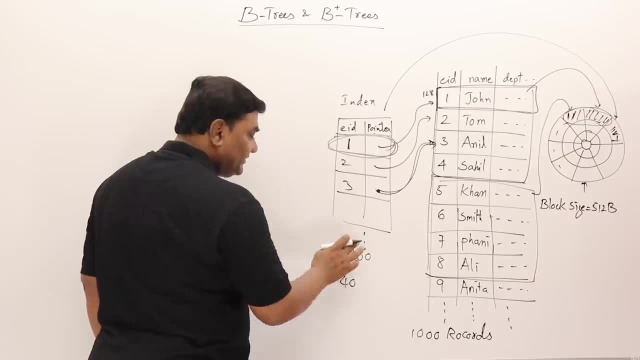 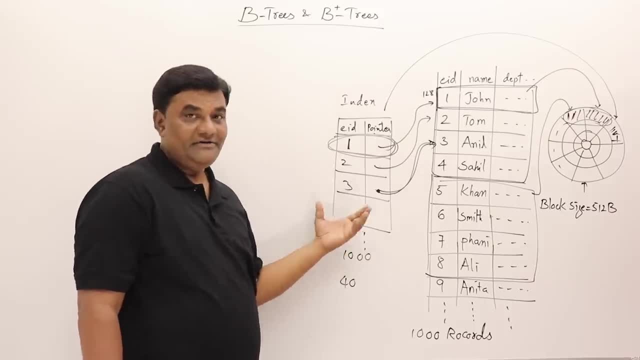 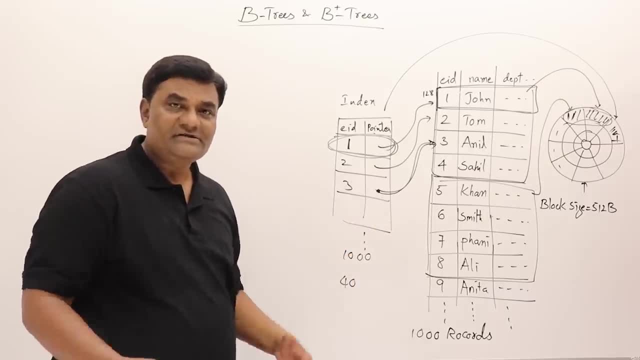 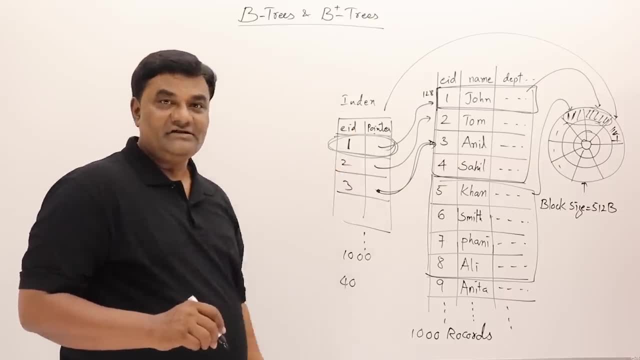 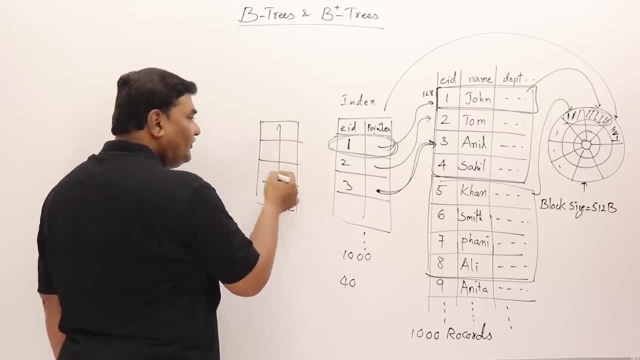 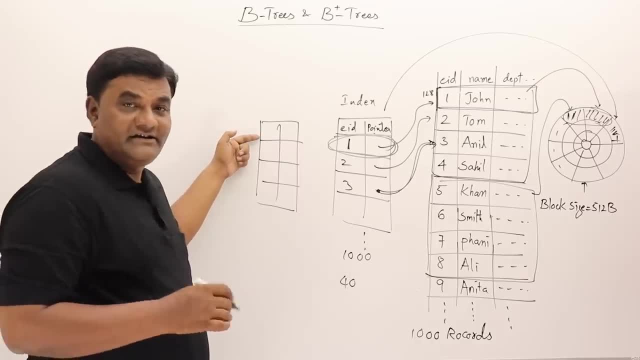 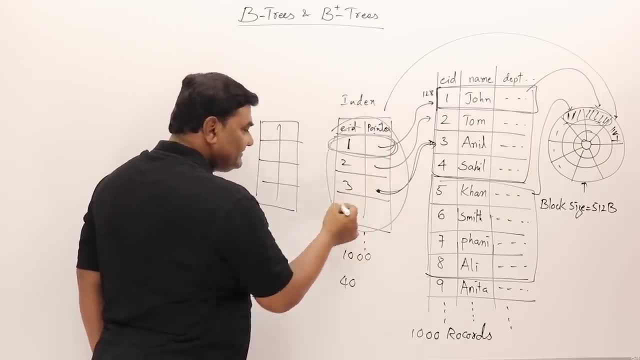 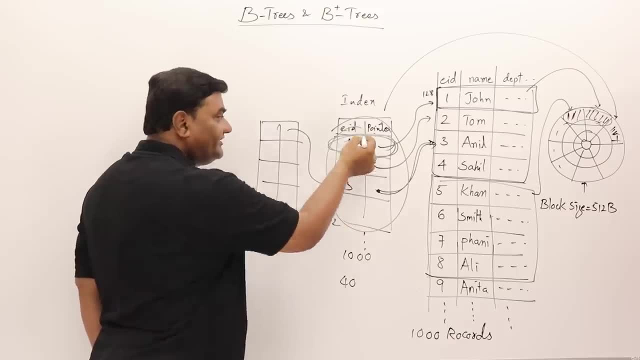 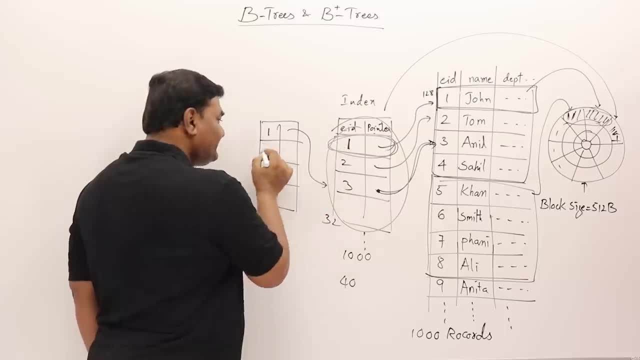 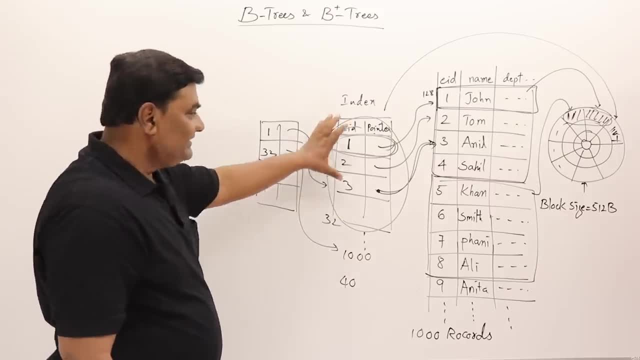 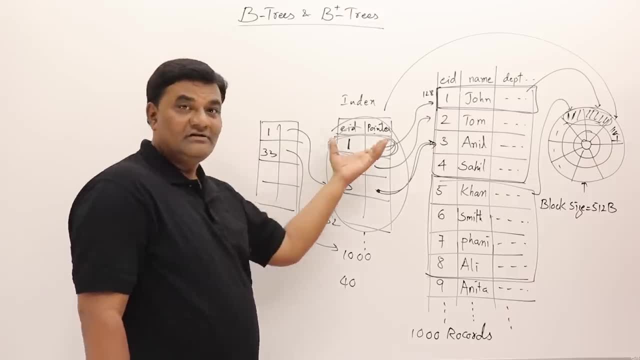 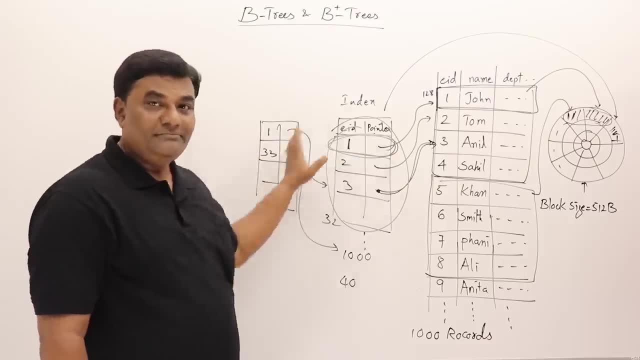 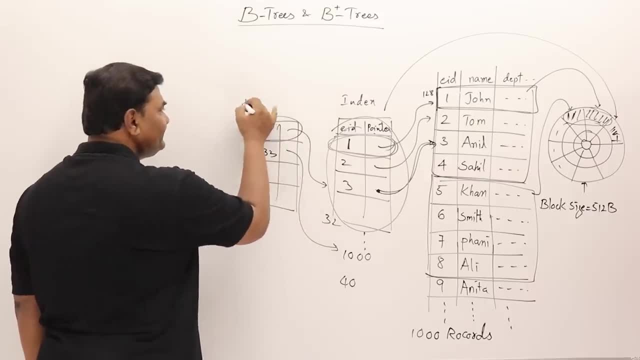 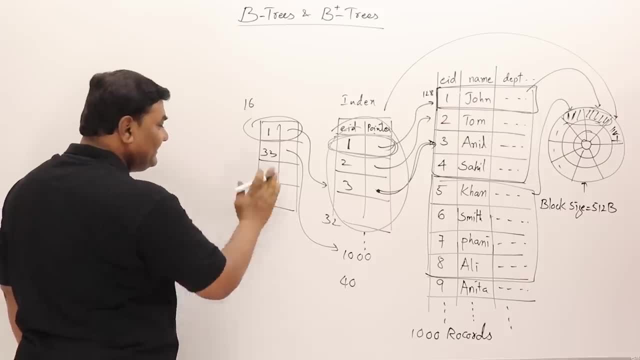 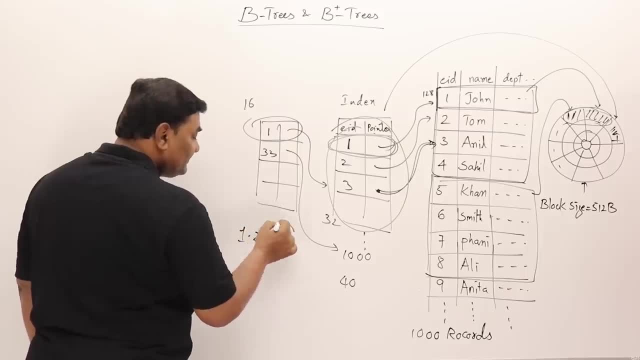 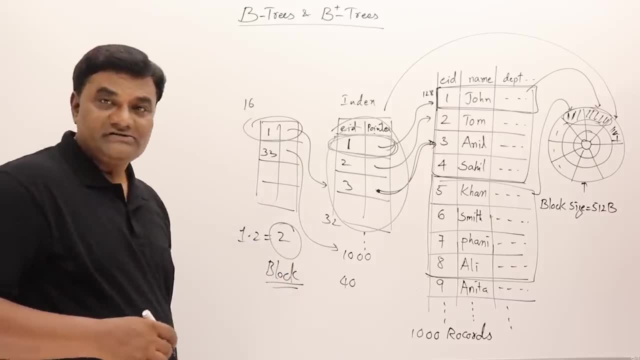 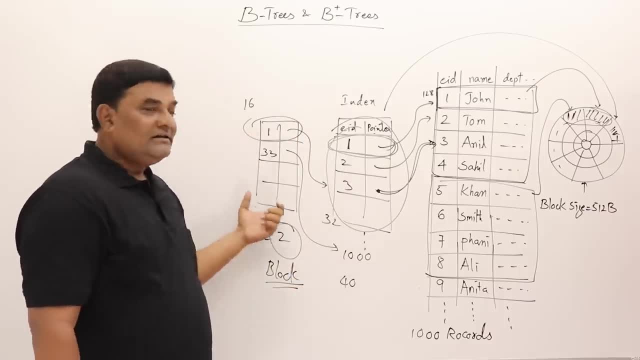 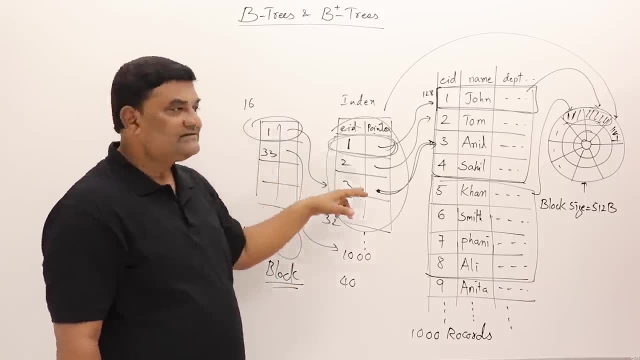 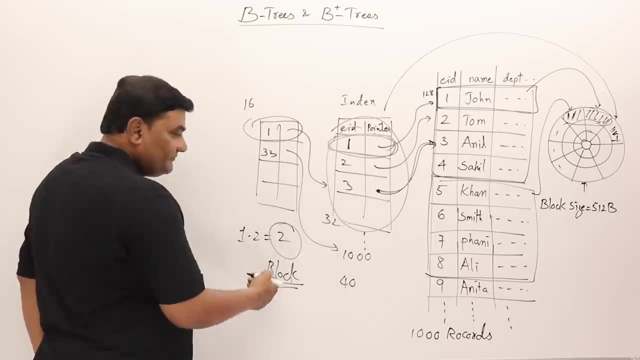 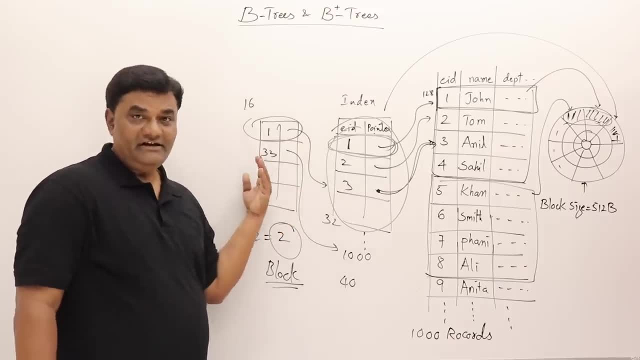 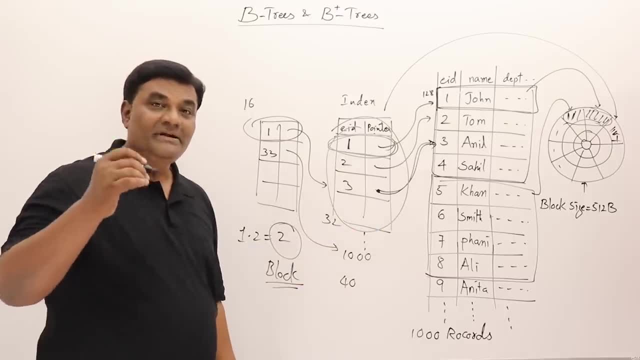 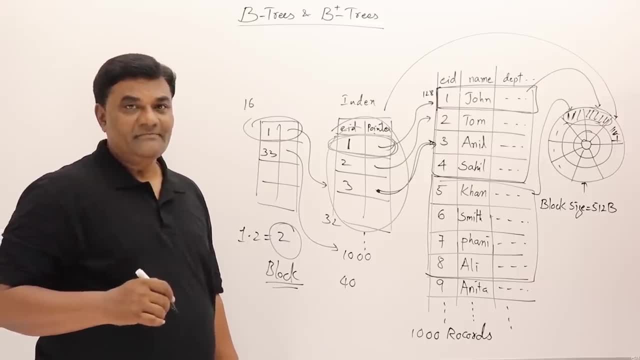 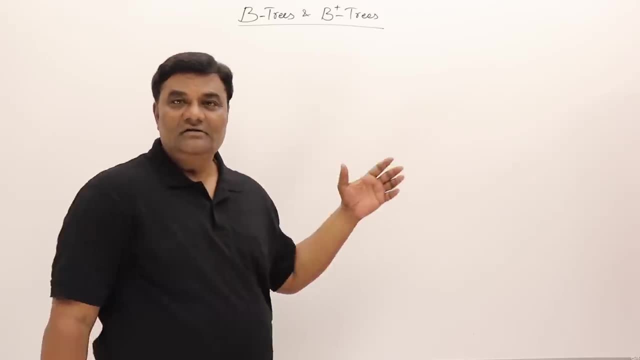 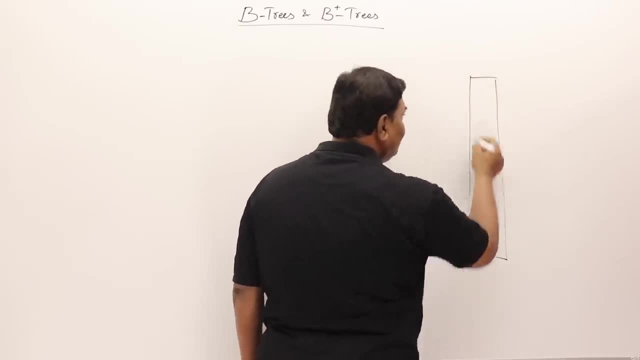 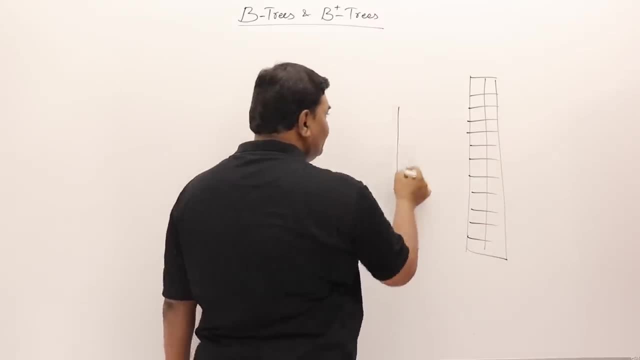 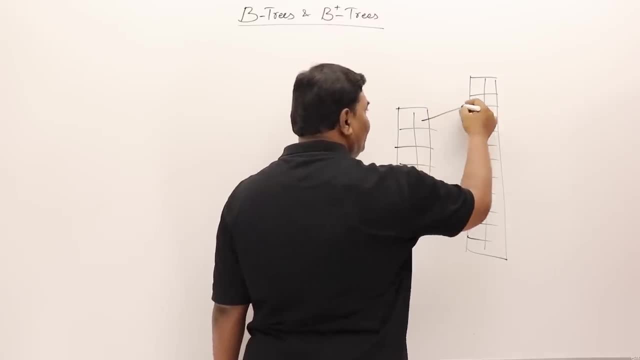 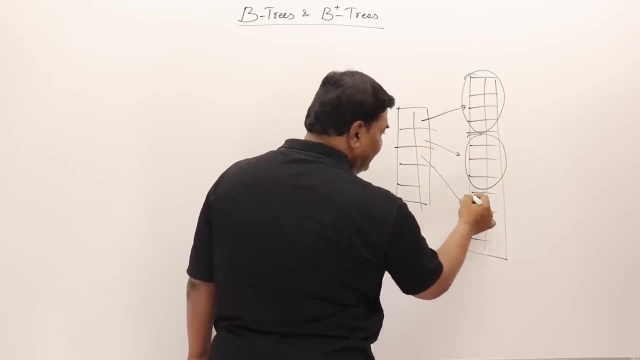 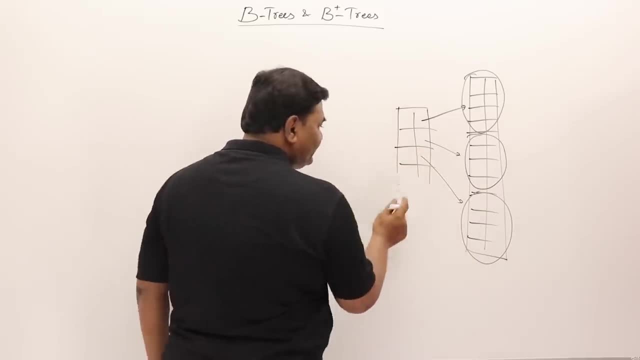 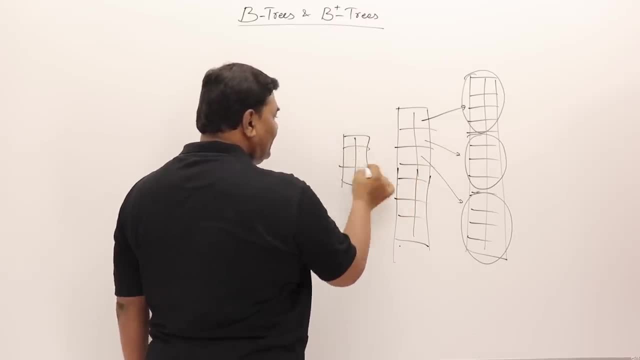 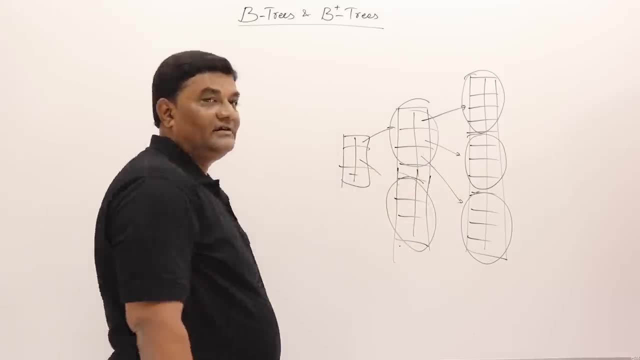 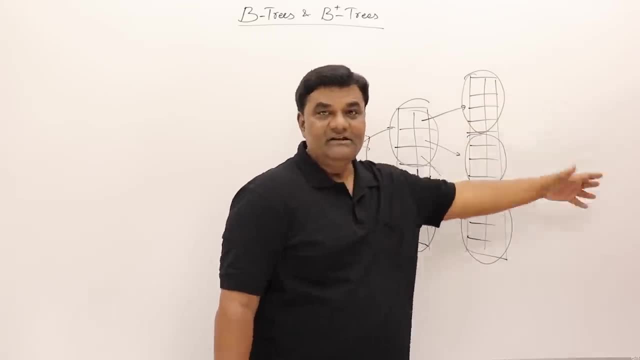 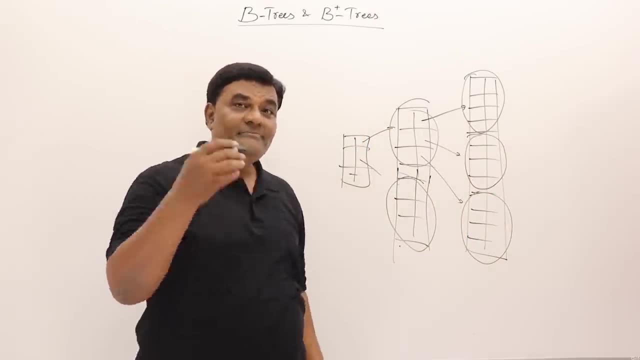 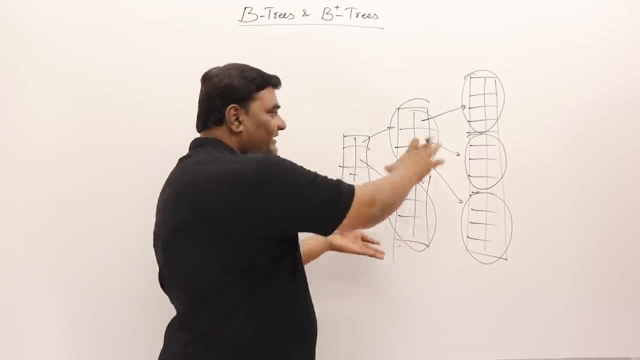 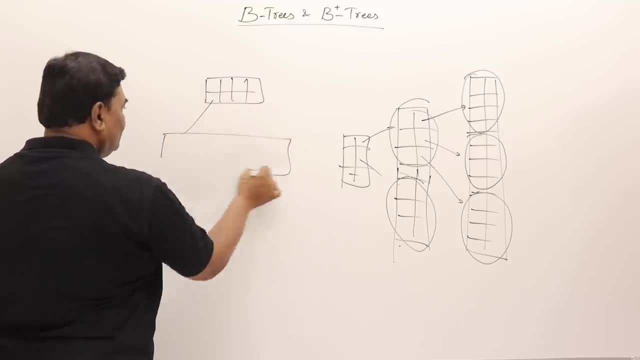 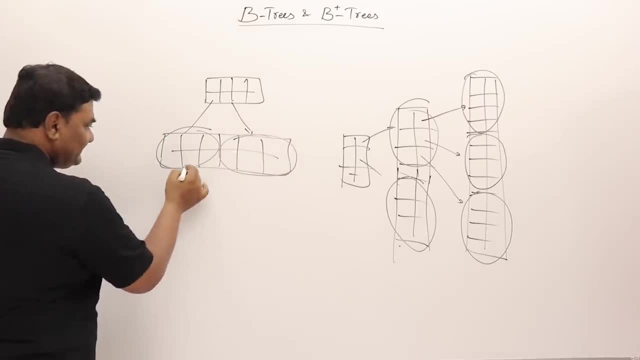 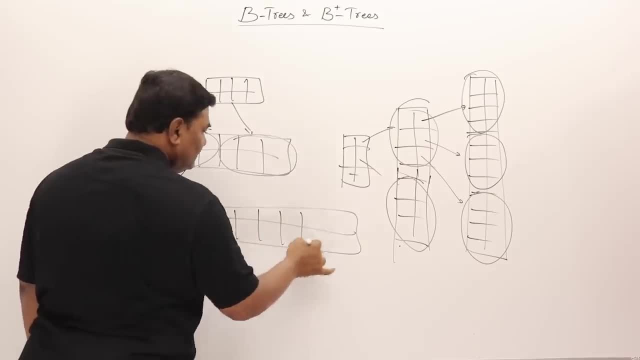 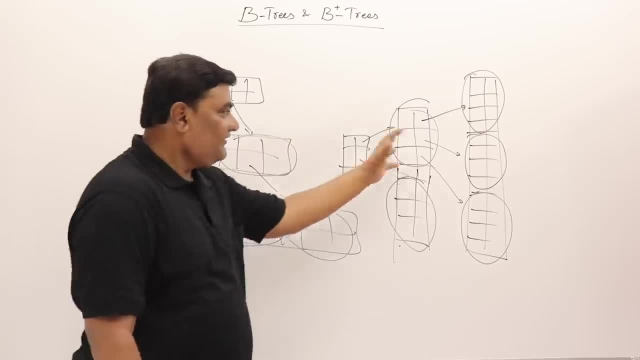 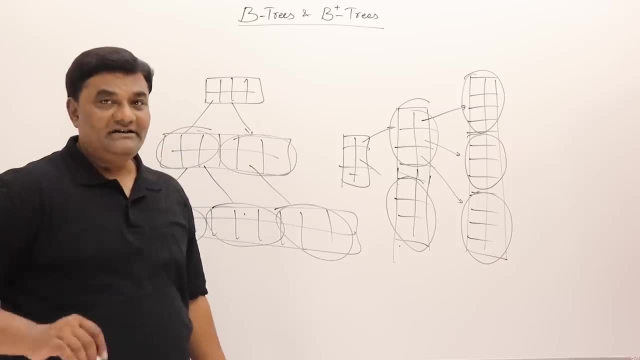 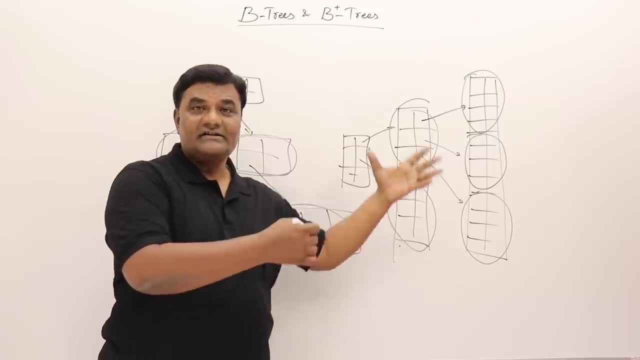 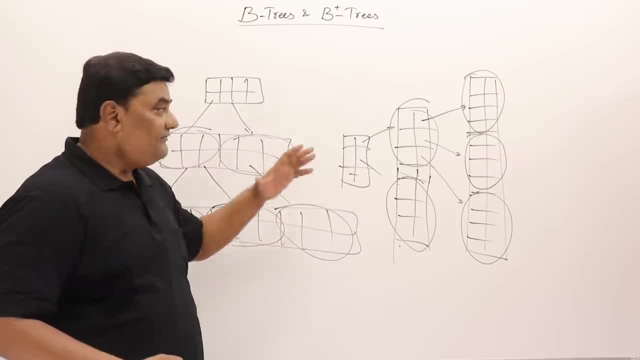 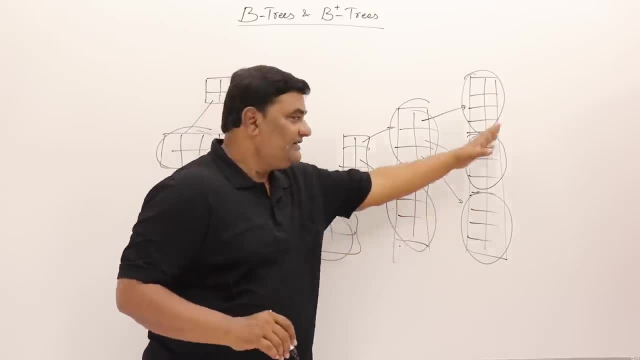 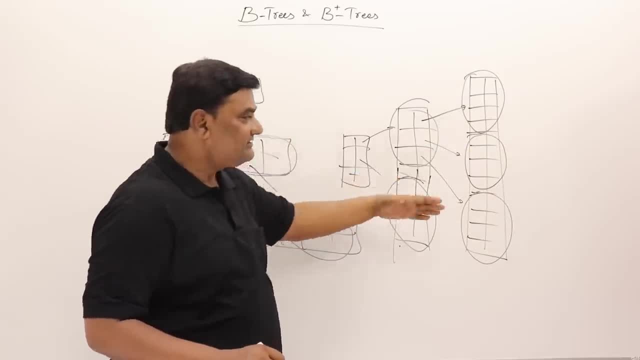 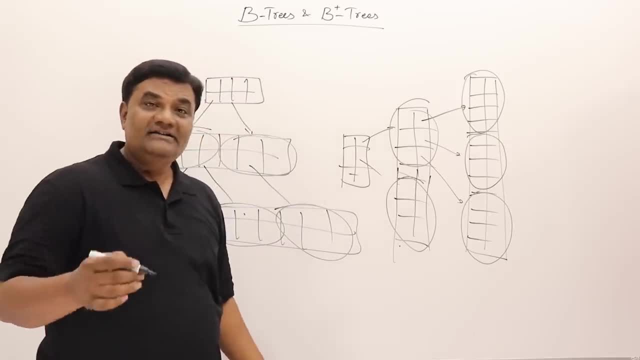 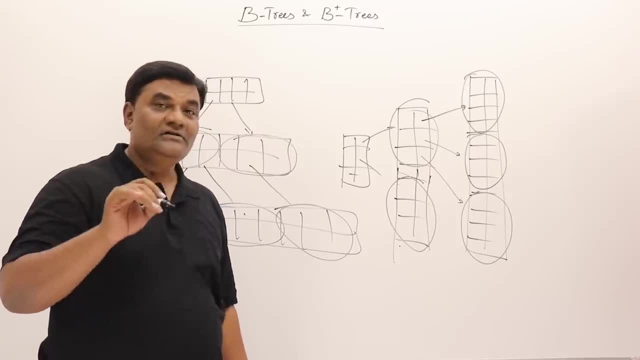 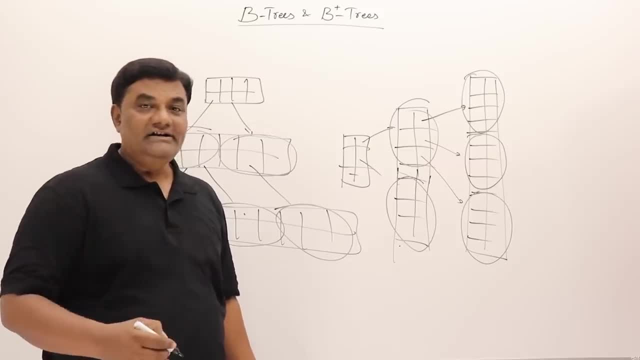 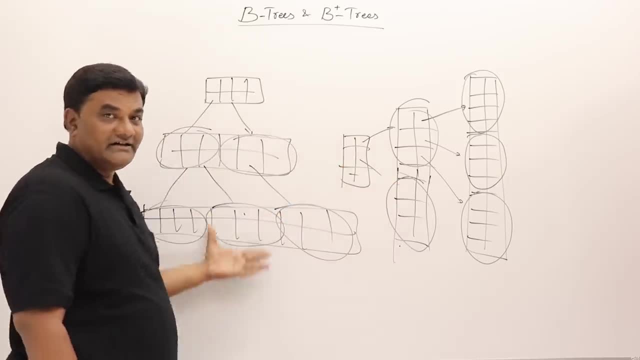 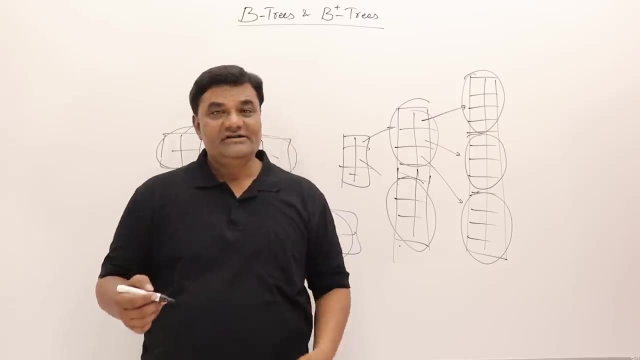 If you know all these topics then you can understand perfectly what B and B-plus trees and B-plus trees are. indices are looking like a tree. if I just turn their side up then it looks like this. B-trees and B plus trees are actually originating from M-way search trees. 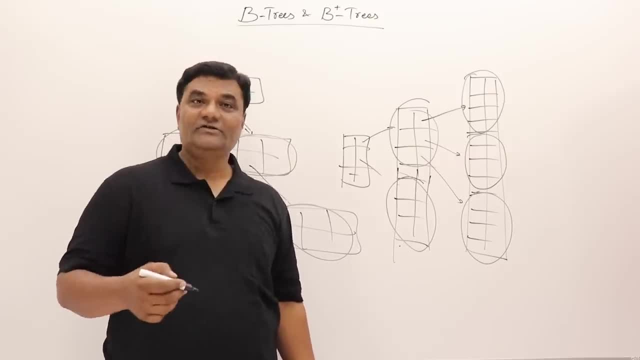 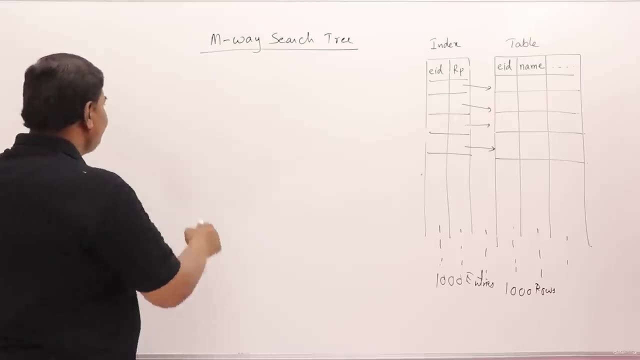 So next I will discuss what are M-way search trees. then, finally, we will go to B-trees and B plus trees. Let us talk about M-way search tree. See for knowing about M-way search tree. let us recall about binary search tree, which is: 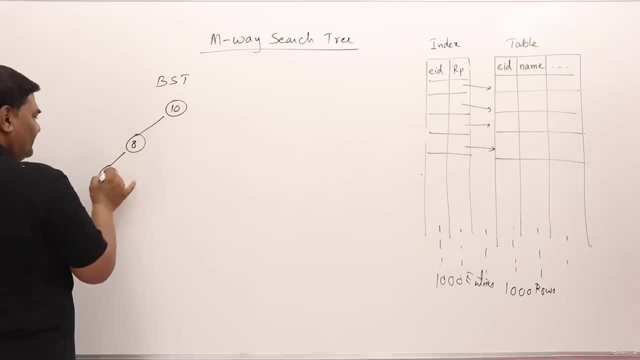 useful for searching purpose and for searching any key value. we start from the root and if the key value is smaller we go on the left hand side. if the key value is larger, we go on the right hand side. like this is a binary search tree. If I am searching for 15, then 15 is greater than this. I will go this side. 15 is smaller. 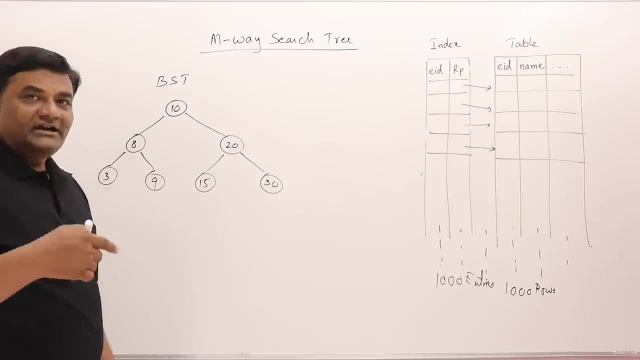 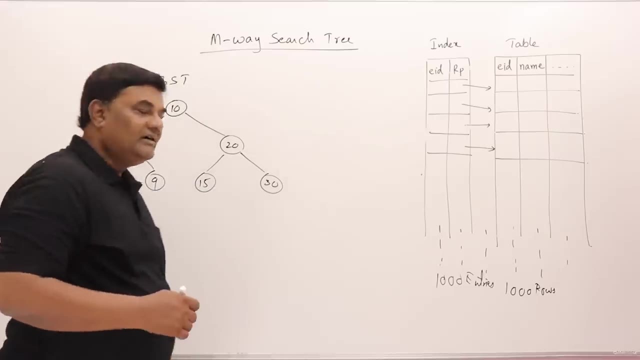 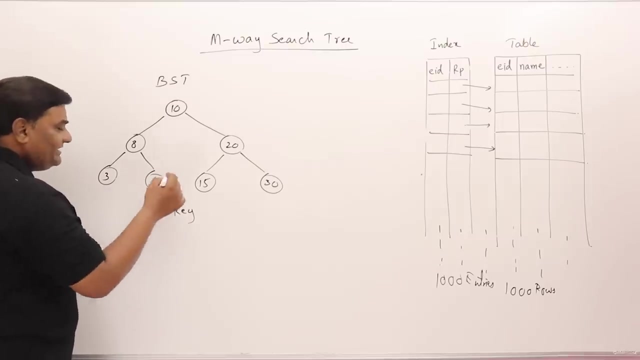 than this. so I will go this side and it is found. So we know that the smaller keys are arranged on the left side and the larger keys are arranged on the right side. This is what is done in binary search, In binary search tree: how many keys we can have per node, just one key and how many children. 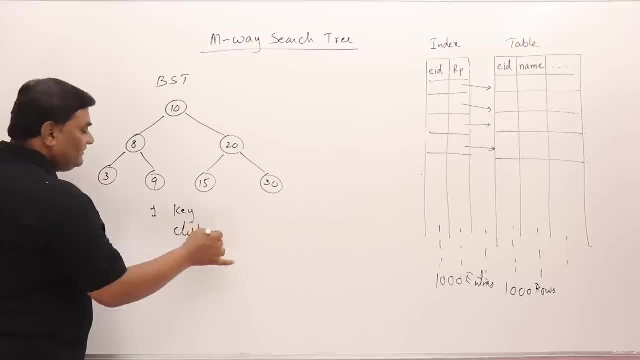 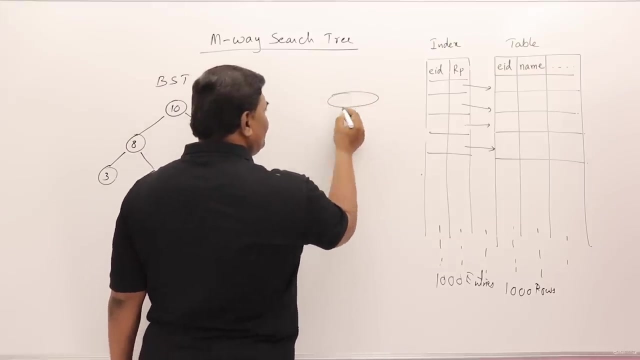 each node can have how many children? there can be two children. each node can have maximum two children. so that's why it is called as binary tree. binary by means two children. So it means: can we have a tree with more than two children or more than one keys? let us 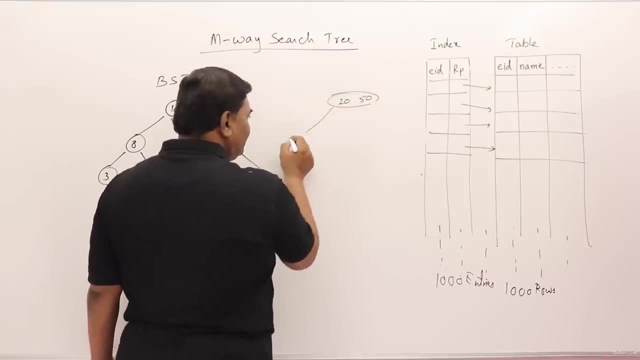 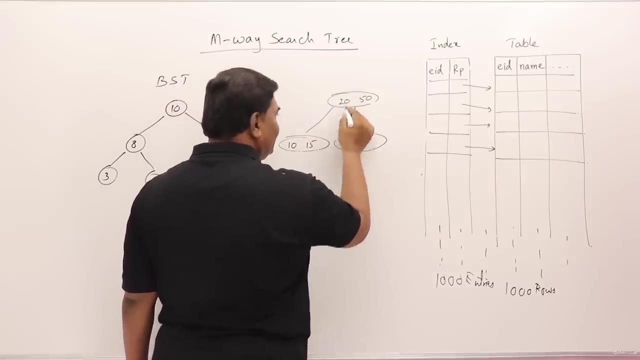 check: 20 and 50. these are the two keys. now, this side, I will have the keys which are smaller than 20, so that is 10 and 15, and here I will have the keys that are in between these two, that is 30, 35, and here I will have the keys that are greater than this, so that is 60 and 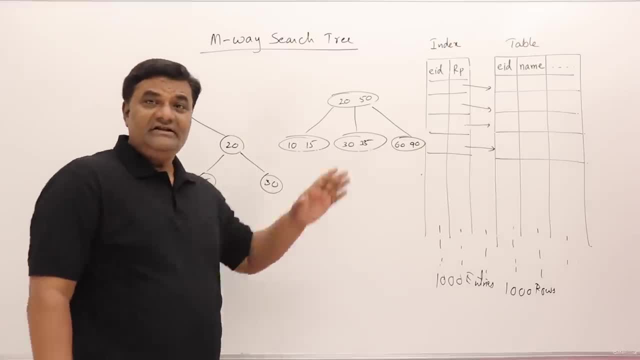 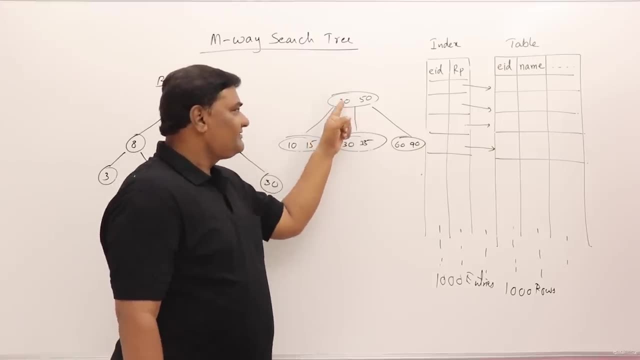 90. So, yes, we can have a search tree like this also. this is a search tree. this is the following: the idea of same as binary search tree. see, the keys are arranged such that they are in the increasing order. So if you see the keys here, see, first key is smaller than second key and smaller than. 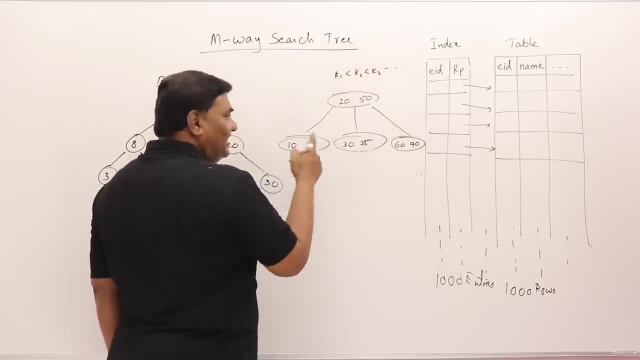 third key. if you have more keys, they will be arranged like this, and if I am searching for 30, then I will start from here. 30 is greater than 20, 30 is less than 50, so it must be in this child. come here. 30 is found. 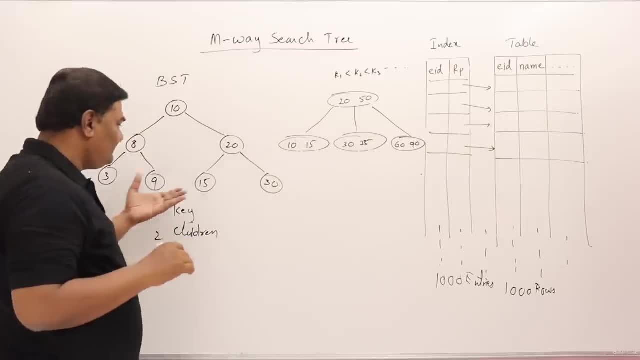 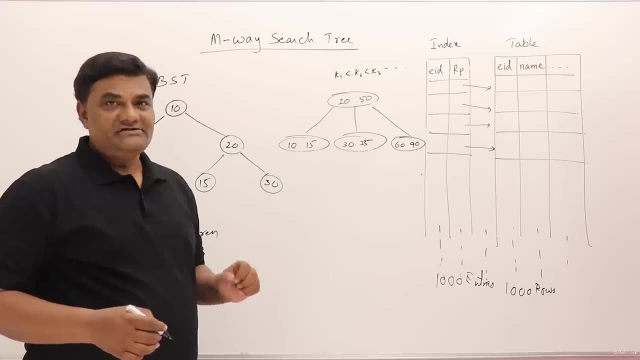 So, no doubt, the amount of time taken for searching is little more than binary search tree, but the approach of searching is same. So these trees are called as M-way search tree. So these trees are called as M-way search tree. So these trees are called as M-way search tree. 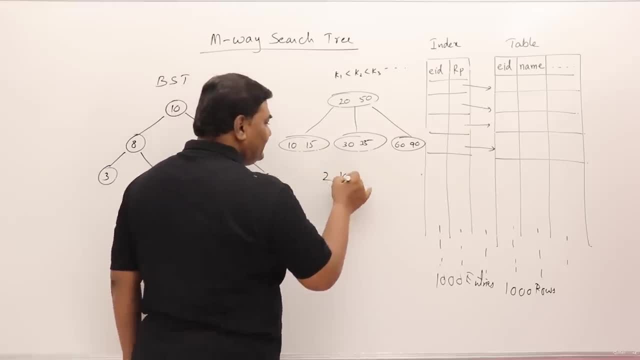 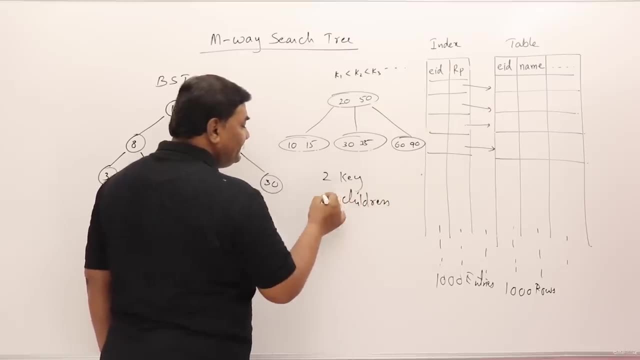 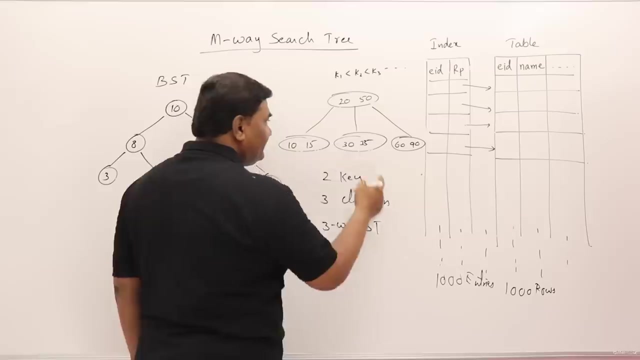 So what is this M-way? see how many keys it is having. in this example it is having two keys, then how many children it is having. so each node can have maximum three children. so this is three-way search tree. this is a three-way search tree. this is called as three-way. 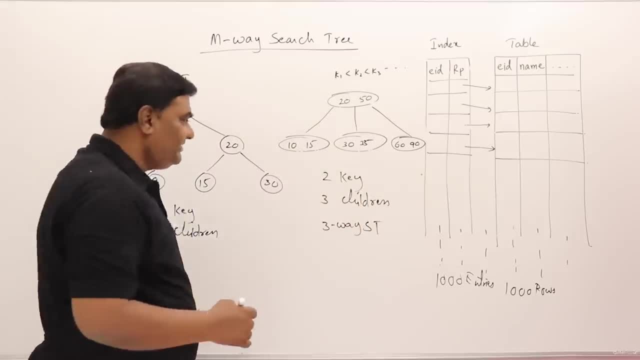 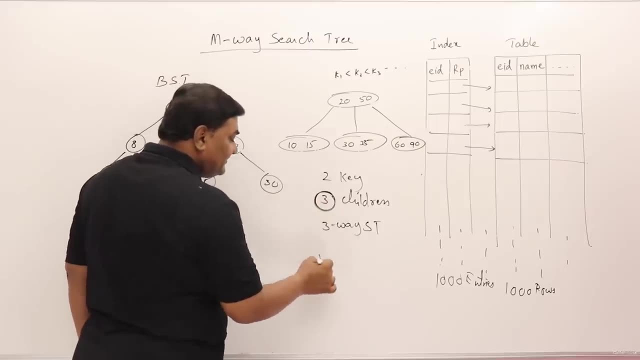 search tree. So in this way, M-way search tree means what a search tree in which each node can have at most M children. M-way search tree, so each node can have at most M children. so how many keys? M-1 keys. So M is based on the number of children, that is the degree of a node. so M-way search trees. 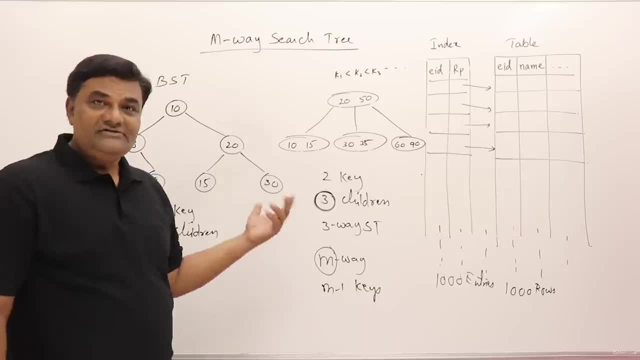 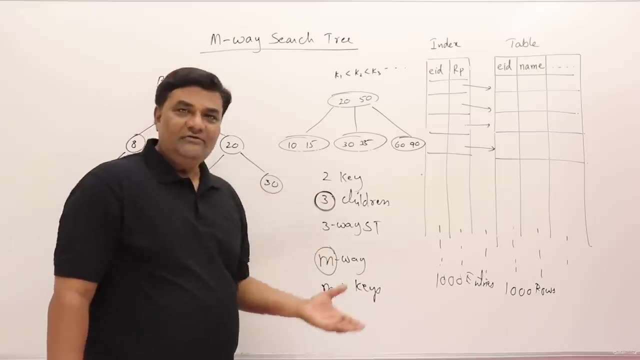 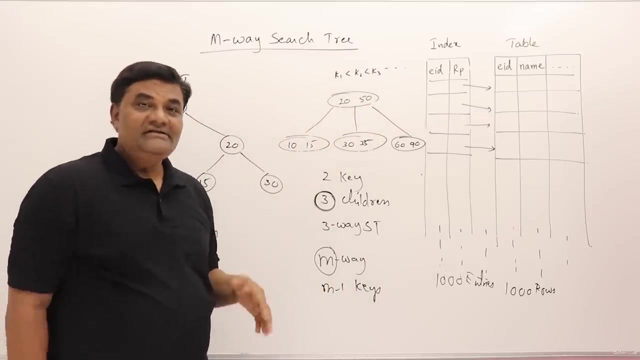 are the extension of binary search trees. you can say, or else you can say: binary search tree is a type of M-way search tree with a degree two, so you can have degree three also, degree five also, degree hundred also, degree thousand also, So it means you can have hundred keys here, and each node can have hundred keys and hundred. 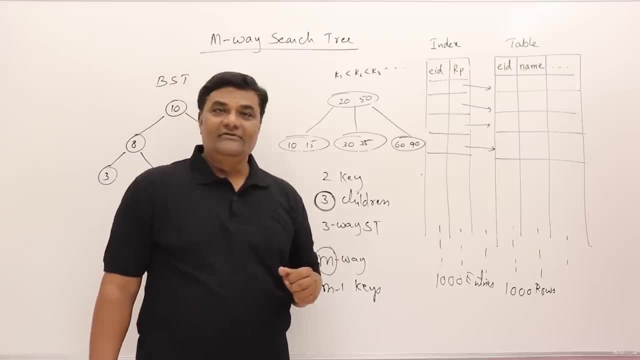 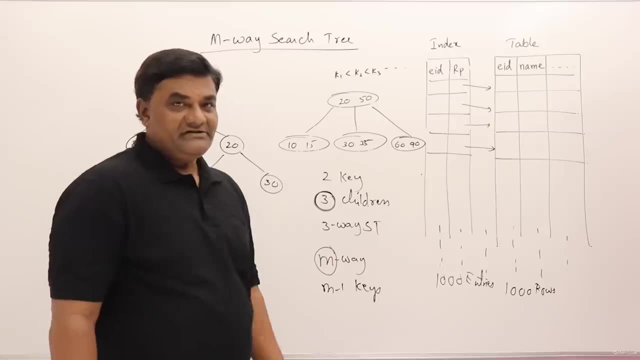 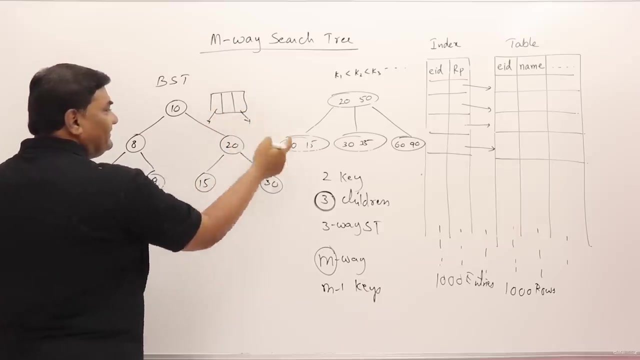 plus one children, so you can have any degree of search tree. This is about M-way search tree. let us look at the node of M-way search tree. like for binary search tree, how we prepare a node is: we will have data here and two children then. 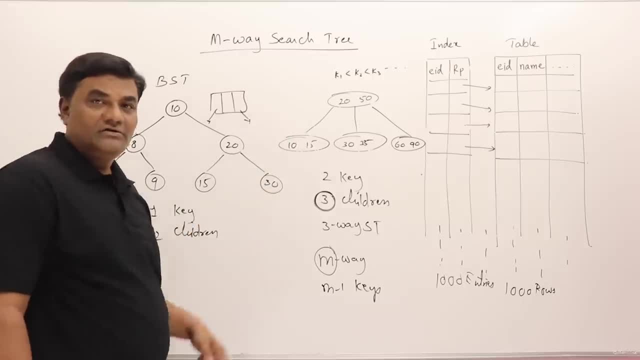 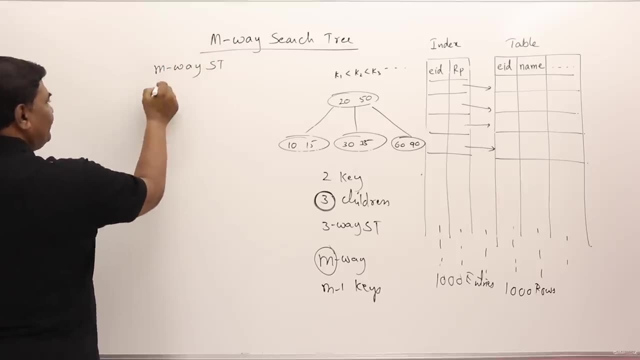 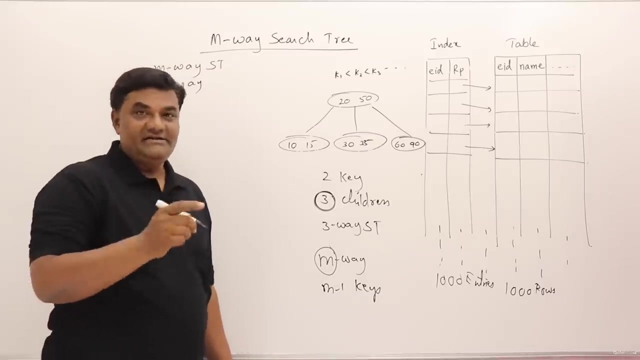 here you need more number of children. so let me draw the node for this one. if the M-way search tree is Search tree, STM writing is suppose four-way search tree means each node can have four children and three keys. let me draw a node structure. 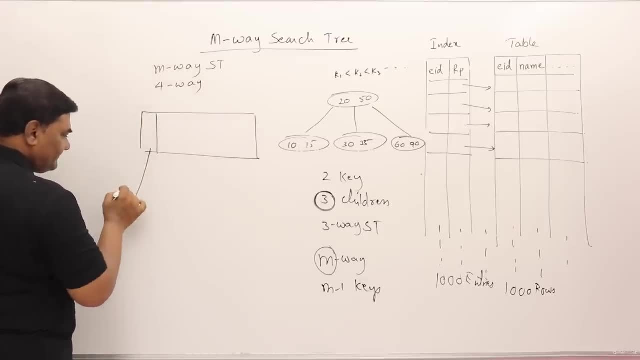 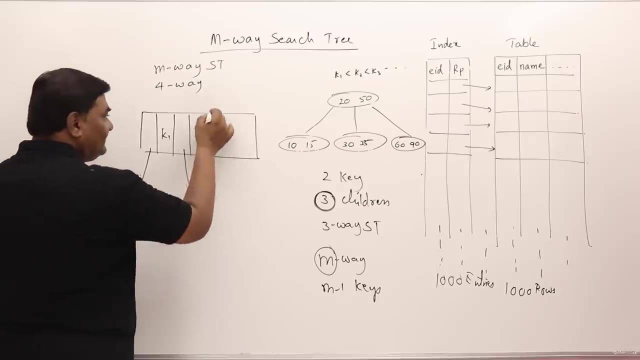 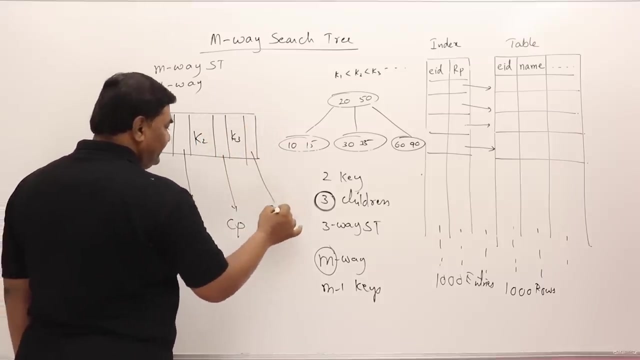 This should be a child pointer, pointer to the child, and this is key one. and again, this is a pointer to a child and this is a key two, and this is a pointer to a child and this is key three, and this is a pointer to a child. so four, child pointer. so this is four-way. 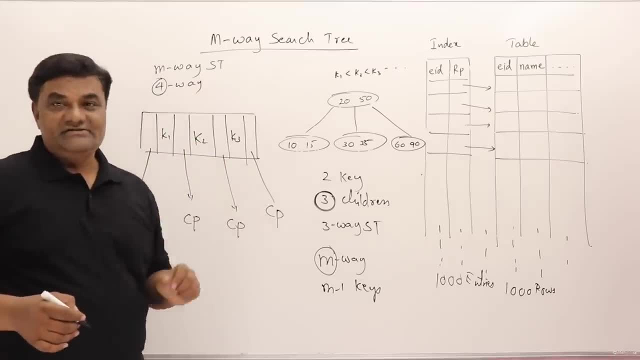 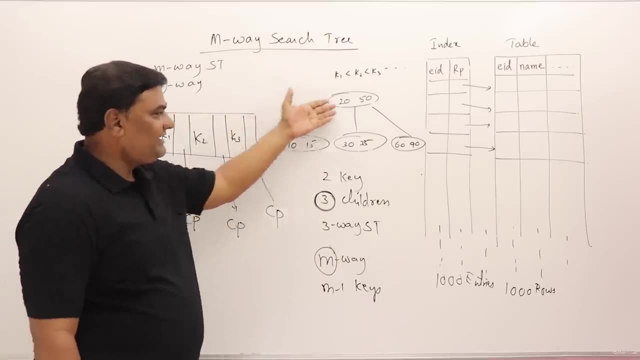 and when it is a four-way then there can be three keys. that is M-way search tree. a node can have M minus one keys. so it is just like this. this is diagrammatic representation and if you are making a data structure, then the node structure looks like this. so if there 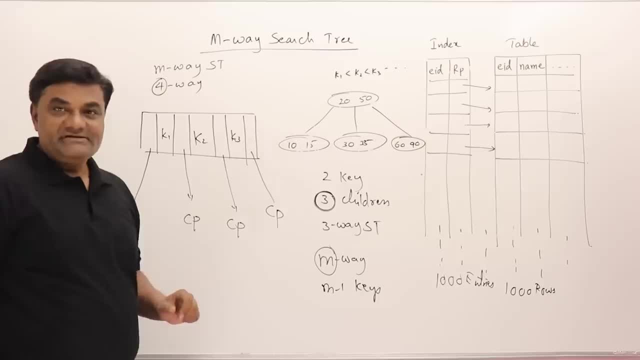 are M children, then M minus one key spaces are required. Now next, Can we use this search trees, these nodes, structure, for preparing index? let us see. so I will try to use this for making index. so let us check how we can do this for four-way. 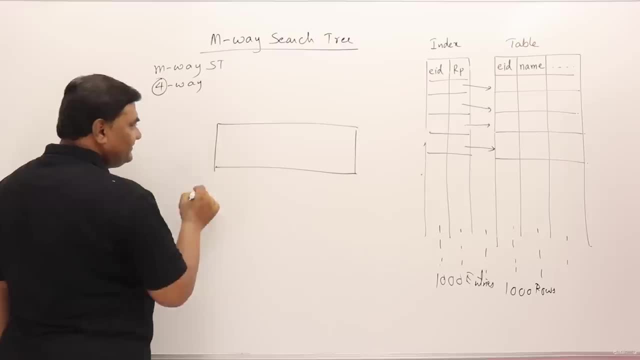 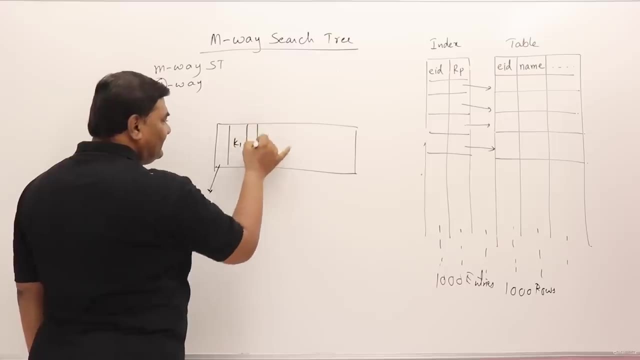 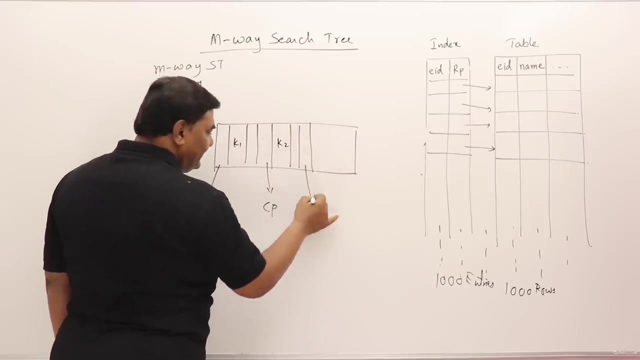 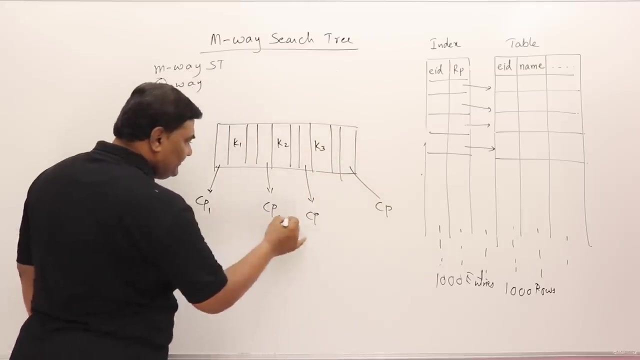 search tree where there can be four children. so this is a child pointer. okay, now this is key one and this is next child pointer, Then This Is key two, then this is the next child pointer, then this is key three and fourth child pointer. so child pointer one, two, three, four, then what is this? I am adding? see this after every key. 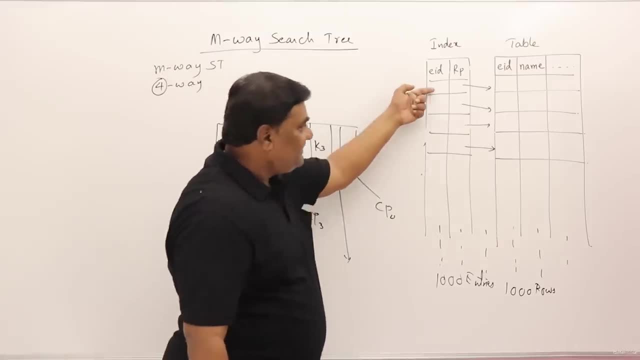 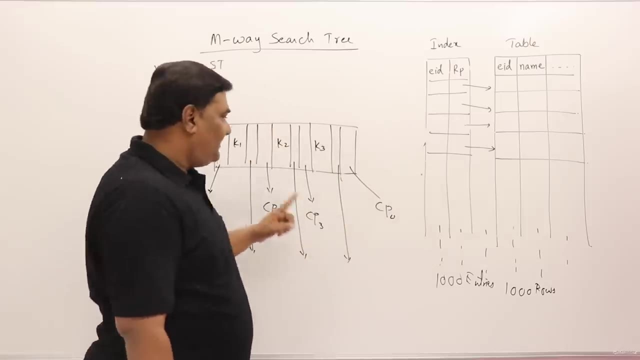 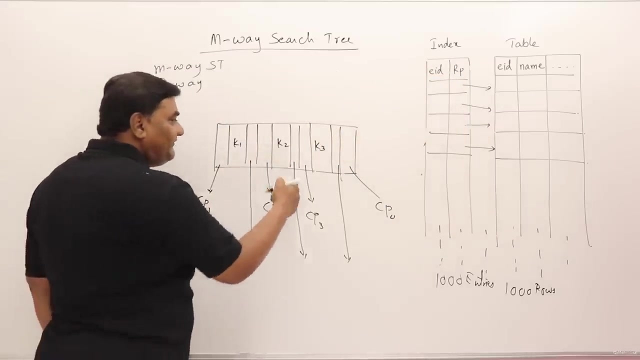 I have a pointer. this is nothing but see. if you have keys here and you are taking a M-way search tree benefit of M-way search tree as an index, then apart from the child pointer, you should have Also a pointer to a record. that is a record pointer. so yes, we will also have a record. 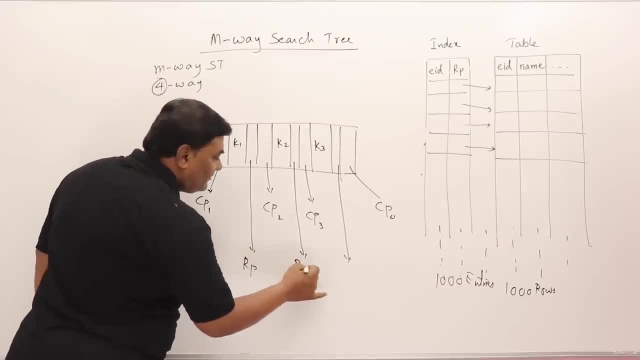 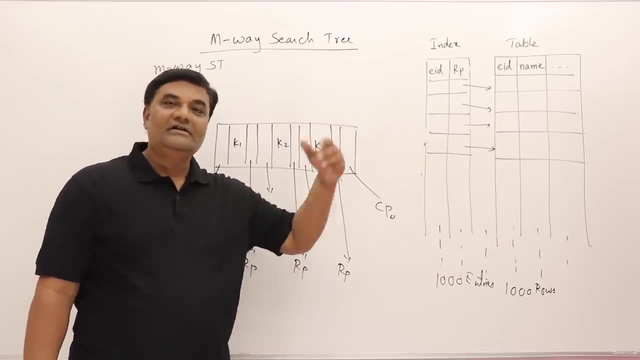 pointer, so this is a record pointer. a record pointer so we can utilize M-way search trees for indices, that is, multi-level indices, like tree, will have multiple levels. so for making multi-level indices we can utilize M-way search tree, but the node structure should be like: 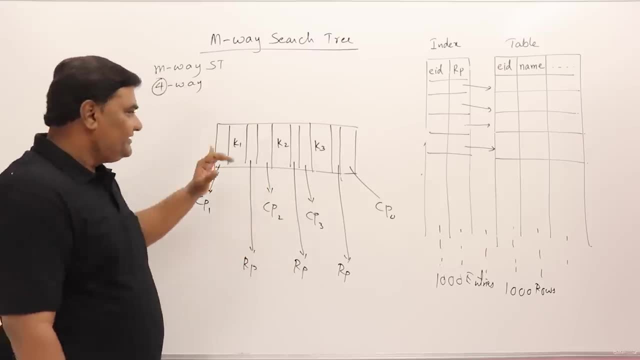 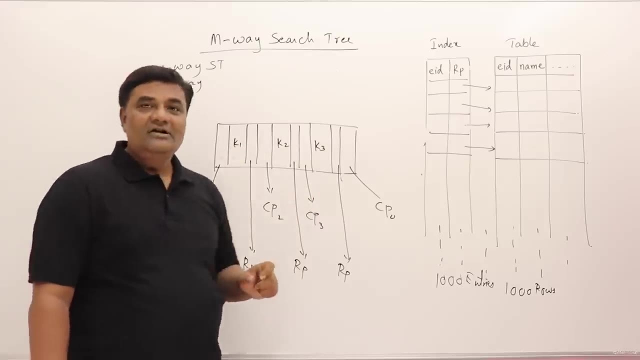 this. So If you want to know more about this node structure, see keys are there- and child pointer, so four. degree four, so four, child pointer. three keys, so three record pointers for each record. for each key there is a pointer to the record, to the database record. 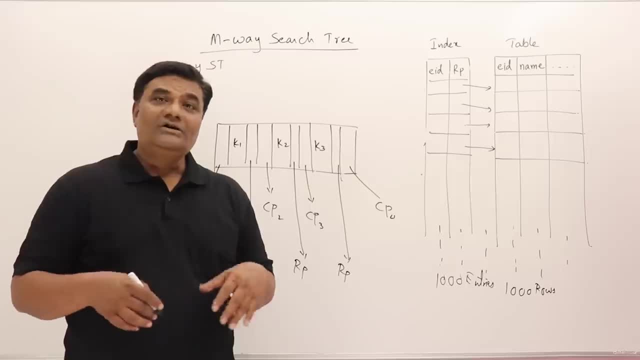 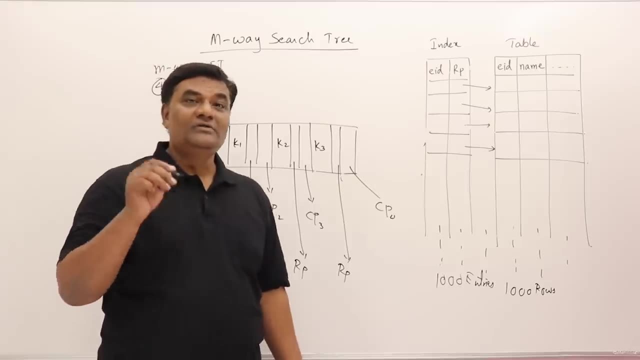 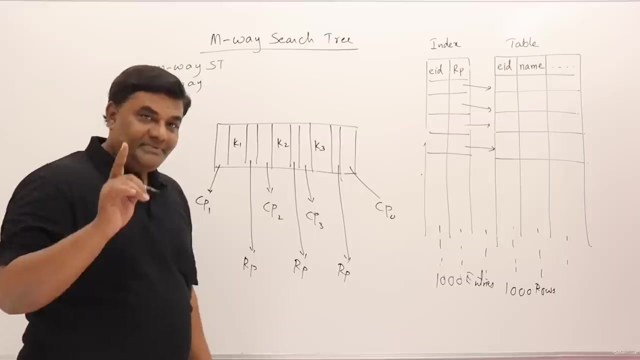 Now, if we simply use M-way search tree, what will be the problem and how we can overcome the problem and we introduce B-trees? now we are going towards B-trees. now, till here, we have discussed about M-way search tree. Now I am taking you to B-tree, and in B-tree we will use the same name: node structure. 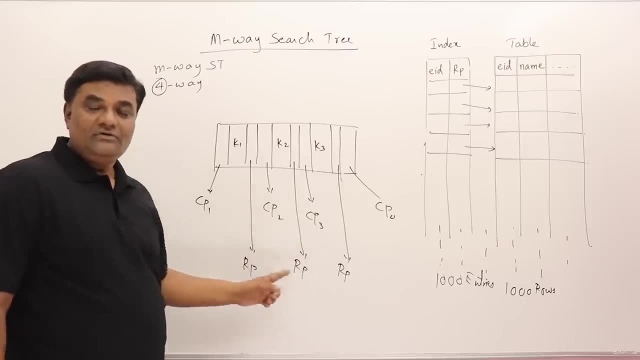 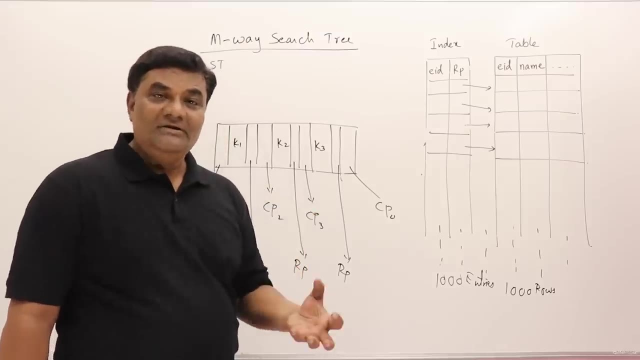 just remember this again. I may not be showing you this will be the node structure that is followed in B-trees, but first of all let us know what is the problem with M-way search tree, then how B-trees are different from M-way search trees. let us see how insertion is done. 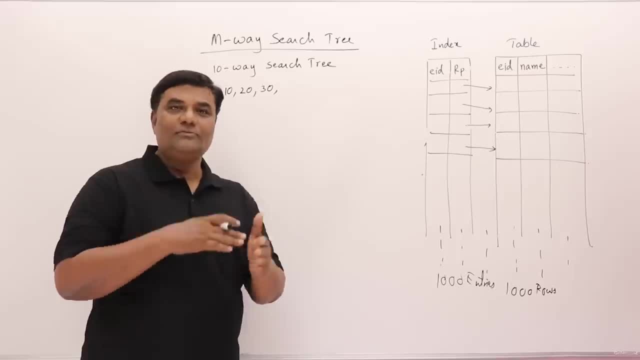 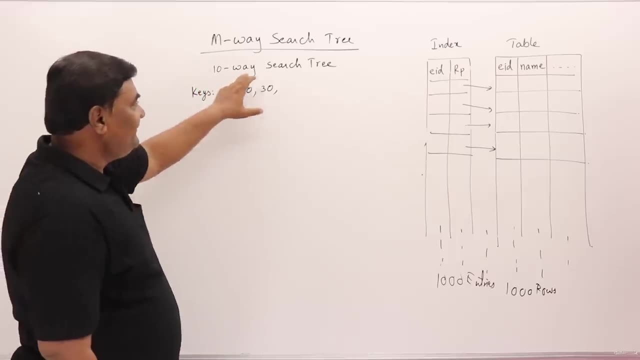 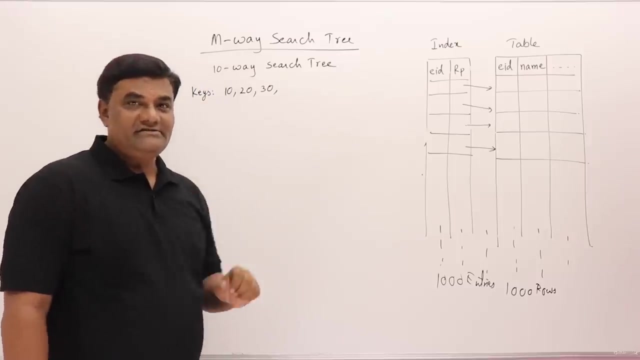 in M-way search tree and what is its problem. then we will move on to B-trees, for that we have discussed. To make you realize the problem, I have taken 10-way search tree. 10-way means degree, 10 means each node can have 10 children and the 9 keys and suppose I have to insert these. 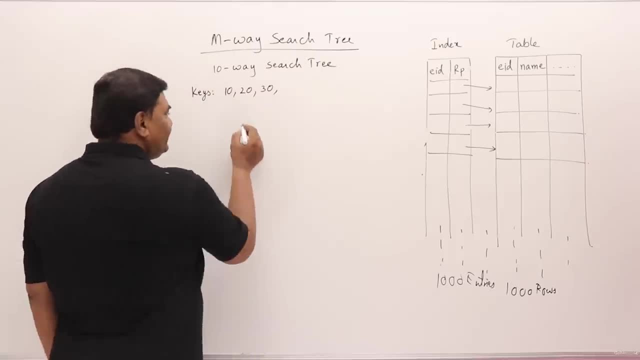 keys. let us see how I can insert first 10. there is nothing, so I will create a node and insert 10. how many more keys I can have here? 8 more keys I can have here, but for inserting 20 I will create a new node as a child and insert 20.. 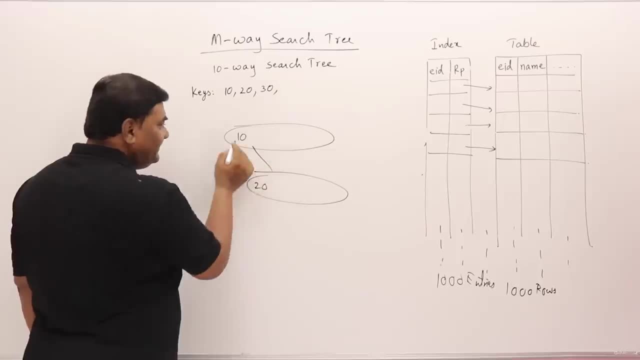 So I have taken 10-way search tree. 10-way means degree 10 means each node can have 10 children and insert 20, then inserting 30- 10 that is smaller, 30 comes on right side, so I will not insert here, but I will come to this- and 20- 30 is greater than this. so 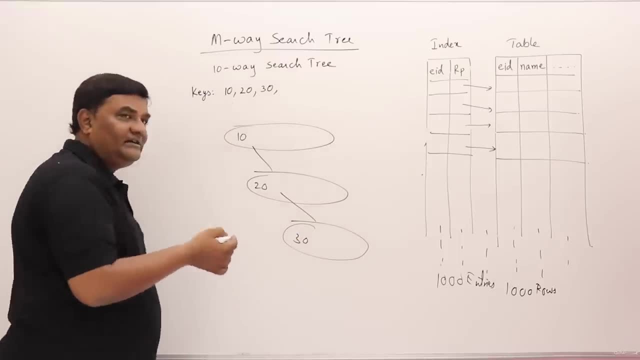 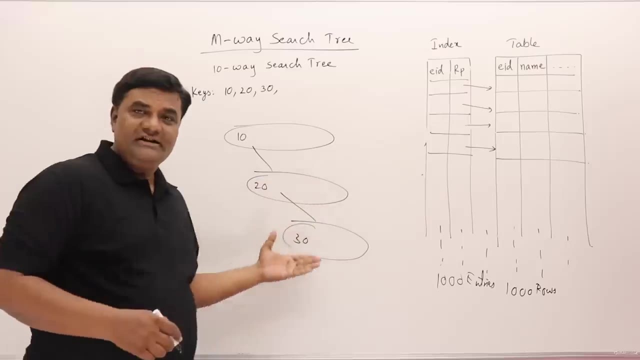 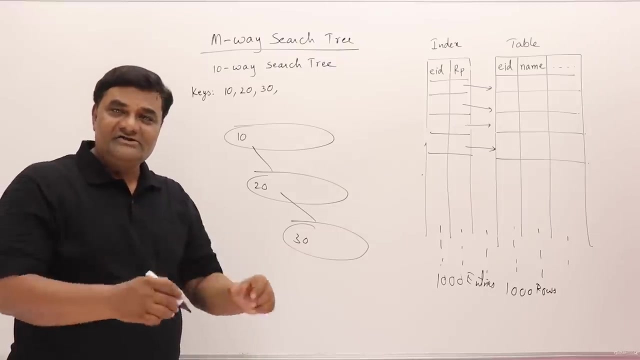 I will insert 30 here, So I can insert like this also. but this is wrong. I should first fill up this node, then only I should think of creating next node. but there is no control on M-way search tree. you can insert as you like. 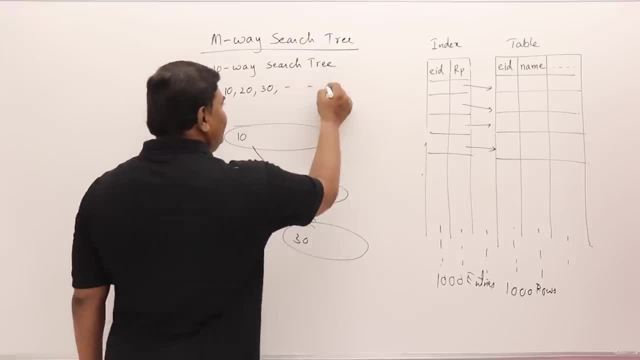 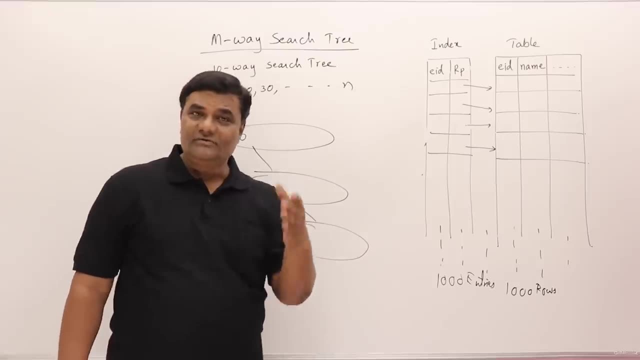 So it means, if I have N keys, then what will be the height of M-way search tree N, so this will be too much time consuming. it becomes similar to linear search. that's the problem with M-way search tree. so what is the problem with M-way search tree? the creation process. 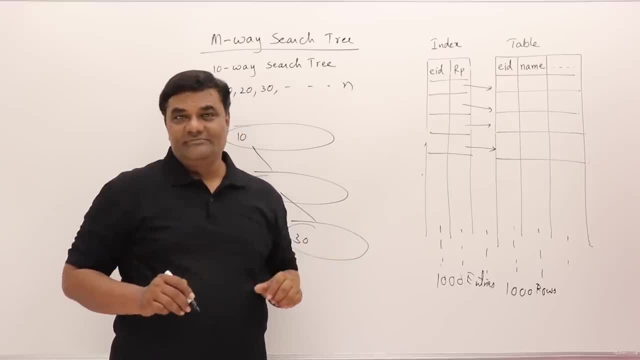 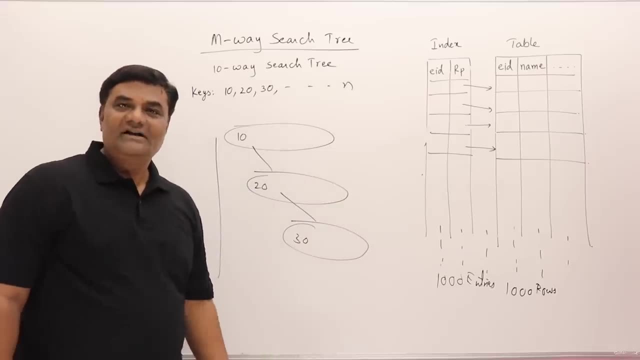 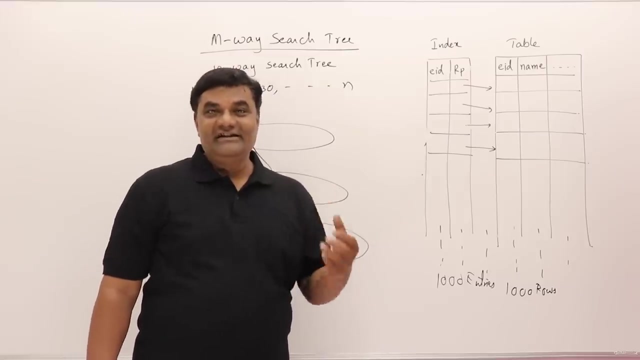 is not under any control. there are no guidelines for creation process. you can create as you like. if suppose you are creating it like this, then it's a waste of time. it will take lot of time for searching. then there must be some rules or guidelines for creating M-way search. 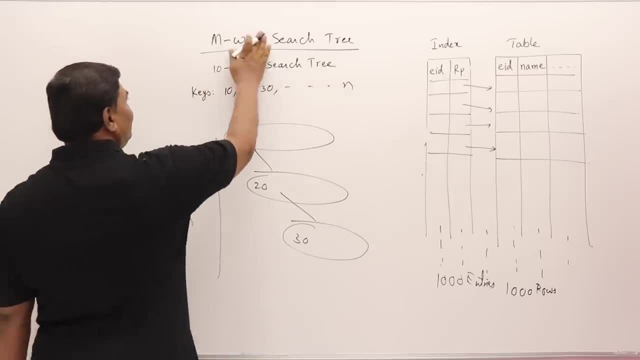 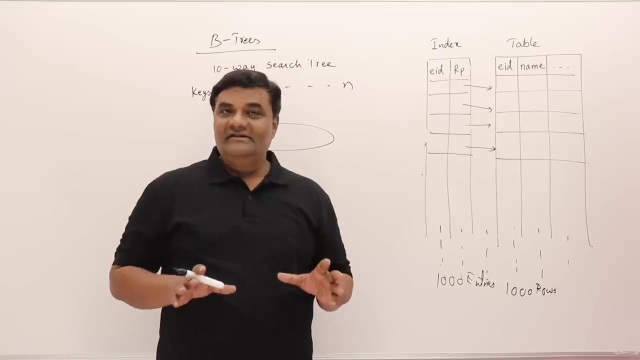 tree. yes, those guidelines are called as B-trees. so B-trees are nothing but M-way search trees with some rules. let us see what are those rules. I will explain them. let us see what are B-trees. B-trees are nothing but M-way search trees. 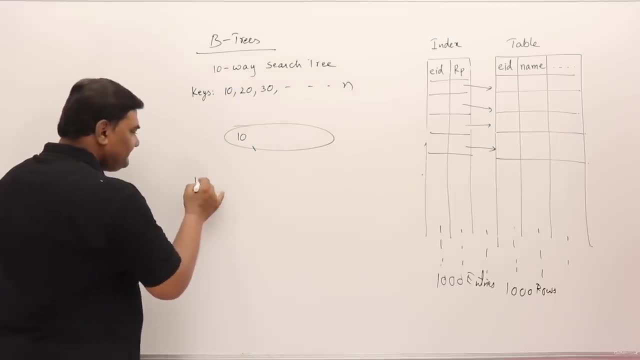 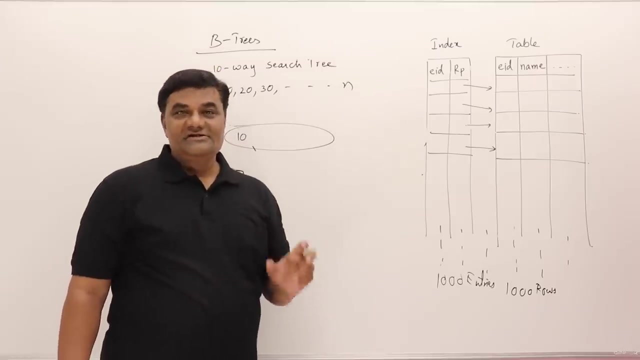 some rules. so what are the rules? let us see. see the first thing: every node you must fill at least half half. what if the degree is m? m by 2, children must be there. so m by 2, seal value is taken, not floor. m by 2 means if degree is a 10 means 5 children must be there for a node. every node. must have 5 children. then only you think of creating new node. that's what to control the height of m-way search tree. this is the rule. you can create a next node only if the current node is at least half filled with children. this is one m by 2. children must be there. 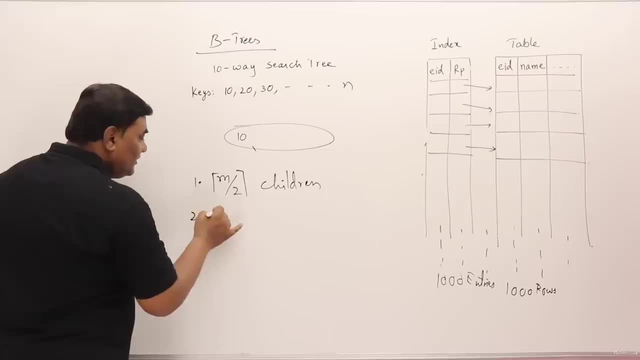 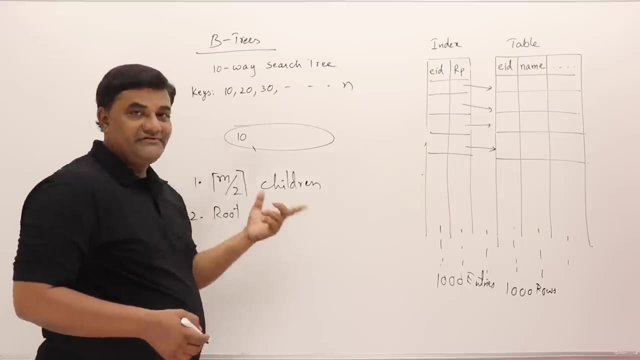 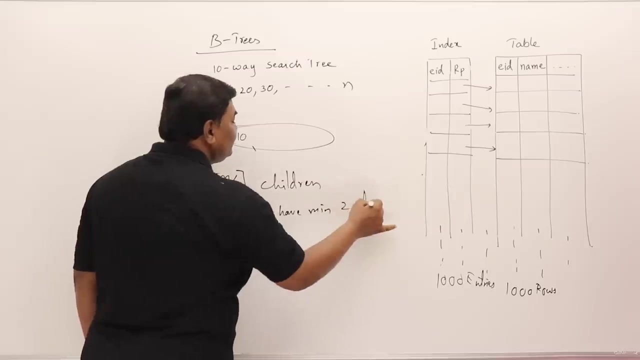 then second thing, how we can impose this condition on a root. we cannot impose this condition on a root. if we impose, then we cannot insert even a first value also. so root can have minimum two children, so root means the first one, so first node can have minimum. 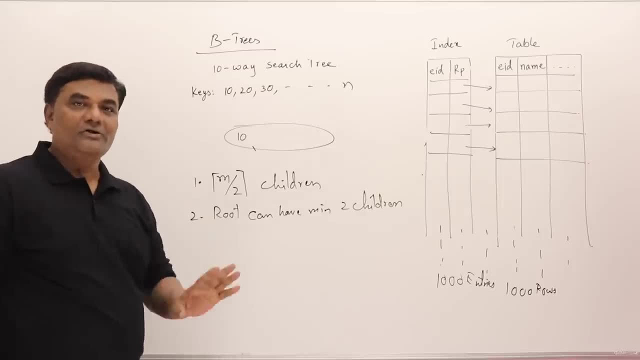 two children, right. so it means it can have just one key also, no problem. but what about all other nodes? they must have at least half of the children. this is the conditions. two conditions now, third conditions. then the third rule is: all leaf nodes must be at same level, all leaf at same level. that's it. these are the three things if you are following. 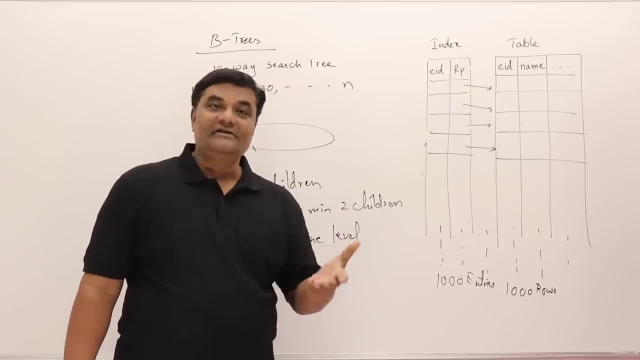 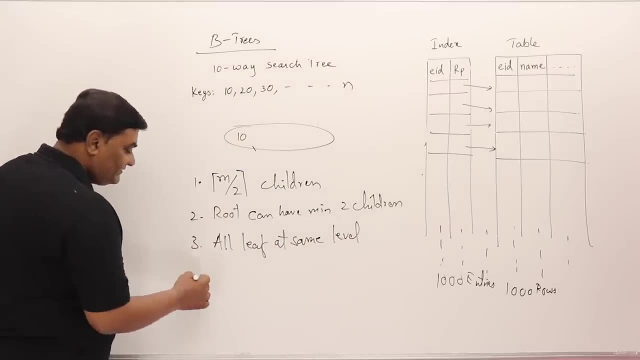 for creation of a m-way search tree. so actually we are creating b-tree. and one more important thing here is that the creation process is. fourth point is: the creation process is bottom up. creation process is bottom up. so now i will take some keys and i'll show you how a 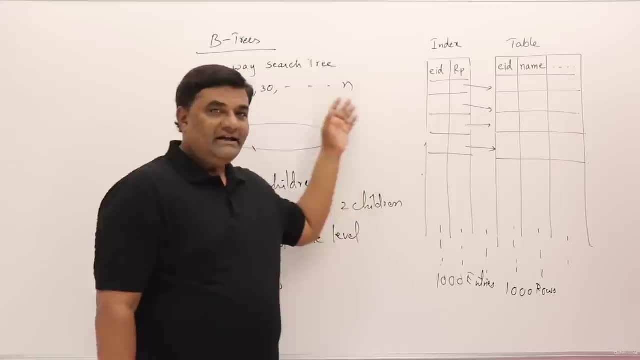 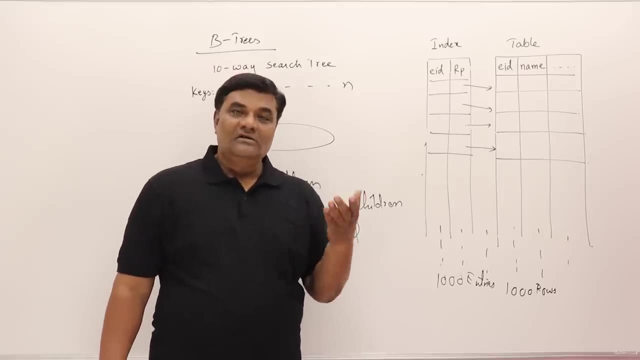 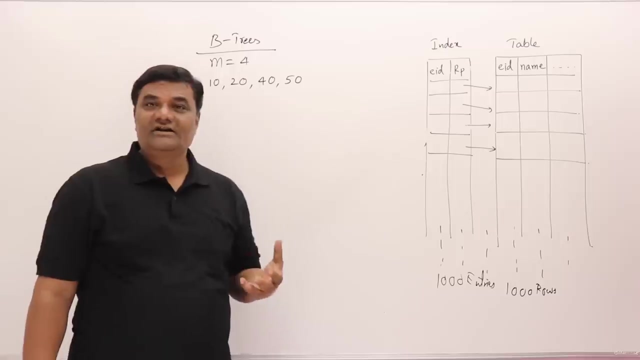 b-tree is generated from bottom up, so for that i will not take a charge. to take a small degree three and show you how a b-tree is created, in other words how insertion is done, we will create a b-tree of degree four means each node can have four children and three keys. so i have taken some. 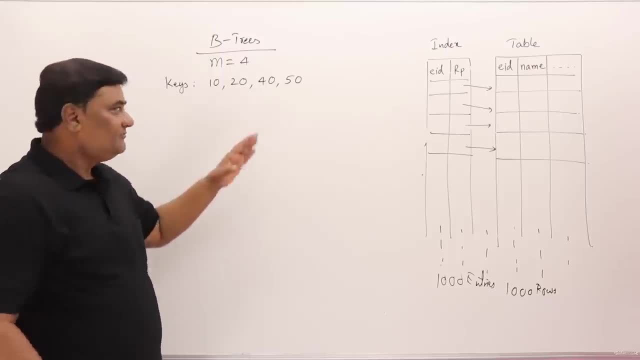 the keys here, then i will be inserting more and more nodes, so i will add more keys afterwards. let us start first. there is no node at all. first key i am inserting. so that is 10 first key. so it can have how many children? two children and as per the multi-level index. when we said, 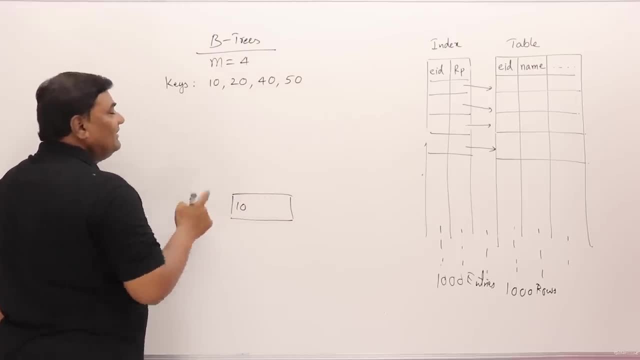 then it can have one record pointer. the next 20: 20 will be inserted here that is greater than 10. 40 is inserted here. next is 50. there is no space for 50. already three keys are there. degree is four, so we cannot insert 50. 50 there is no space. then what we should do? split this node and create one. 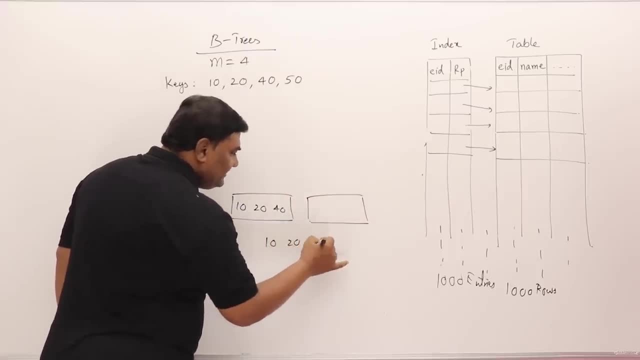 more node. so out of 10, 20, 40 and 50, two keys- i will keep this side and one key i will send this side. 40- i will send it in the root. 40- i will send it in the root. 40, i will send it in the root. 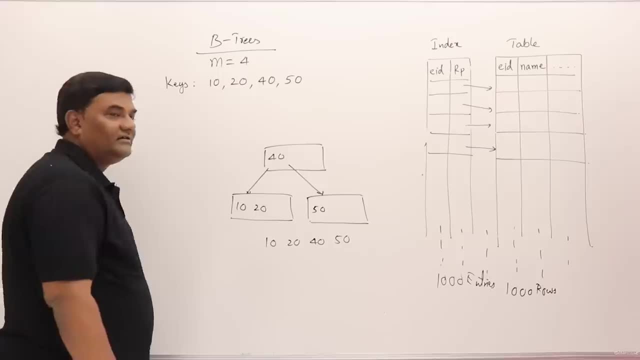 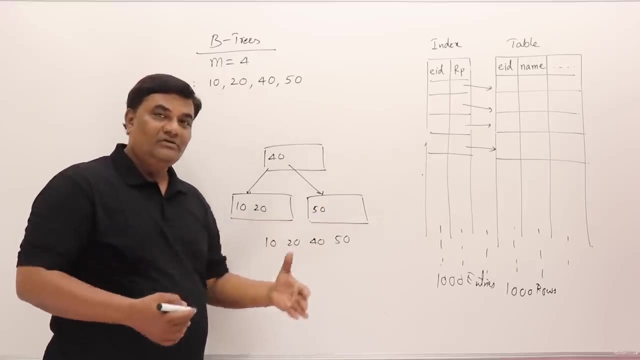 then this is the left child, this is the right child, that's it. so when the node was filled, there was no free space. then for inserting a key. we have splitted a node and one of the key, we have sent it on the route out of four, including 50 out of. 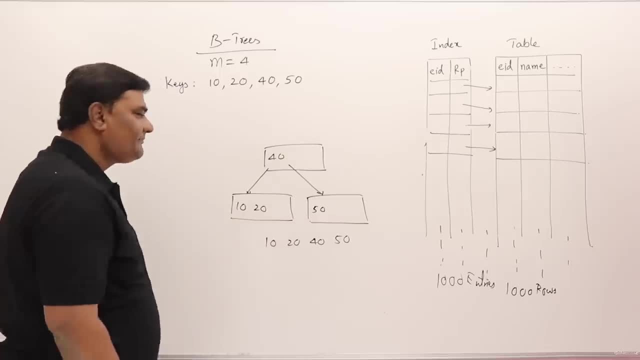 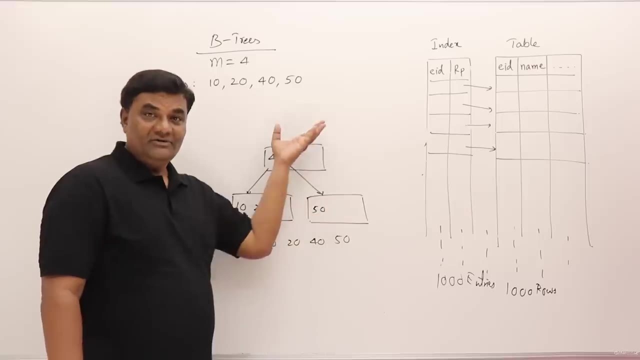 four: two this side, one that side, 40 up. this is how splitting is done, while creating a b tree, and you can see that the tree is growing upwards. so that's it. it's created bottom up, and i was telling you that this is b. trees are useful for implementing multi-level indexing. 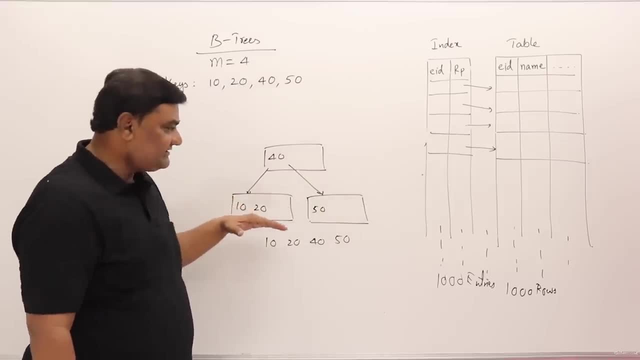 then if you say this is one first level index, then above that this is the second level index created automatically. if you add keys here, automatically this is created. now, let us see i will add more keys here. then again you can see that this is growing. so let us continue. i will insert few. 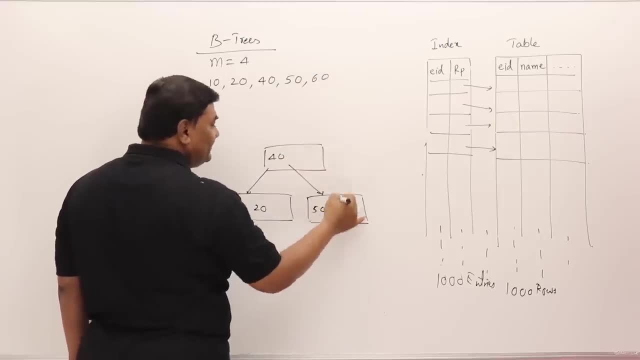 more keys. let us say 60, so 60 comes here, then 70, and then i will add more keys here, and then i will say 80, and it is still here, and then it is still here, and then i will say 60, then 80 comes here, then 80, 80. there is no space. 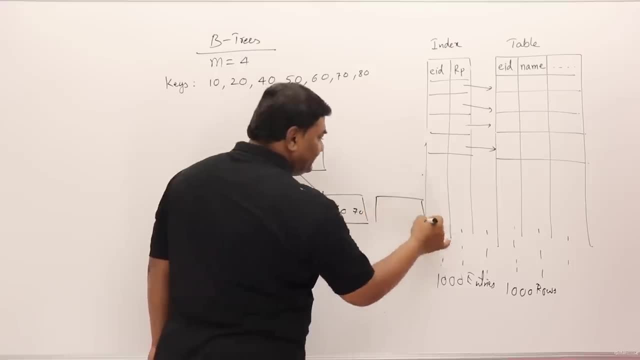 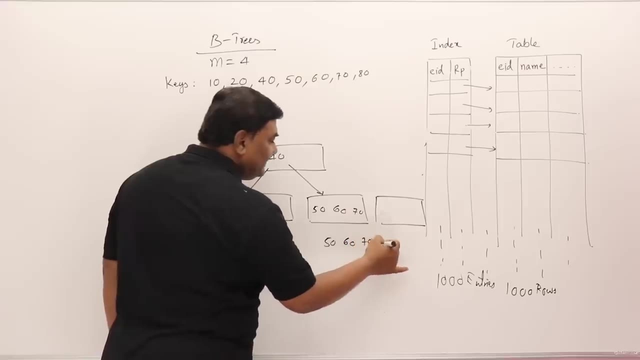 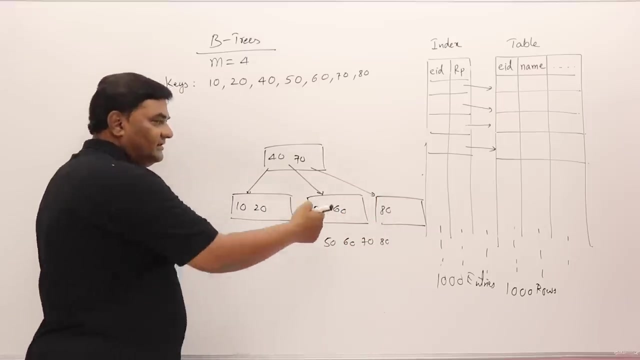 here. 80 should come here. there is no space then split again then what i should do, including 80, 50, 60, 70 and 80. so 80 should go this side and 70 should be in the root. that's the child. now the tree looks like this then. 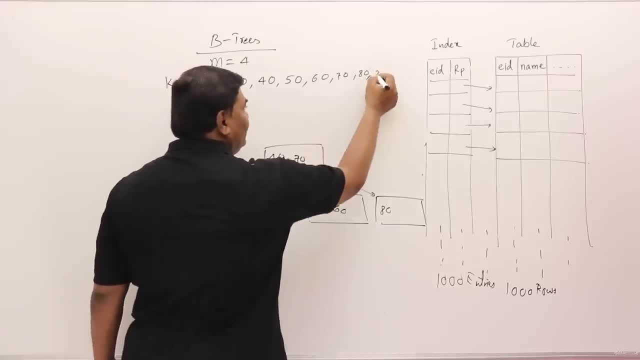 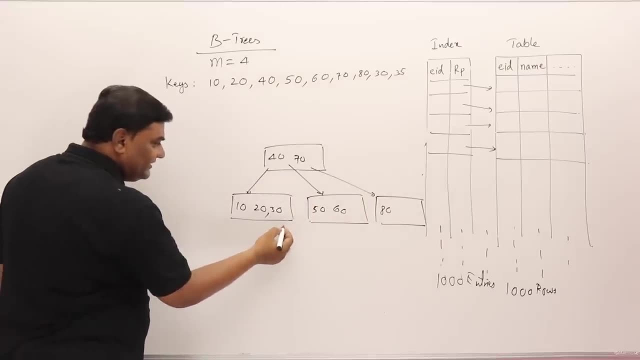 next i will insert insert 30,. 30 will come here. Then I will insert 35, there is no space for 35 here, Then split. so as there is no space, I will split this side. So out of 10,, 20,, 30 and. 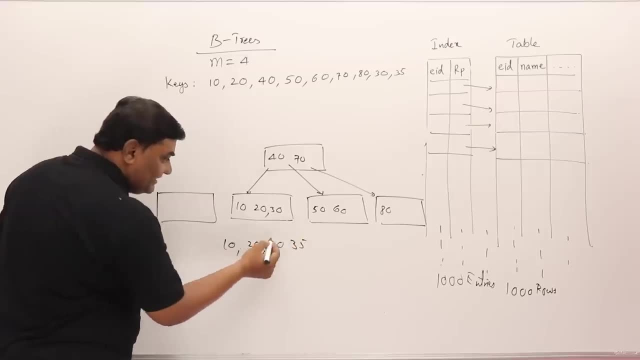 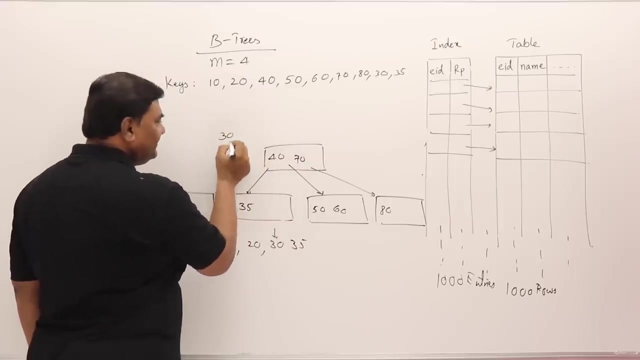 35, 35, this should go in the root- and 10, 20 this side and 35 on this side, right side side, 35 on this side. Then who will go in the root? 30. So I will redraw it. 30, 40. 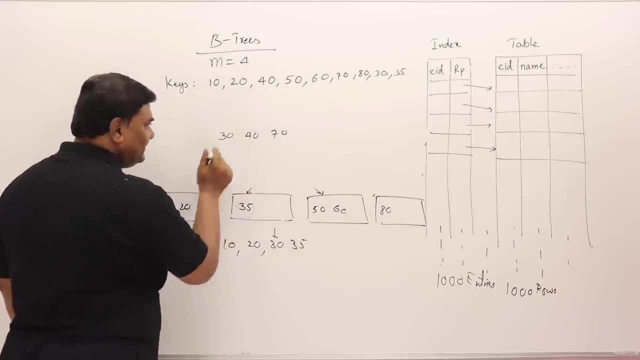 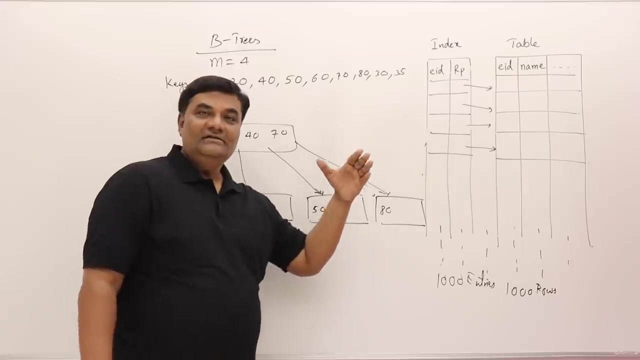 and 70. I will remove this. Yeah, watch here, This is the child, this is the next child, this is the child and this is the child. This is how the tree looks like now. See, whenever the node is becoming filled, we are splitting it and we are sending one of the key in the 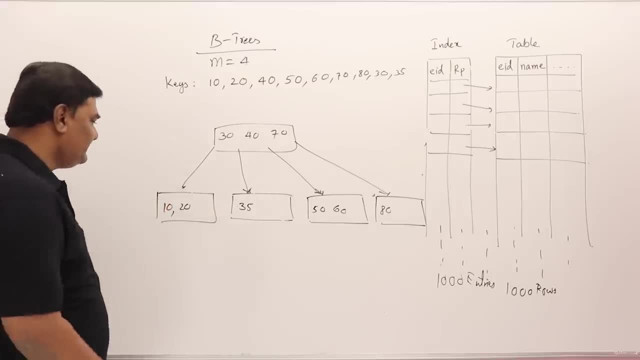 parent. I will try to fill few more keys here and let us see. I want to insert 5.. So where 5 will come, 5 will come in the beginning. So 5,, 10 and 20.. Now I want to insert 15.. 15. 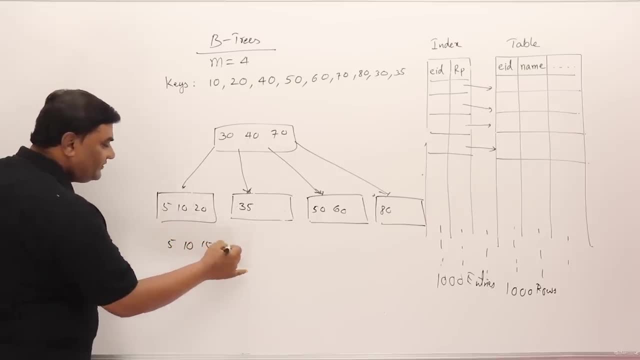 there is no space, So 5,, 10,, 15 and 20, there is no space for 15.. Then arrange them in this order. Then there is no space when split it, So for splitting I will create one more node. 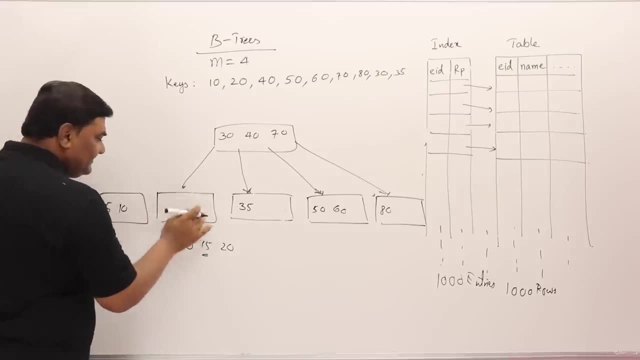 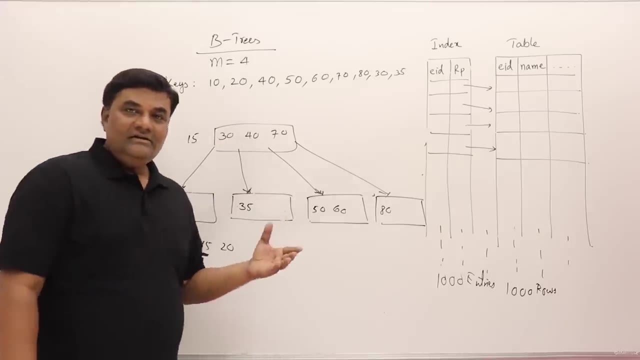 on this side, 5 and 10 this side and 20 this side. Now, 15 should go up here. This should go up. Alright, this should go up. OK, one more point. You would have been thinking why I am sending third key. I want to send second key, Okay. 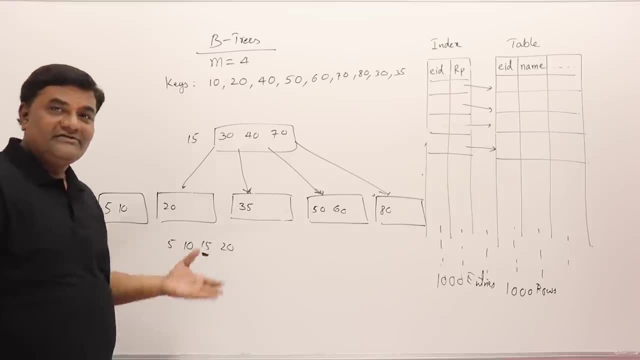 that is your choice, So you can make either less biased or right biased. Either way, you can do that. Now it is left. biased means it is more keys are on the left side, So whichever one you want, you can take it. 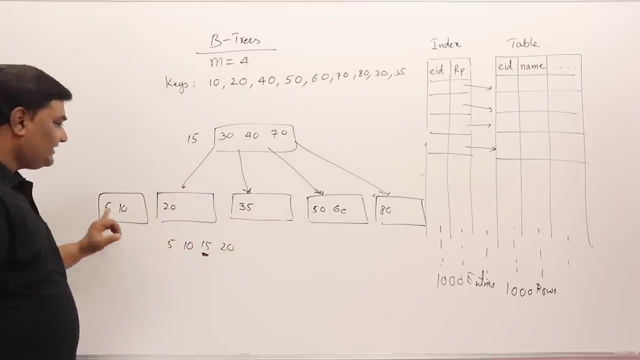 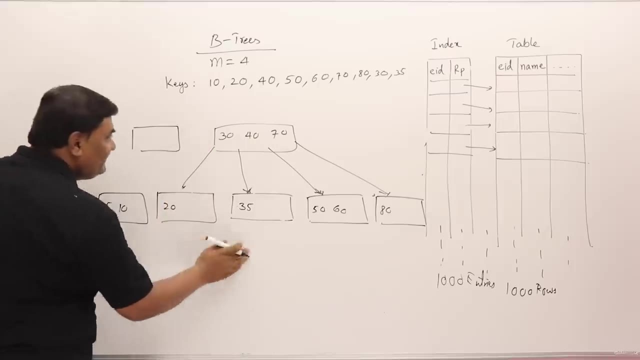 So 15 moves up, 20 moves up on this side, 15 moves up on this side and 5 and 10 this side. now there is no space here also, so here also you split it. so out of how many keys? 15, 30, 40 and 70. so 15 and 30 this side, 70 that side and 40 in the parent. so this will be. 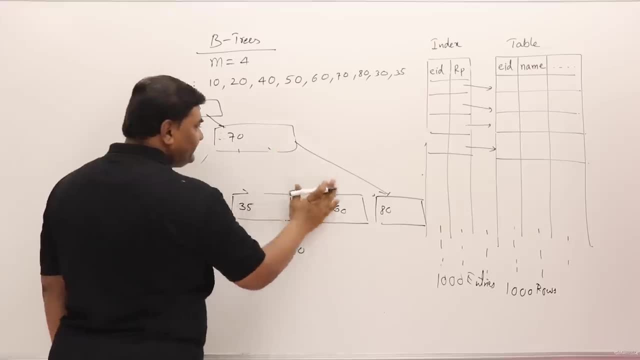 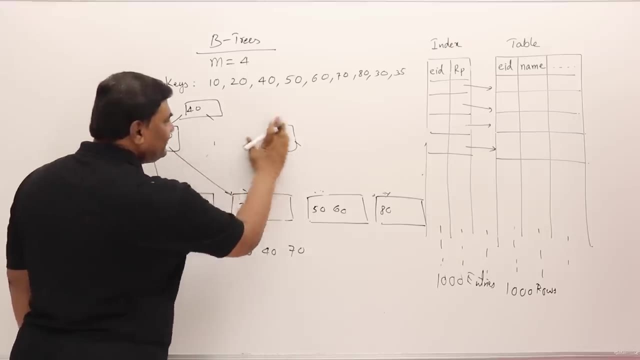 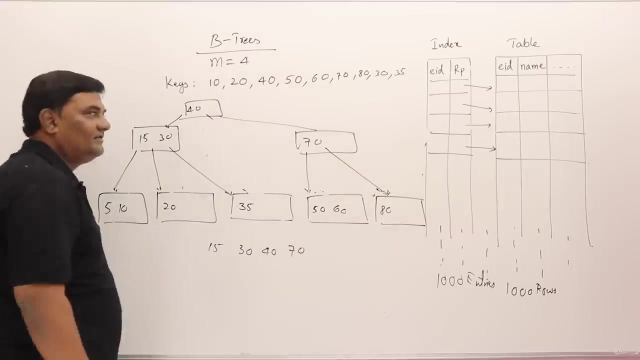 on this side. this will be on this side. now all these links will also change, because we are splitting it. so this is on this side. this is on this side, this one- and i will draw it little far from this one- 70, then 70 is left and 70 is right. so now you can see there are three. 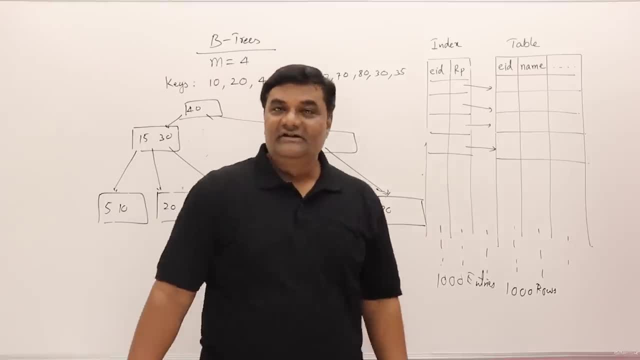 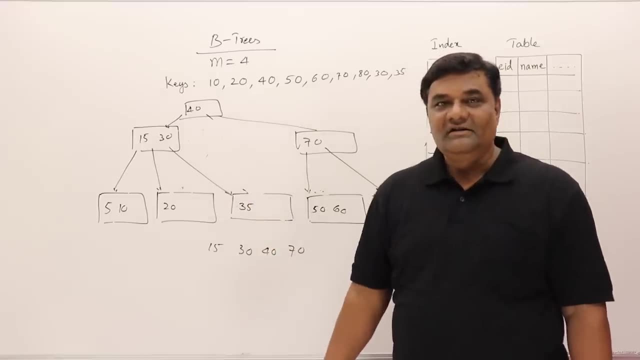 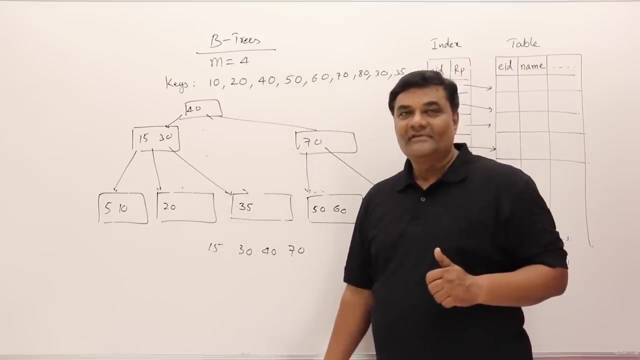 levels one, two, three, so three levels of indices are created and this is how b tree is generated: by inserting keys, and the height of a b tree is increasing and this is same as a multi-level index. so this is the creation process, so it's under control and all leaf nodes are at same. 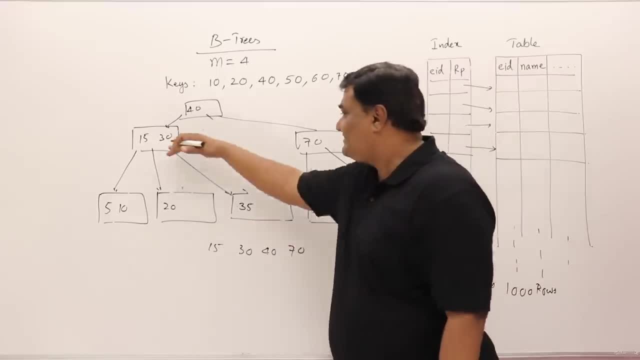 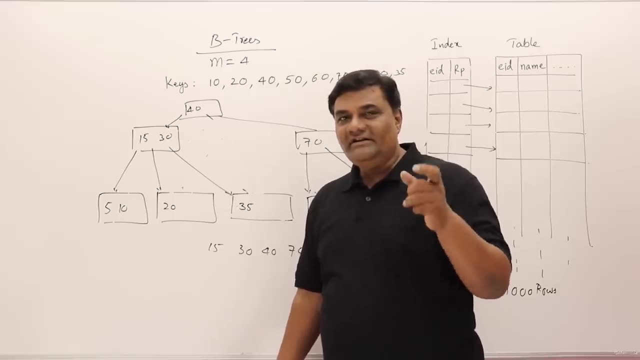 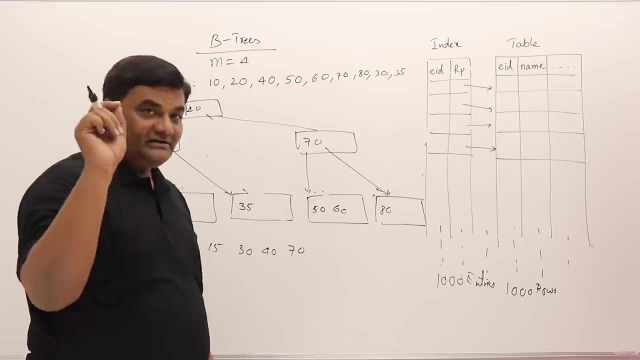 level, so they are looking like more like a index and this at same level. this is forming index and above one is also an index. so i have shown you how to insert and how to create a b tree. now let us see how it is useful for the databases. just minor things are very important and key. 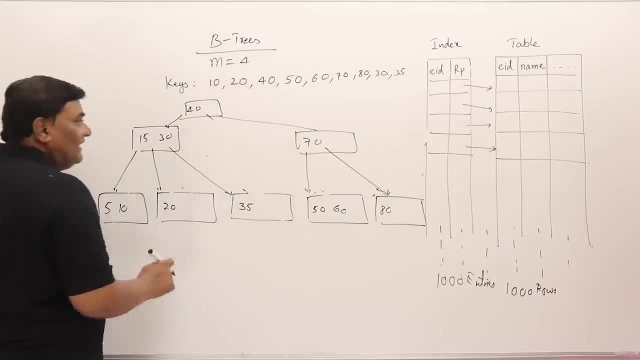 points. i am showing you, as we discussed just now, that every node will have a pointer to the child node as well as a record pointer. this 20 will have a record pointer. 5 will have a record pointer. 10 will have a pointer. 15 will have a record pointer. 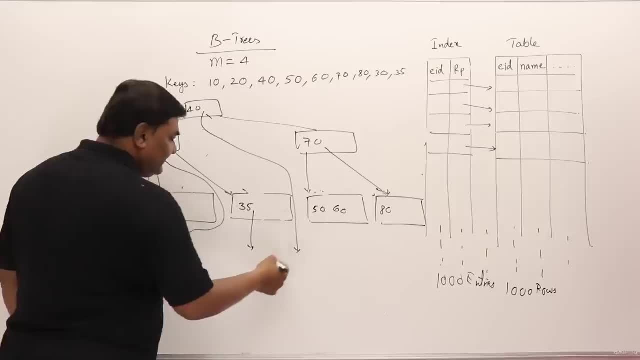 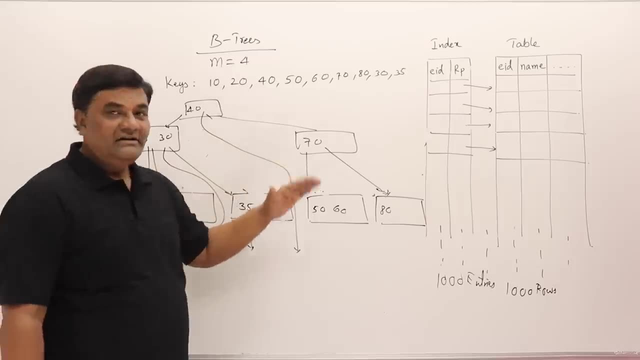 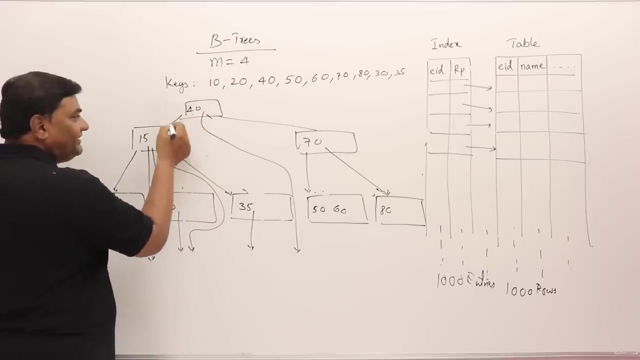 every key will have a record pointer also that is pointing on the database. so this is useful for implementing multi-level index. Apart from the child pointer, this is a record pointer. so a ba tree can We can have what child pointer. that is a block pointer and this is a record pointer. that's it. that's it about b trees. 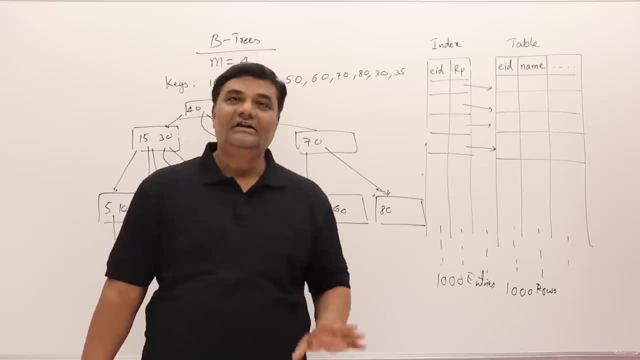 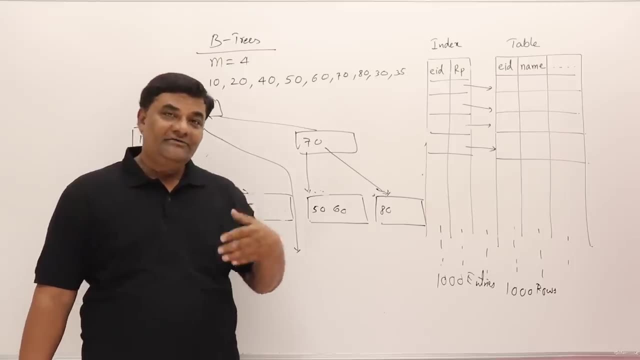 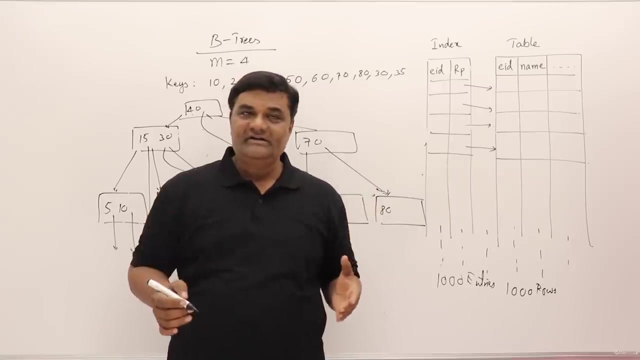 i did not show deletion. it depends how much you have understood from this one. just you reply me back. leave your comment and, if required, i'll prepare deletion also. okay, actually i wanted to show you what is the application of b trees and b plus trees, so i have started my topic, right. 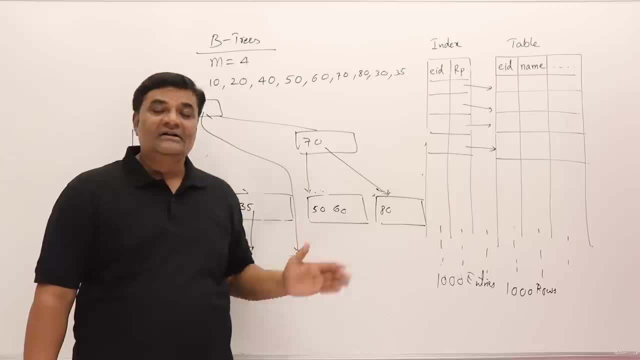 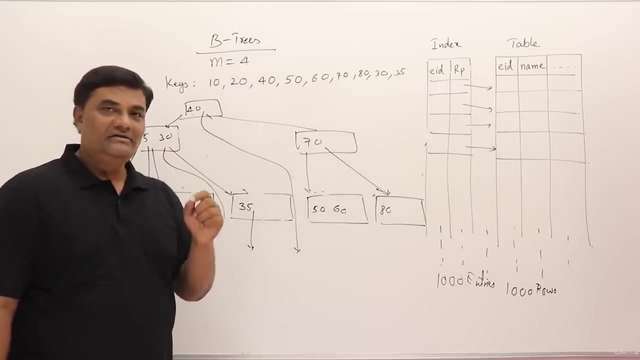 from indexing and brought you up to this point so that you can understand the relation with the databases and b trees. otherwise, mostly people study just about b trees and b plus trees without knowing indexing and databases. so now you can relate it with the databases. now the last thing. 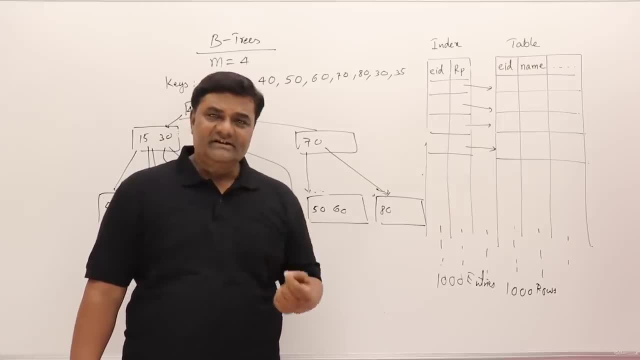 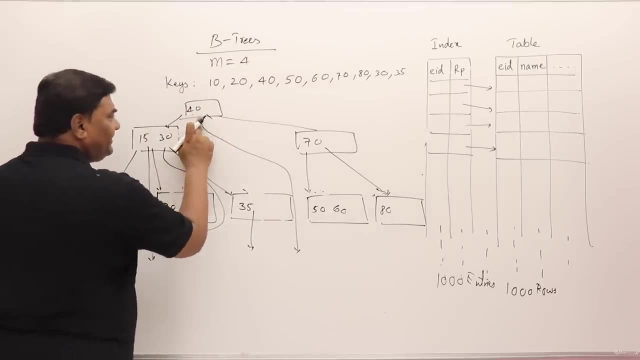 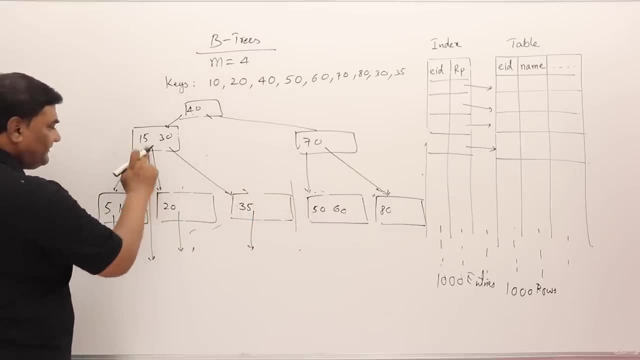 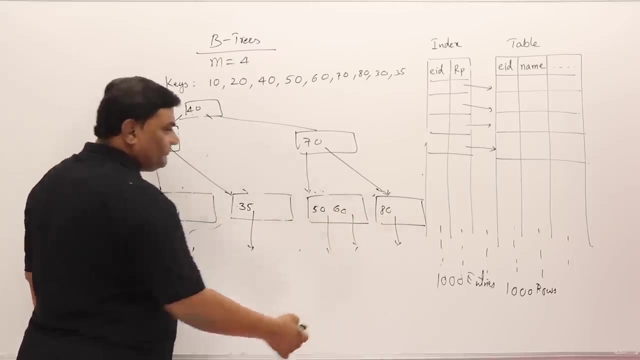 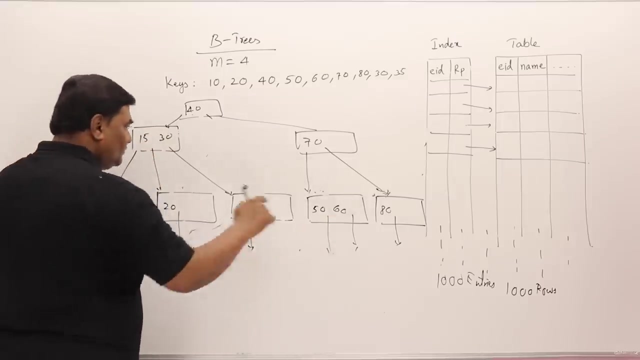 pointer from every node. we will not have a record pointer from every node. we will have record pointers only from leaf nodes. only from leaf nodes will have a record pointers. then what about these keys? every key will have its copy in the leaf node. so means, who is missing here? 15 is missing here. 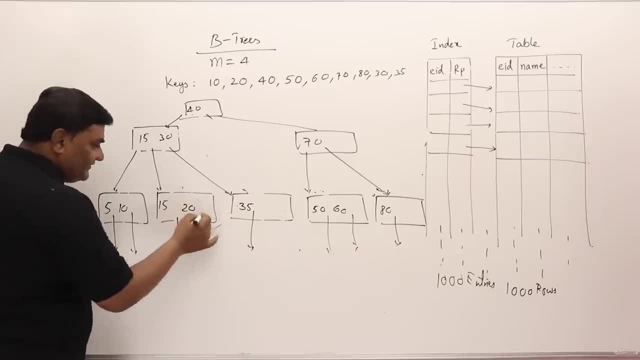 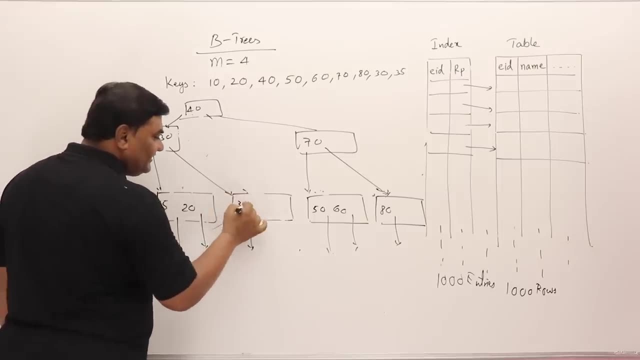 so 15 will be here also 20. so 15 will have its copy here also. so there will be record pointer for 15 also, 20 also, then 30 here will have a copy of 30 also and 35. so what about what about 40? 40, we will have a copy here also. 40. 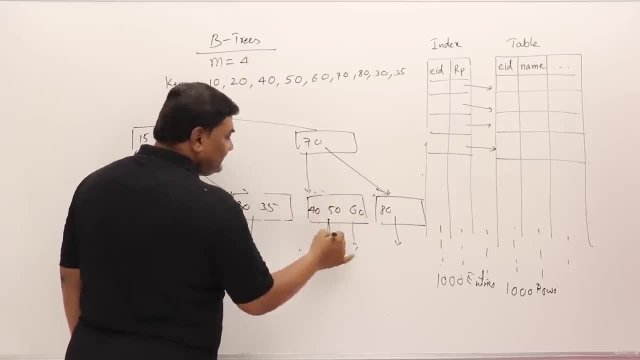 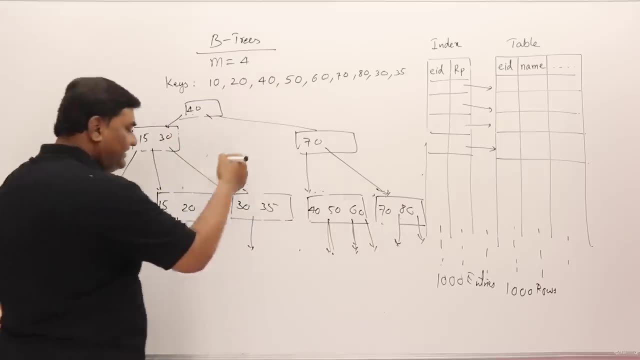 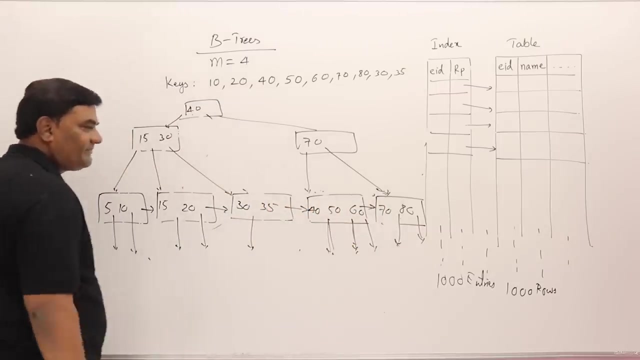 will be having a copy here. so 40 and 50 and 60, so three record pointers, so 70 will also be present in this one. so every key in the tree will definitely present in the leaf and this leaf nodes are connected like this, like a link list, so this becomes a dense index. now this is exactly. 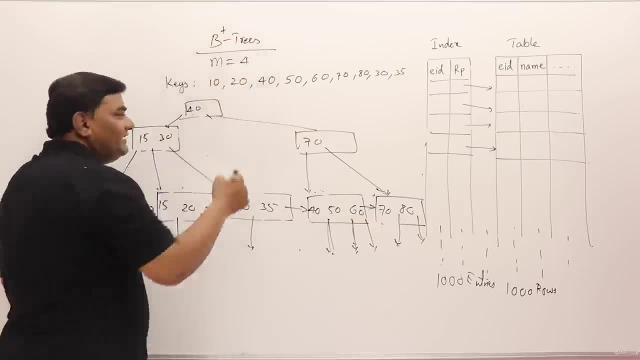 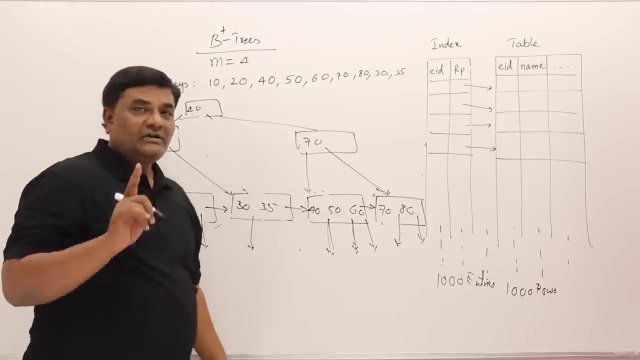 like multi-level indexing. so this is b plus tree. so what are the differences from b tree to b plus tree? let me quickly tell you that all the keys are present in the leaf nodes and in non-leaf nodes their duplicates may be present. every key must be present in leaf and there are no record pointer. 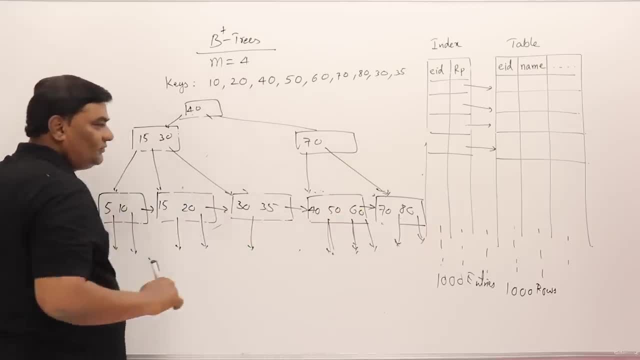 from non-leaf nodes, the record pointer will be from only leaf nodes. so leaf nodes, all leaf nodes, as they are at same level, they will form a link list. these are the points. then this becomes a dense index. this becomes a dense index, then this is a sparse index. next, 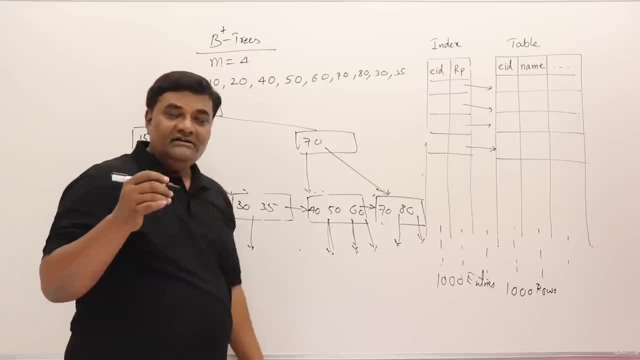 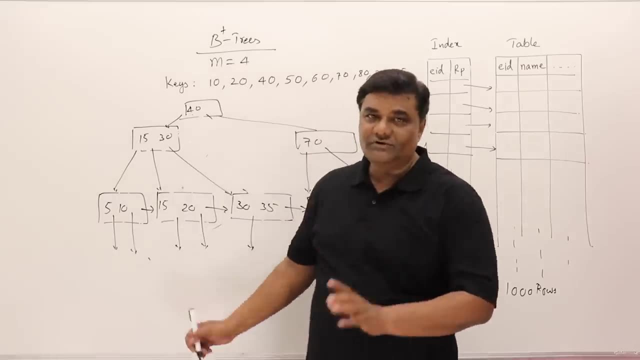 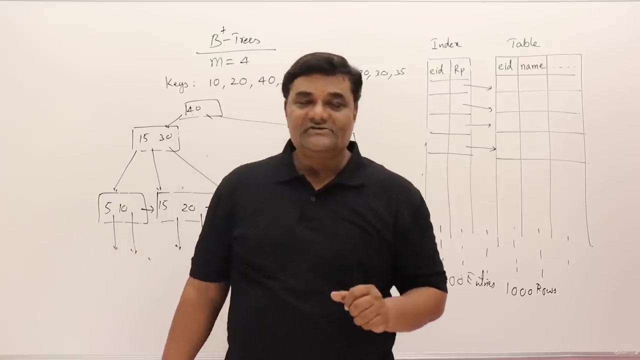 level. the next level is sparse index. so rather than b tree, b plus tree is more like multi-level index. so what is plus in this one that i have shown you? so if you understand b tree, understanding b plus tree is not difficult. that's all with this topic. there are analysis and a lot of things are. 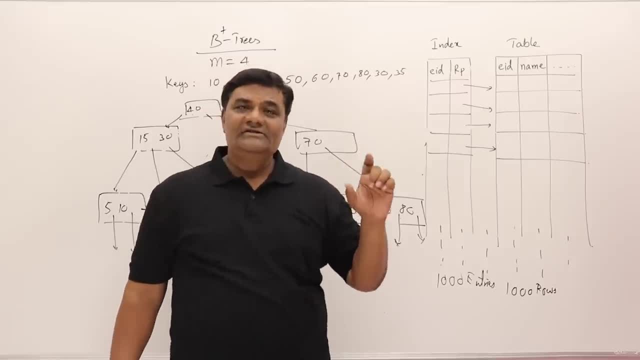 there, so it's a big topic. the purpose of coverage of this topic was to relate it with the databases. all right, so i have covered more from the database side than just b trees and b plus trees, so just b plus b b trees and b plus trees can also be taken. 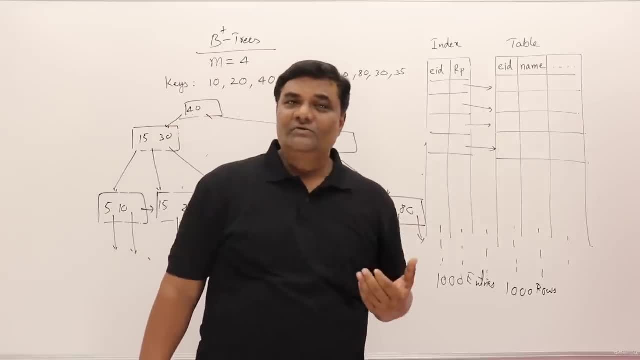 as a topic and discuss. leave your comments, let me know. if required, i will prepare a separate video.